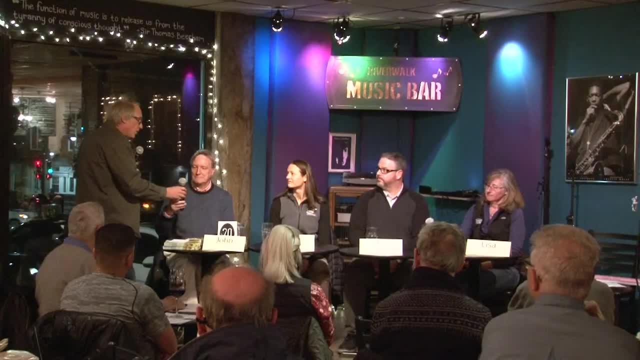 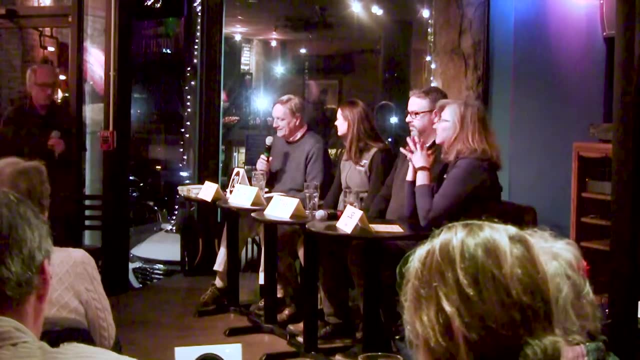 So this is a great panel. We're very proud to have them here. Maybe introduce yourself in a little more depth and then we'll start taking questions. John Aber, UNH, 32 years. Um, as the intro said, I survived eight years in administration to return to real life as a faculty member. 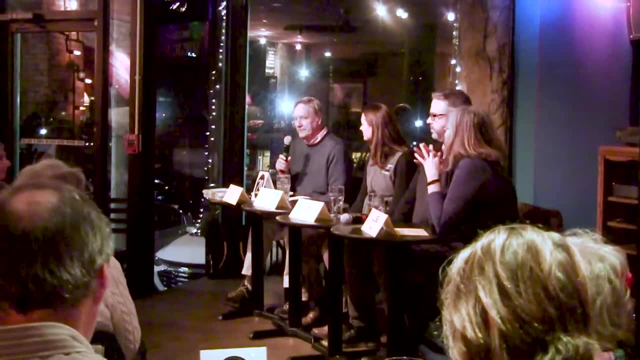 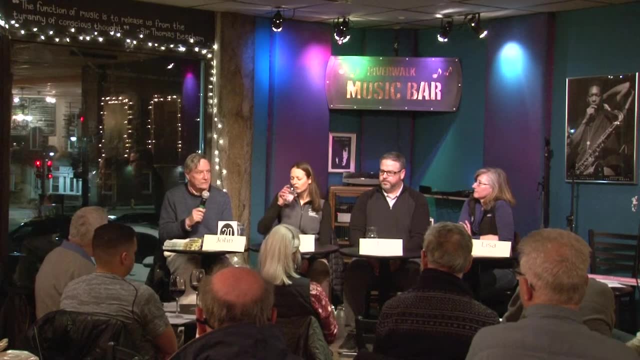 With a break in there that actually allowed me to apply for a grant to do research at at the first in the nation, I'm sure, organic dairy research farm at the University of New Hampshire, And actually still the only one in the country. 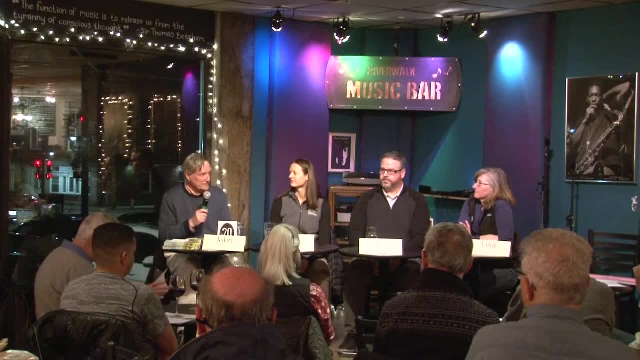 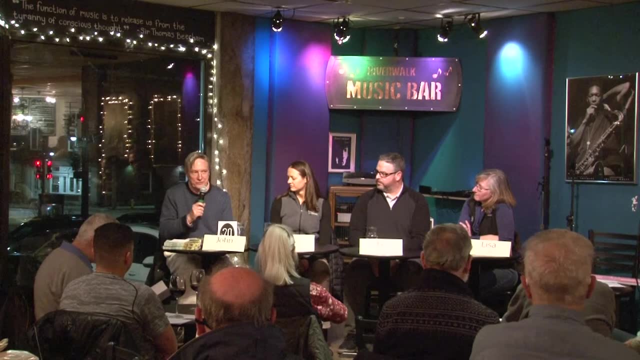 which is a story in itself. Many thanks to Stonyfield for their early support and guidance in the development of that farm. One of the projects that we pursued as part of a ecosystem approach to try to close nutrient cycles and energy cycles was an innovative approach to composting. 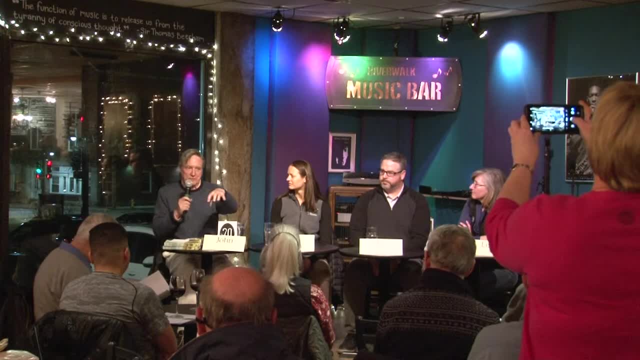 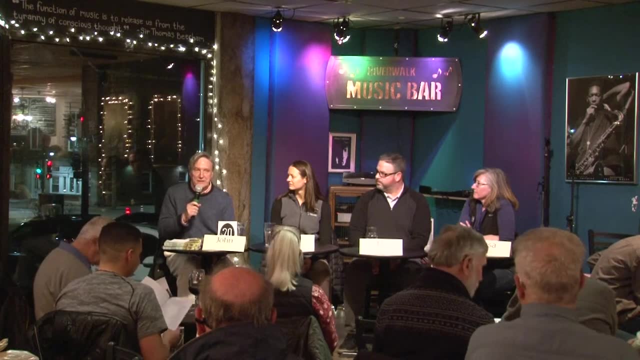 So you think of compost piles as those turnable long windrows. you know the things in your backyard. Compost is going beyond that In the last 10 years. there's a process called aerated static pile composting with heat recovery. 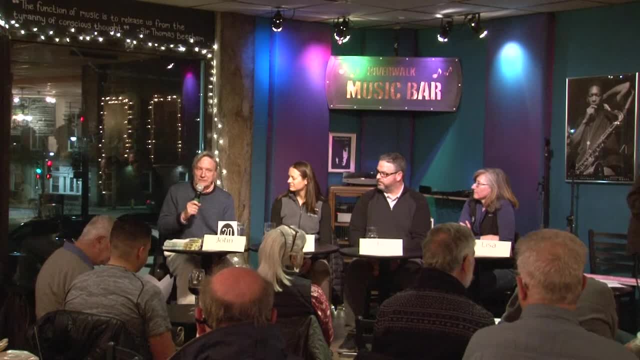 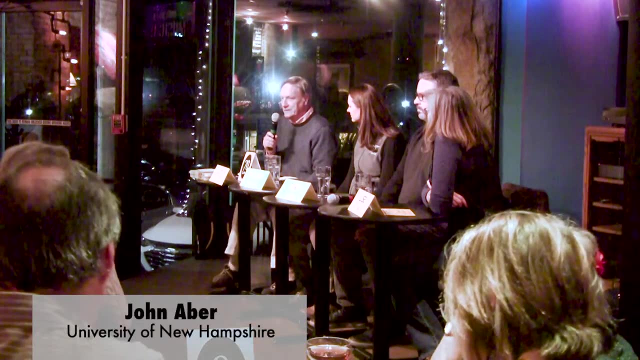 And the facility we have out at the organic dairy actually generates vapor air at 150 degrees and we can get about a million BTUs a day out of this facility composting farm waste. So part of a larger effort at UNH maybe we get a chance to talk about. 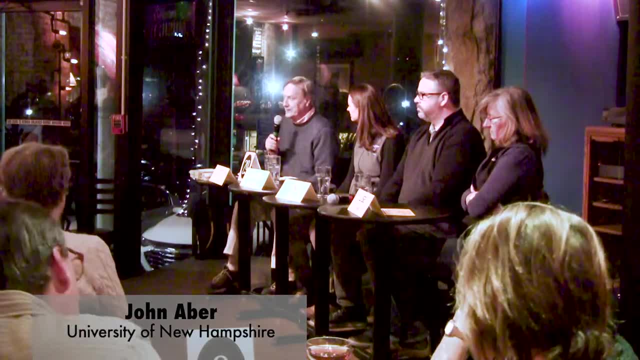 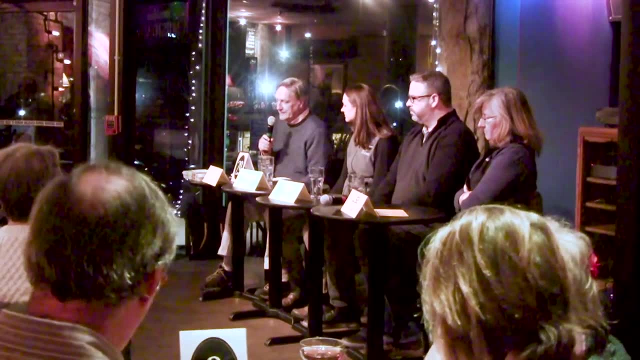 well, UNH is very proud of its role in sustainability nationwide. We get about 70% of our energy from landfill gas from Turnkey Landfill in Rochester. And to top it all, I guess the top one is that we are one of three universities. 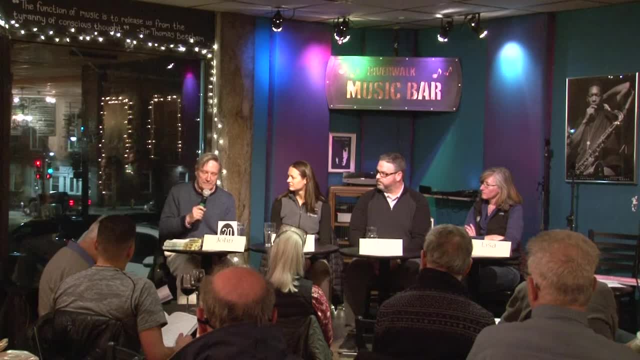 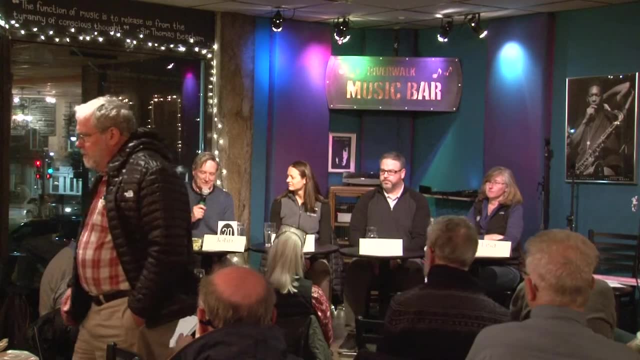 that have platinum status under the STARS program by the professional association that rates universities. So anyway, I'm looking forward to the discussion here. Hope I can add to it. So thanks for coming out. My name is Ragen Bissonet. 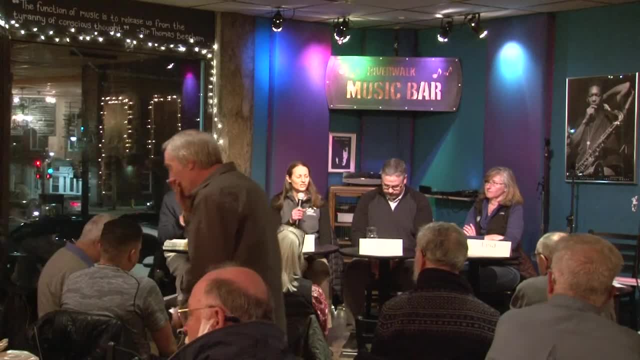 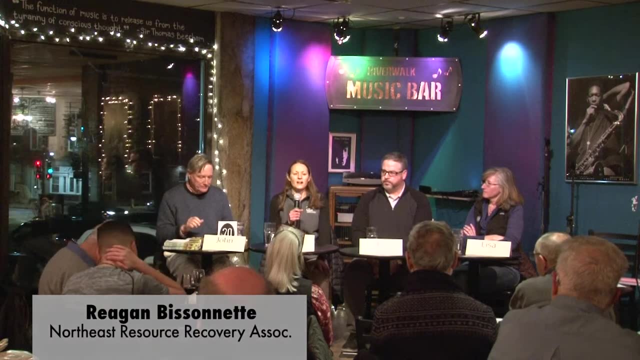 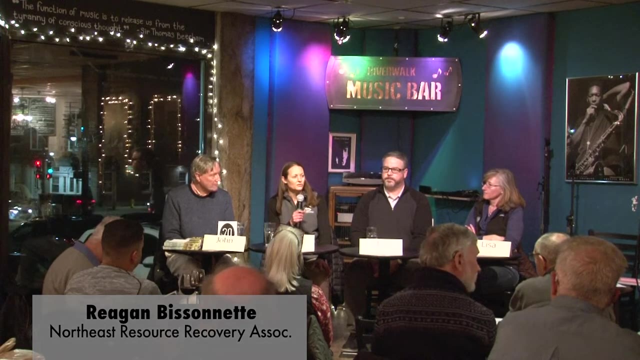 I'm the executive director of the Northeast Resource Recovery Association And we are a nonprofit that enables communities to manage their own recycling programs, And what that means is that we actually help communities sell their recyclables by connecting them to the companies that actually wanna purchase. 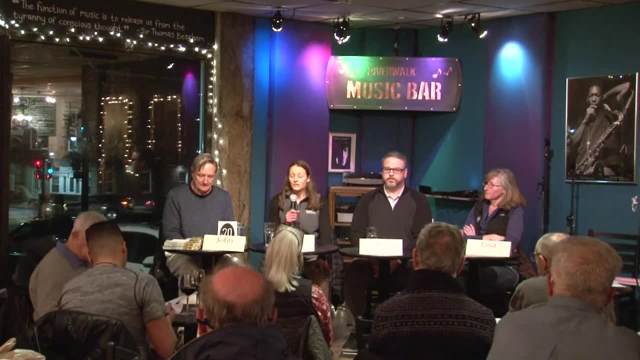 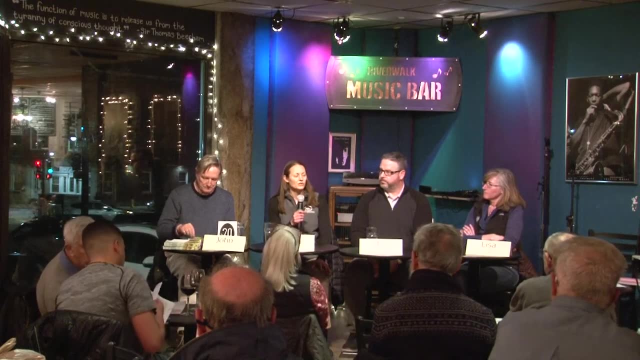 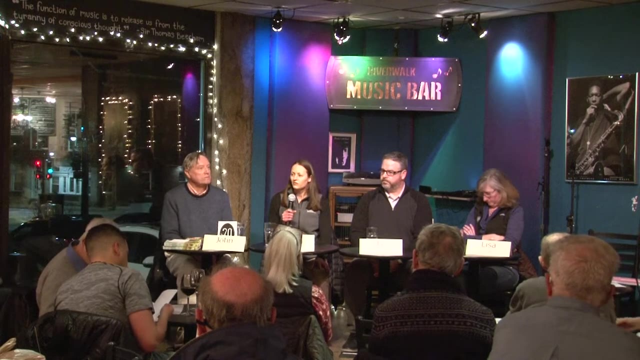 those recyclable materials, And the City of Nashua is a member of ours. We were actually founded jakiś years ago, About 40 years ago, when four municipalities in New Hampshire decided to pool together their resources so that they could get better pricing at market for selling their recyclables with their greater volume. 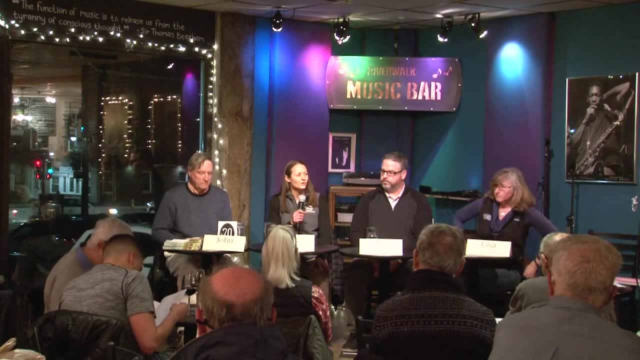 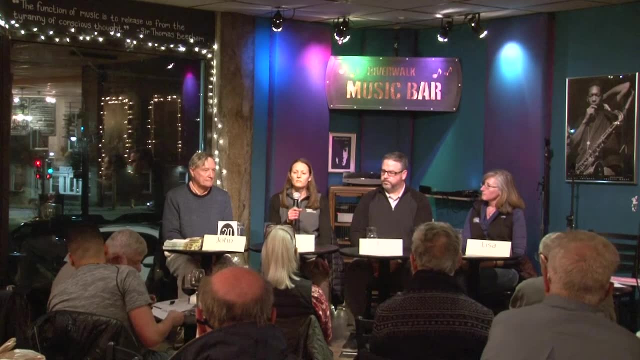 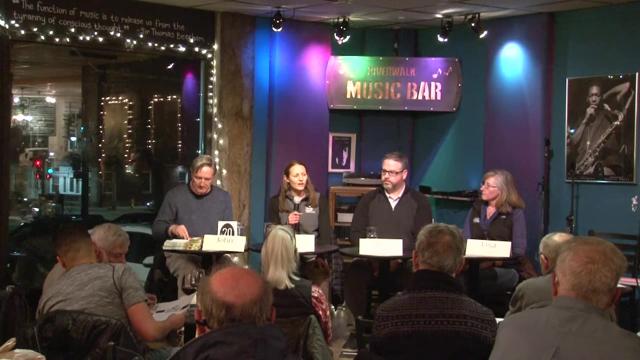 and so they could also share information about how to improve their recycling programs, And that really informs what we do today. We have over 400 members throughout New England. Most of those are municipalities, but we also have some businesses and individuals, schools, nonprofits and governmental agencies that are members of ours. 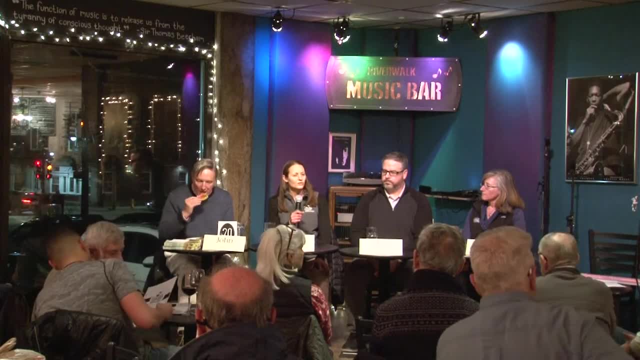 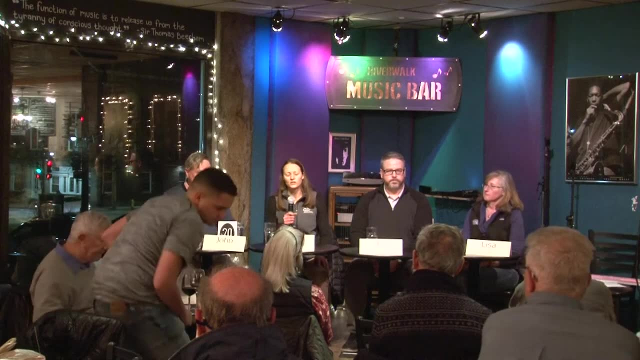 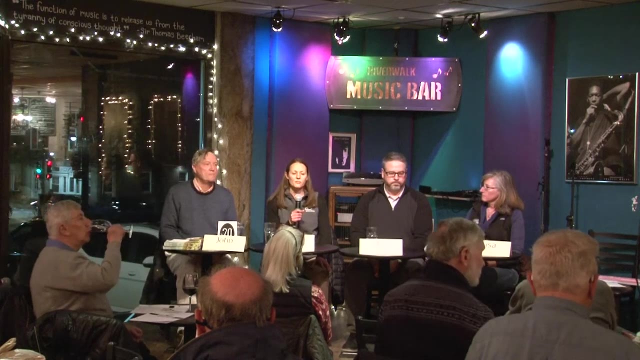 And the bulk of our membership is in New Hampshire and Vermont. We were founded in New Hampshire And the two key aspects of our work is one: we still offer what's called a cooperative marketing and purchasing program, So we do connect communities to the purchases of their recyclables, and that's very unique. 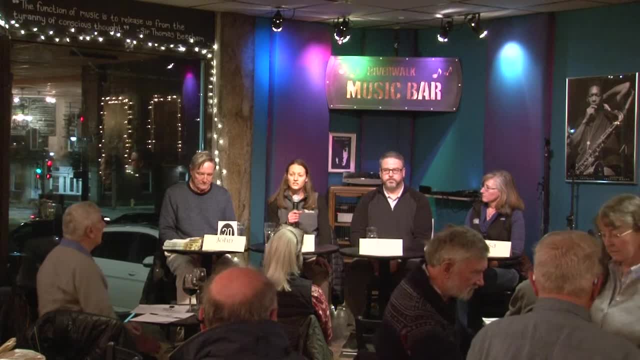 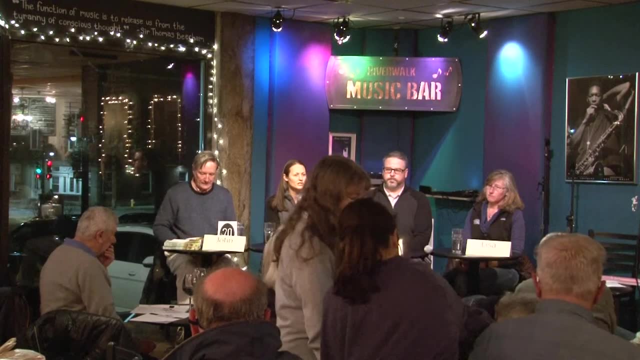 We're one of only a handful of nonprofits in the country that does that kind of work. It's typically done by for-profit companies, So that means that we're very- We're very- uniquely tuned in to what's happening with the recycling markets here in the Northeast. 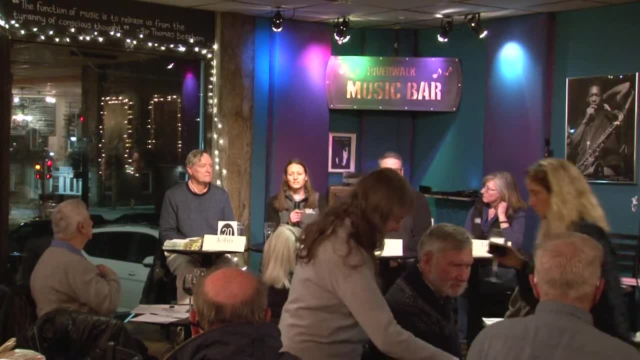 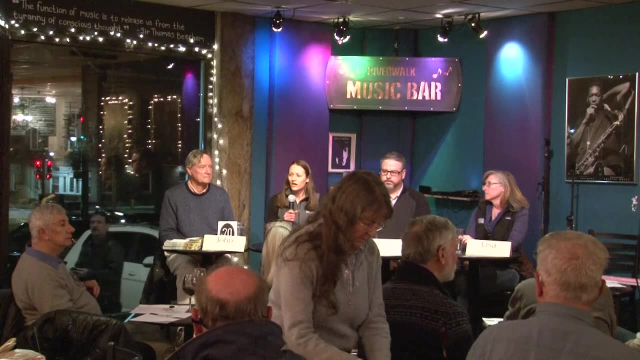 And then the other big piece of what we do is education and technical assistance. So we have monthly meetings for our municipal members to get together and share their challenges and success stories and to learn about what's happening in the recycling markets. We have an annual conference each year. 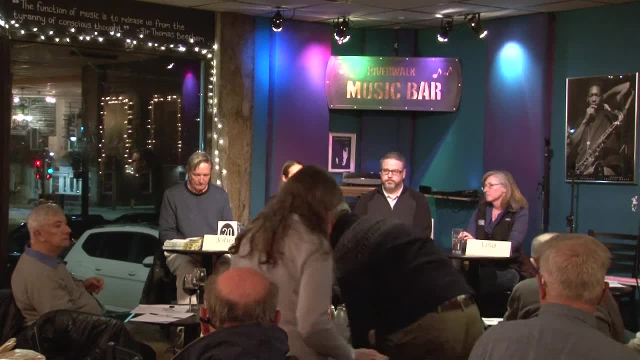 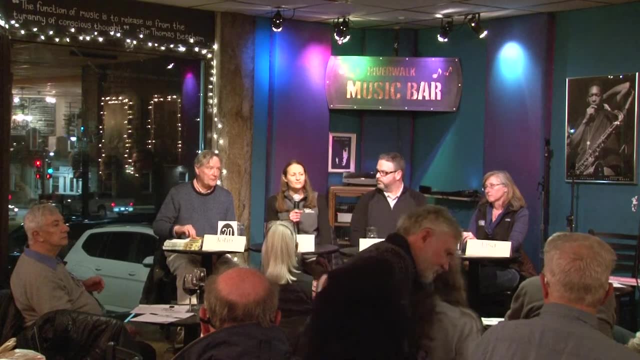 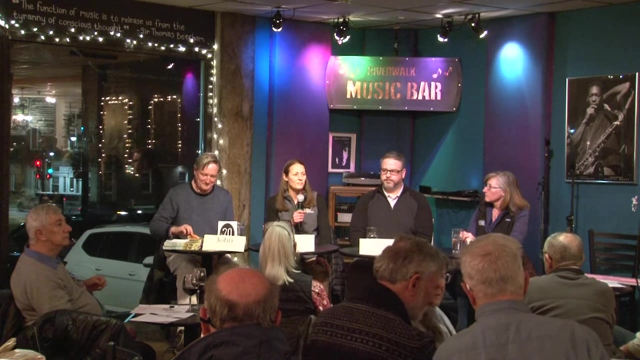 And I imagine that, for those of you who are not already residents of Nashua, many of your communities are likely members of ours, So very happy to be here to talk about recycling and solid waste and what's happening specifically in New Hampshire and how communities are being impacted. 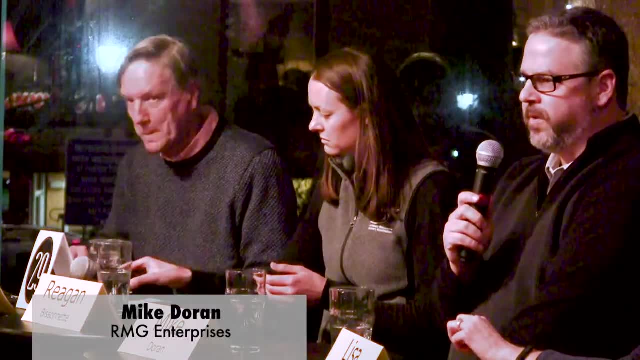 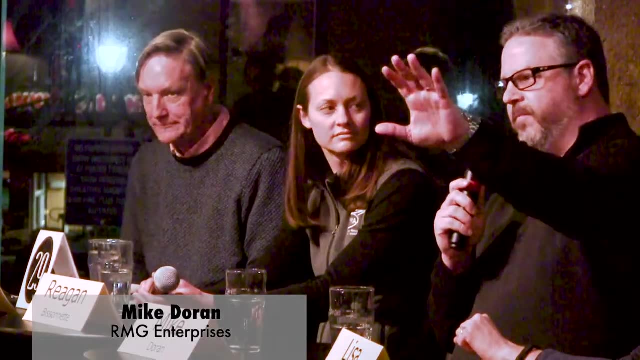 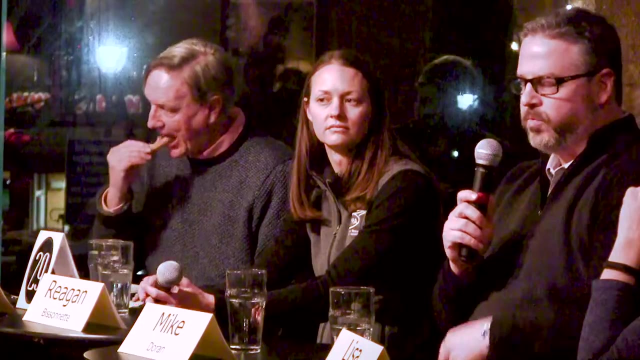 My name is Mike Doran. I'm the business development manager for a company here in Nashua. We're up off of Amherst Street behind the market basket in the old Amphenol building. If any of you are familiar with that manufacturer, they did circuit boards. 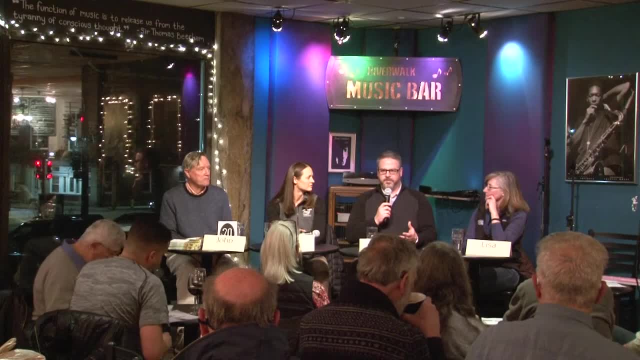 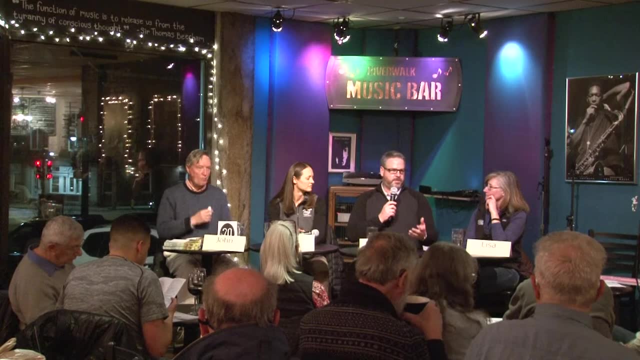 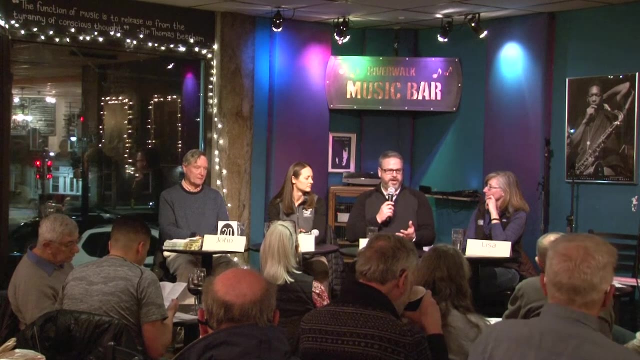 We're in their old space. The focus mostly is on electronics recycling. If you've taken a TV to the local landfill or your business has recycled its computers or computer monitors, it would come to a company like ours And then, depending on the type of device it is, you know it will go through a certain process. 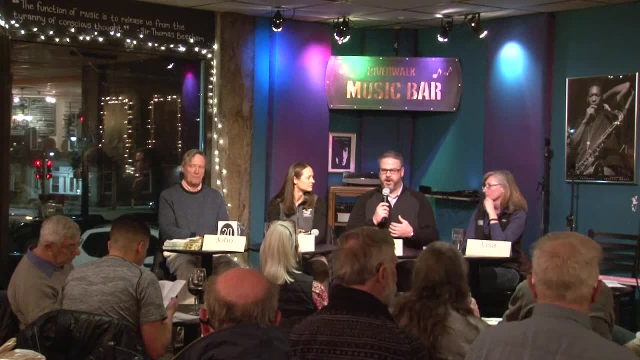 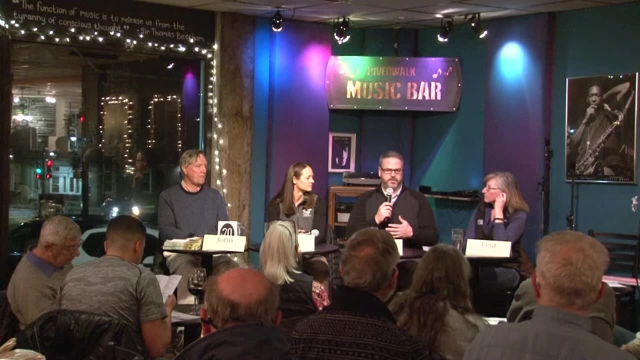 and either we dismantle it ourselves within- you know our operation- or we would work with a partner company that specializes in that type of stream, And the goal is obviously to do that. Oh, there you go, Thank you. The goal is obviously to recover as much reusable commodity and direct that back. 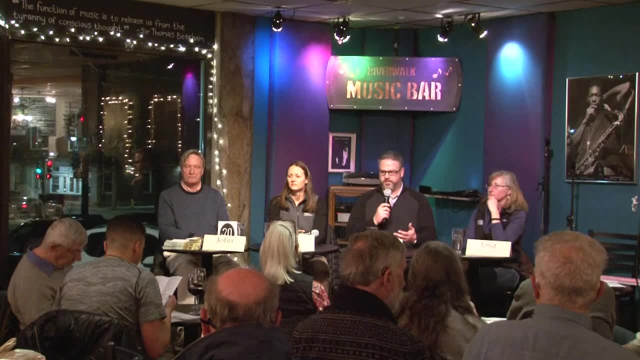 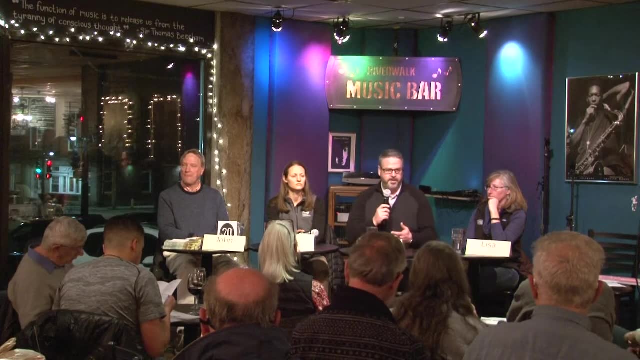 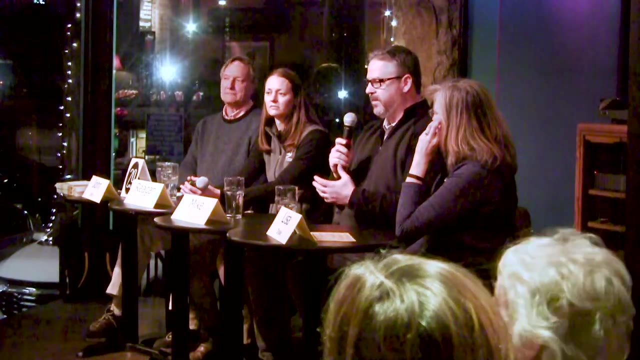 into the recycling stream as possible, But there is waste involved with a lot of this material as well, as you can imagine, Which is why, if you'd have recycled a TV in years past, you had to pay for it because of the amount of waste and the glass and the weight that has to be managed once that TV is dismantled. 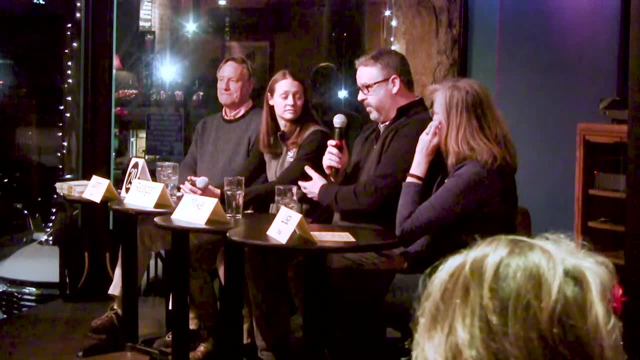 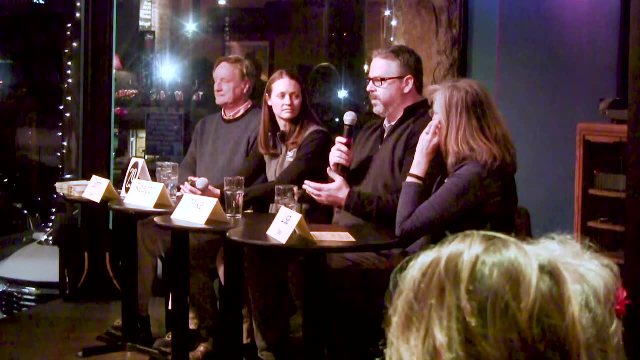 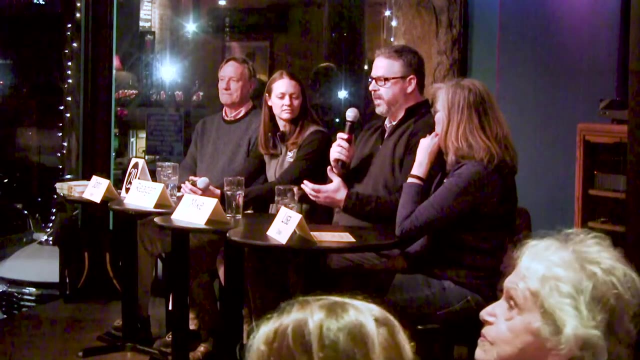 We support, you know, groups like the NRRA: a lot of businesses, a lot of systems, a lot of cities and towns. We're the state contractor for the state of Rhode Island. They have a producer responsibility program where the manufacturers actually contribute. 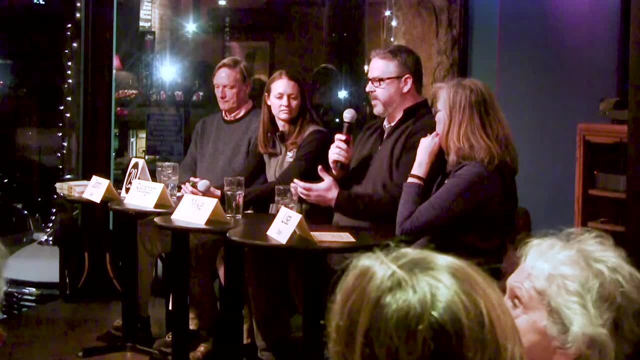 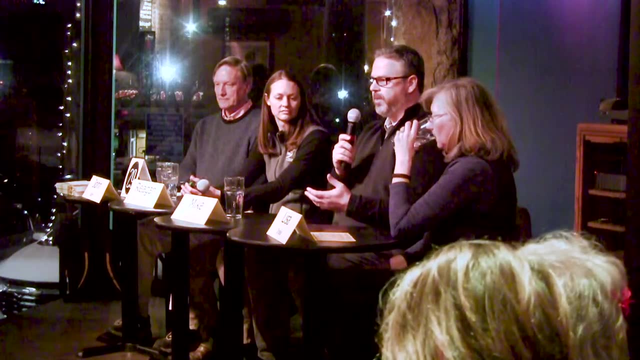 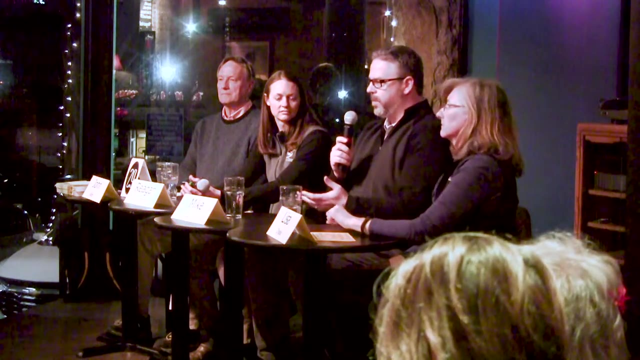 to pay for the recycling of some of these items. that cost a little bit more. We also work quite a bit in Massachusetts with a lot of the public agencies. We're on the Massachusetts statewide contract. We've been a contractor in Connecticut and we do a lot of work up here in New Hampshire as well. 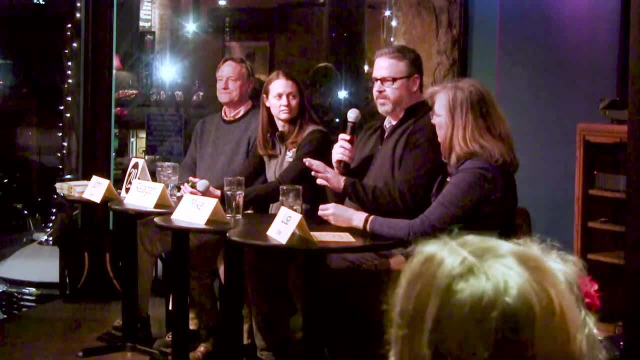 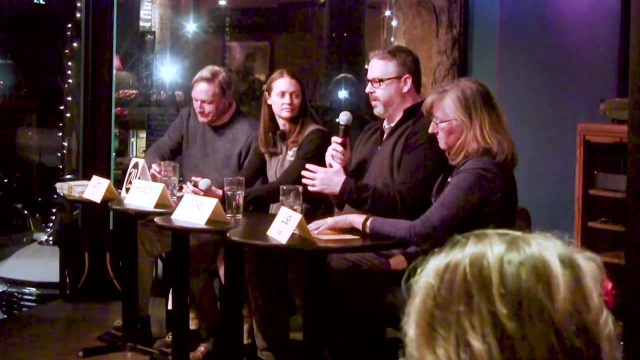 You probably wouldn't see us face-to-face at your home. We're a company that if we're sending out a truck- it's a tractor, trailer or a box truck- We're picking up in bulk. It's not like a door-to-door type service. 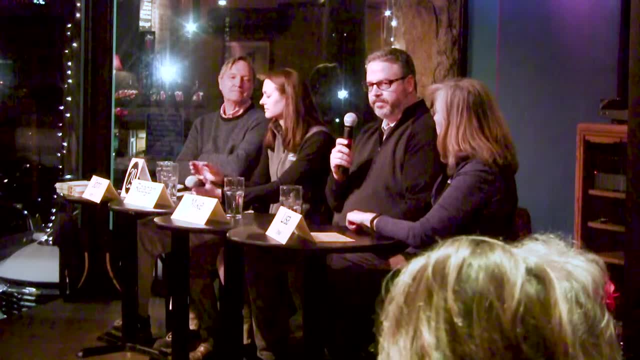 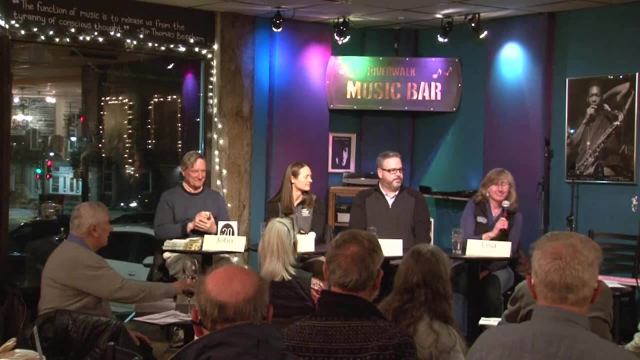 That'll give you kind of an idea of the world that we're operating in. Good evening I'm Lisa Drake from Stonyfield Yogurt and hopefully you all have a great day. I hope you all know who we are and are familiar with our yogurt products. Our history in New Hampshire was that Stonyfield was founded in 1983 on a farm in Wilton, New Hampshire, And the idea of making yogurt was to help support a nonprofit organization on the farm that was educating people about sustainable agriculture. So they had seven cows and they had a lot of milk. and so they started making yogurt to make some money. So now we are, Let's see, 37 years later or so, And we are in Londonderry and we're the number four yogurt brand in the country and the number one organic yogurt. So we're distributing our products all across the country. More than 85% of it is made right here in New Hampshire. We have a few places where we contract out for yogurt to be made elsewhere, And we're founded with an environmental ethic that we work hard to stay true to today. We have a mission to support, to make healthy food while supporting healthy people, a healthy planet and delivering on a healthy business. And so how we interact with this topic of recycling solid waste. of course we do create waste And we have had a recycling program in-house. 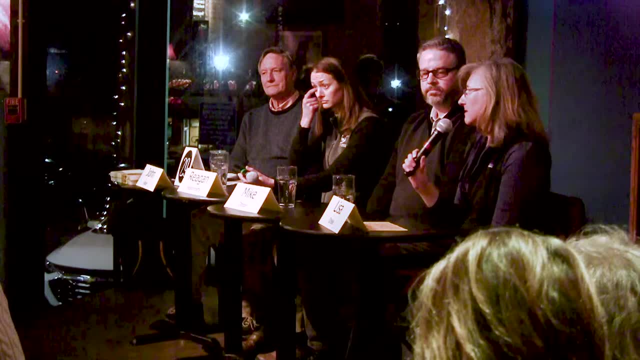 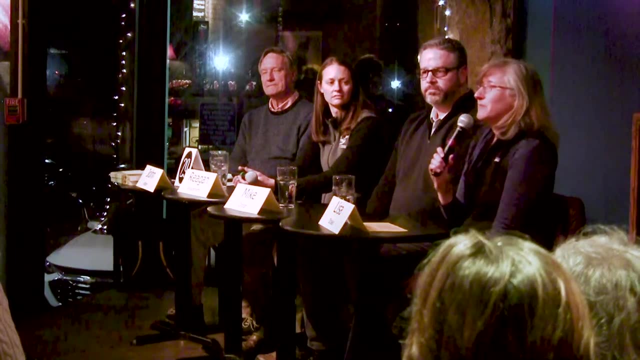 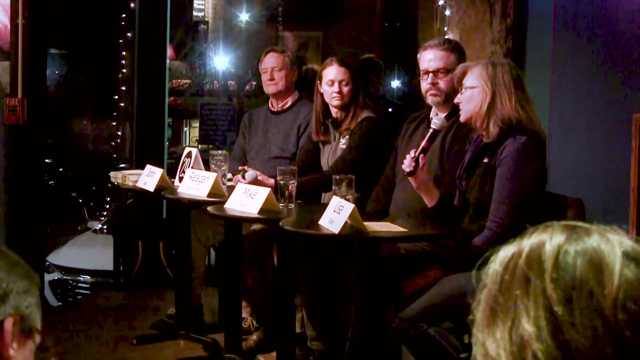 for about 30 years now, So I could talk about some aspects of that, but I think the more interesting aspect is that we're very conscious of the fact that we create waste that go into your homes, That the packaging, packaging that we use- is the way that we get that product home to our consumers and get 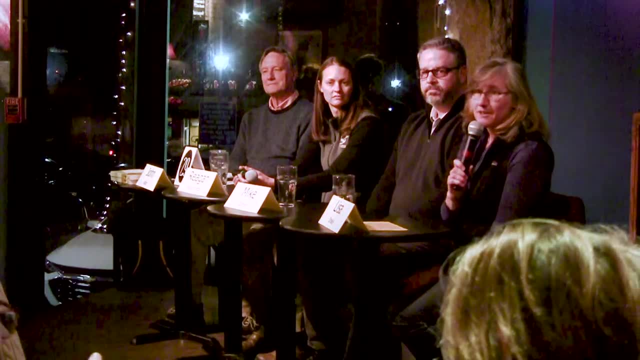 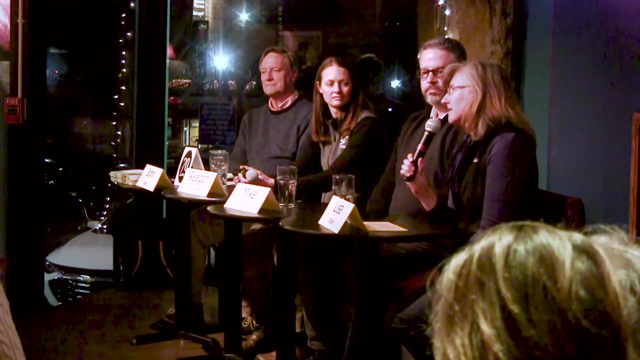 it there in a way that is safe for the food, in a way that gives you the information you need to know about our product and attracts you to buy our products. So there's a lot of considerations that go into packaging, but certainly we're very mindful about the. 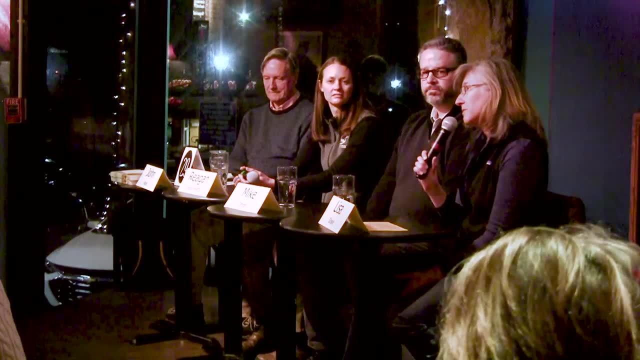 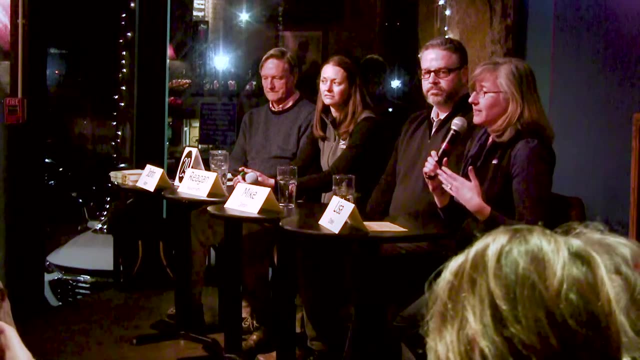 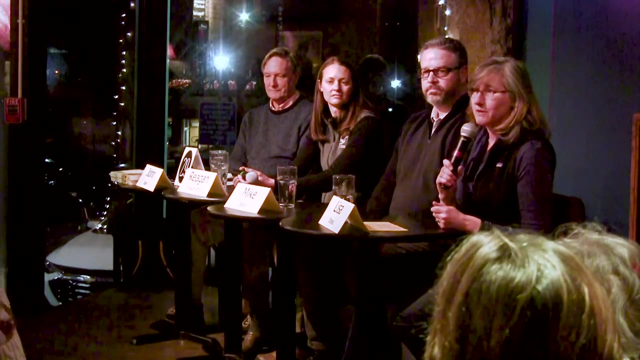 environmental impacts and the waste impacts associated with those choices that we make- And so that's just one example of my job in sustainability- is: how can I help the company operate in ways that we're mindful about our impacts and that we are doing the best we? 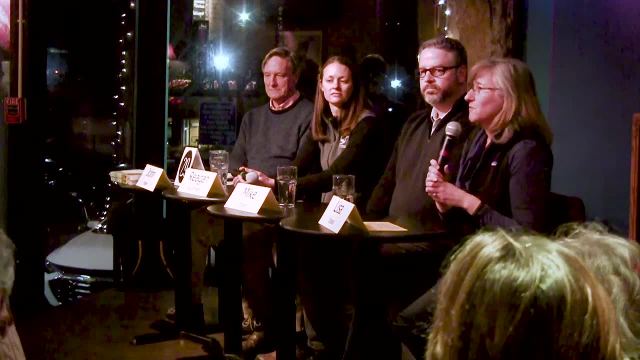 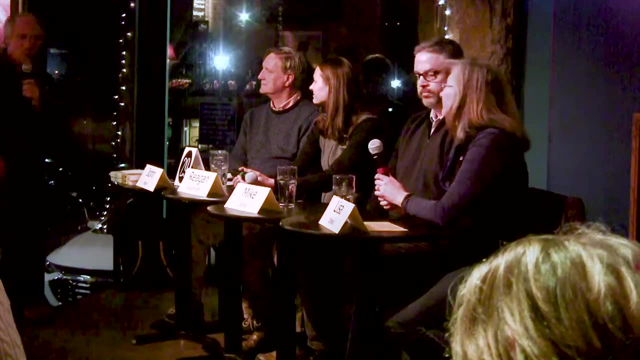 can to be sustainable in the long term for the environment and our communities and our supply chain. So that was great. What an excellent panel. Who wants to start? Does anybody have a question for the panel? Thank you very much for the panel coming in with all the questions. Just broad level of expertise. My primary question, I guess, is targeted for Reagan and Mike- With the recent political changes and the shifts in the offshore recycling, I'm thinking specifically of China, the destination for many of our very toxic recycled items. 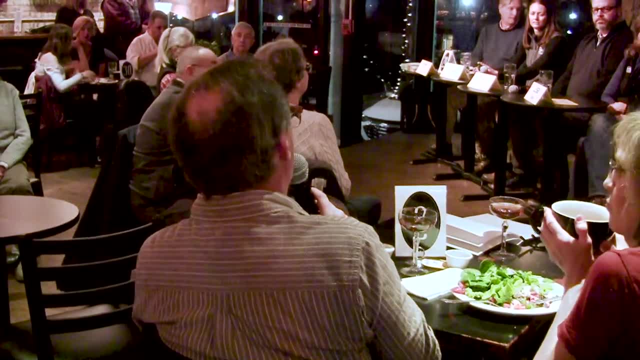 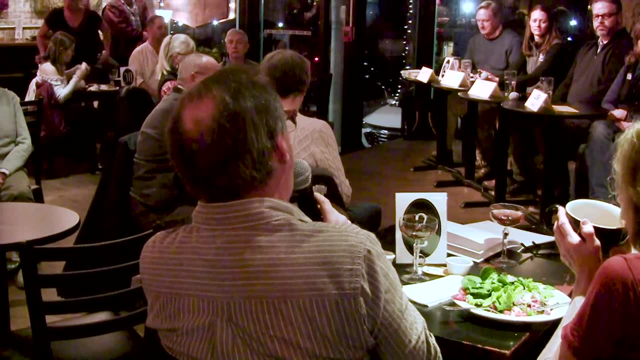 what percentage do you feel of the waste and the recycling that we produce in New England is being turned around in the local economy? Yeah, Yeah. So I think that the question is how much of it is being taken from the local areas by some of the companies and how much of it is going offshore, And are there challenges? 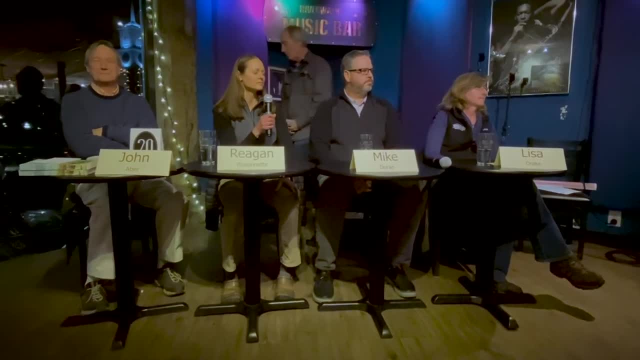 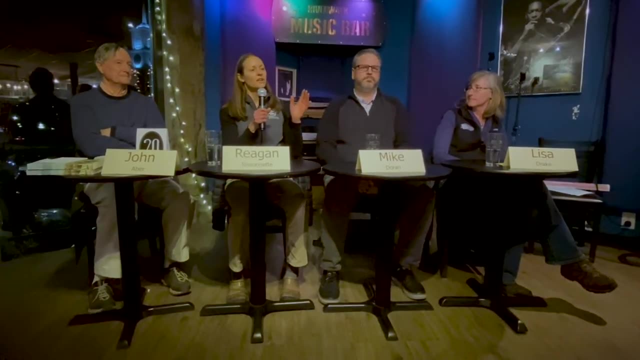 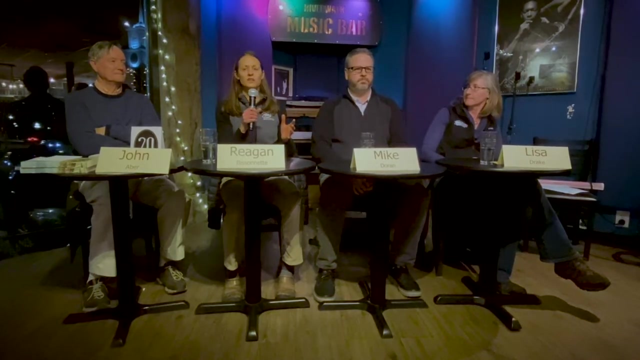 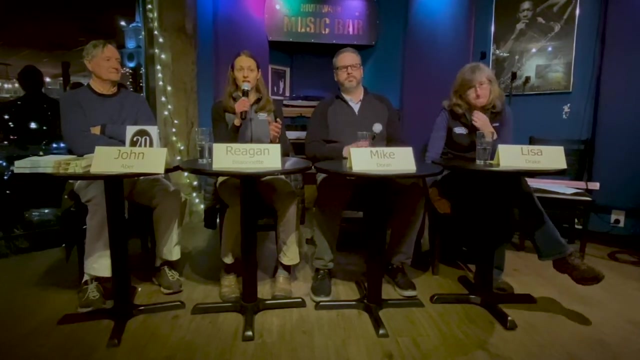 in that new political economic model. So, just to start off, as many of you may know, at the beginning of 2018, China stopped importing all unsorted mixed paper, all plastics and some other materials into their country. I think we're going to talk about that in a little bit. 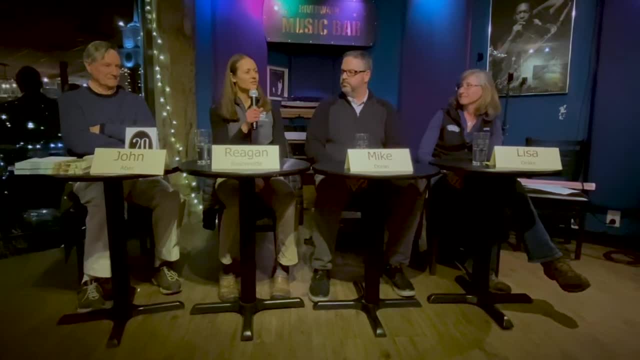 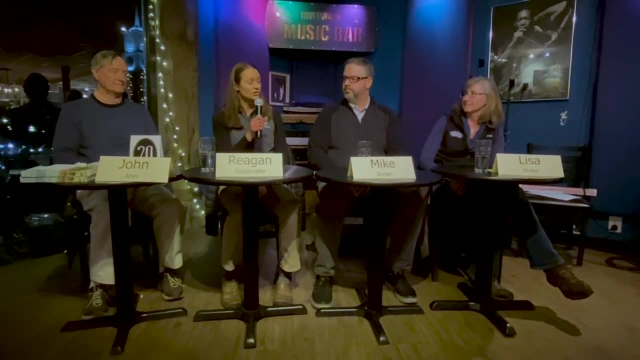 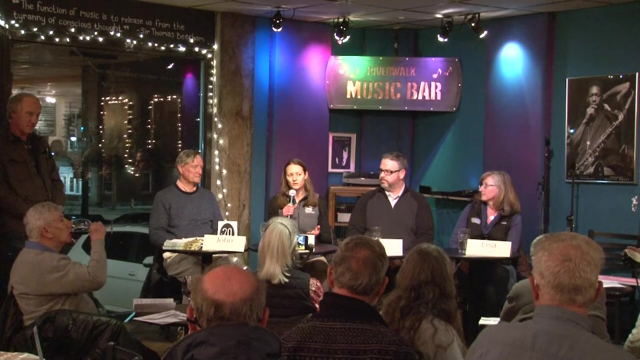 Can you get closer, Please Now? when that happened, China was one of the largest purchasers of recyclable material for the entire world. So, just as an example before this policy, it's called China's National Sword. before this ban was implemented, China purchased over half of the entire world's. scrap paper. So that's massive, And so what happens is when your largest buyer stops buying, We had this massive oversupply of material, And so that, in a very simple nutshell, is why we have such a reduced value of recyclables across the board right now, is primarily tied to China, the world's largest buyer of recyclable. 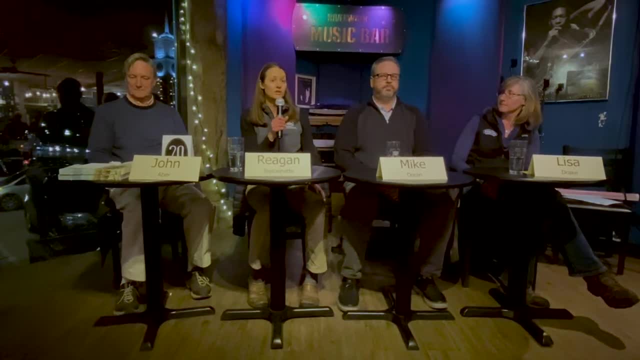 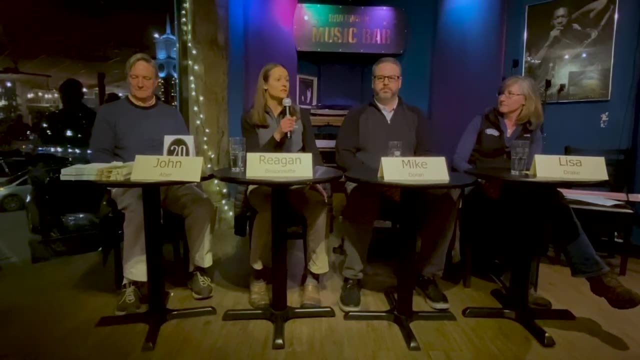 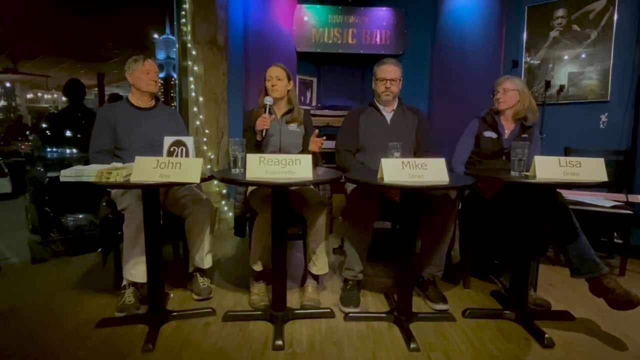 material, deciding that they no longer wanted to import certain material. So what that means is that temporarily, some material is being thrown away if it can't find a new outlet. We did see, for example, with mixed paper. when I say mixed paper, that is your office. 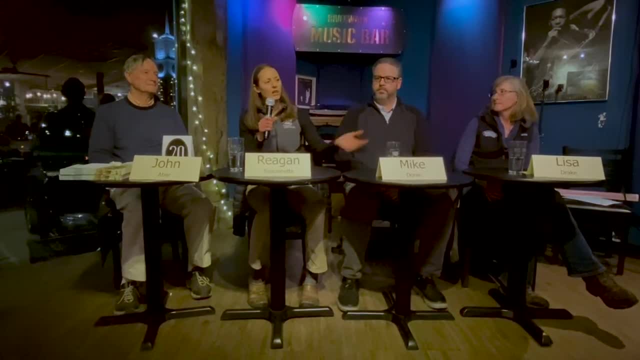 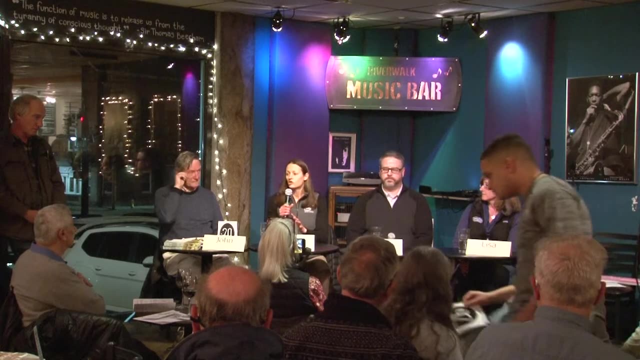 paper, your junk mail, your newspaper, your magazines, all of those mixed together. When China closed its door to that material, India became the next largest importer of that material, And so there was, you know, a new market, a new buyer, who was? 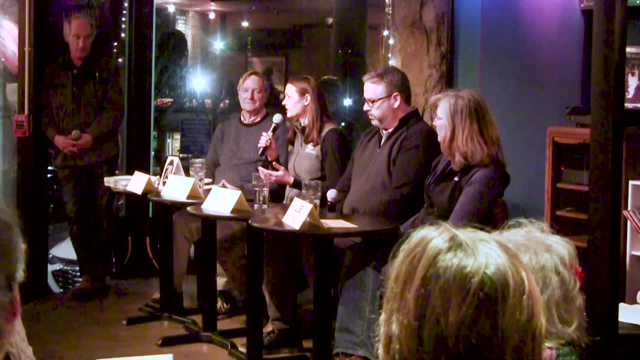 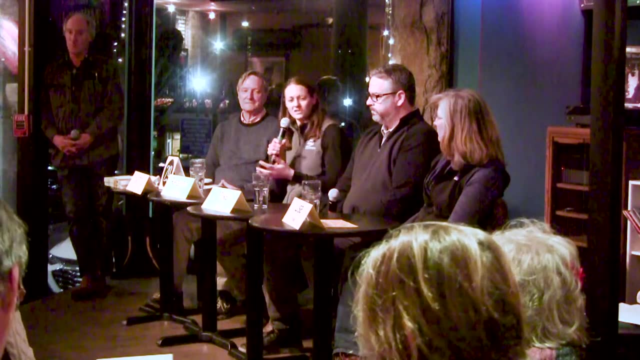 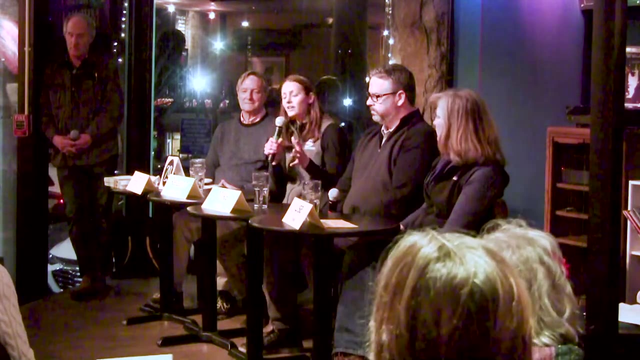 going to take up some of this excess supply. We're actually seeing just in the last month or so that India is tightening its restrictions as well, So we still have this oversupply of material. Now the silver lining is to the extent that material like mixed paper is not already being. 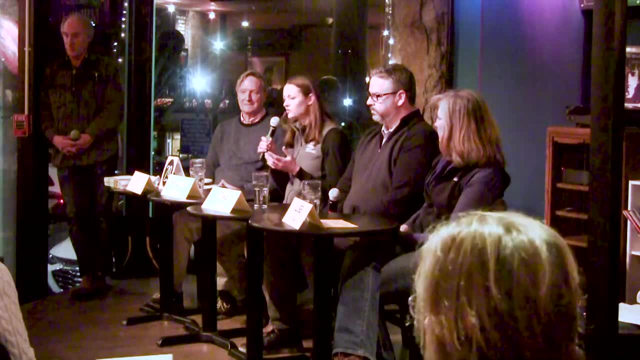 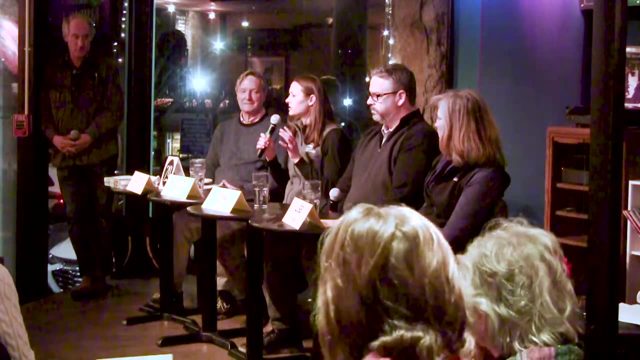 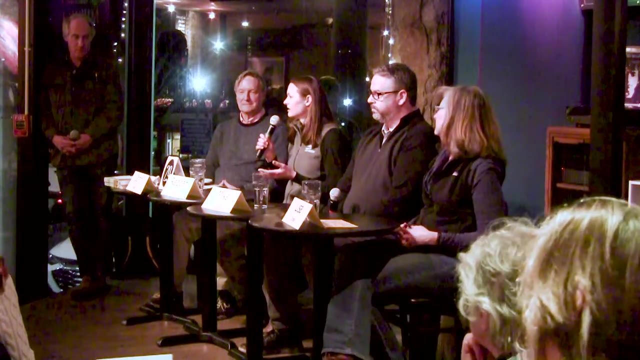 used as a feedstock for new products. in the United States, there's actually 22 new or existing paper mills that are Okay Being developed in North America that are going to use cardboard or mixed paper as a feedstock, And so they're going to start taking up some of that excess supply. 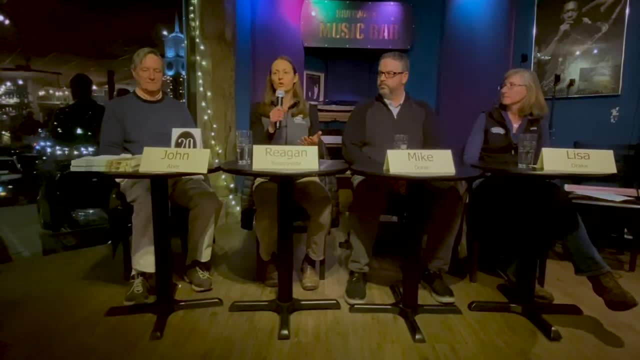 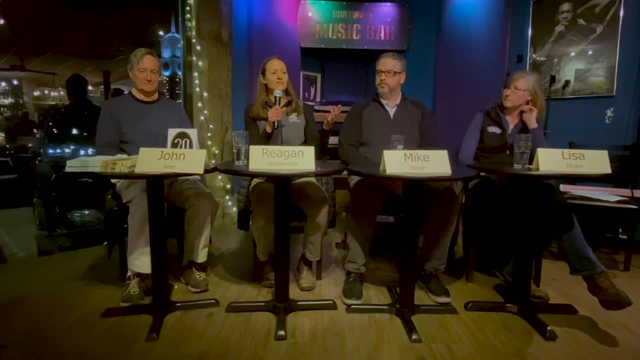 And you know, the predictions we've heard from the vendors that we work with is that we can expect by, hopefully, the end of 2020, maybe the beginning of 2021, that we're going to see an improvement in the value of that particular recyclable commodity. 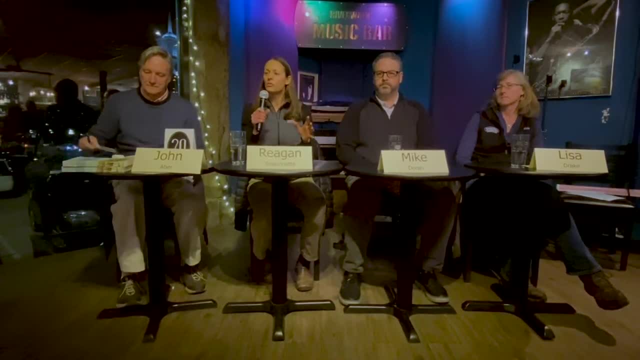 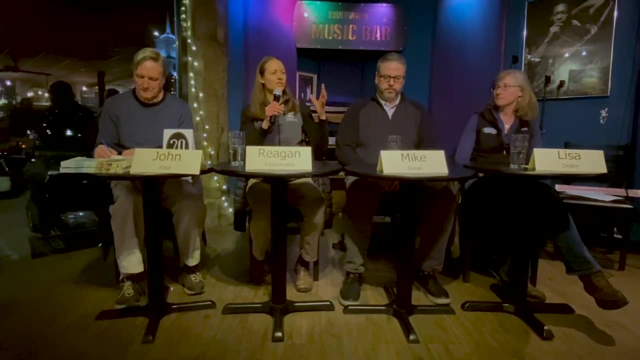 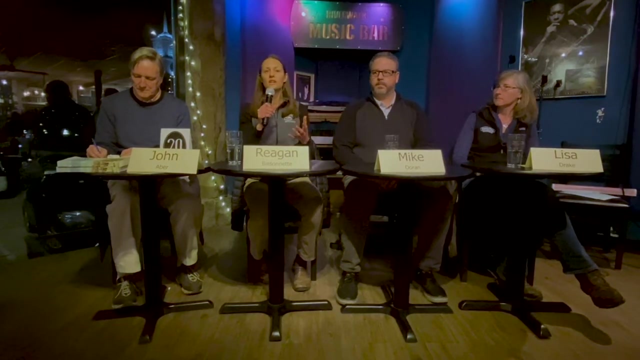 And the reason I'm talking so much right now about mixed paper and cardboard is because, again, we've got to look at the entire pie of what are the recyclables that we generate as individuals- Municipal, you know, municipal- solid waste. What are the recyclables we generate? 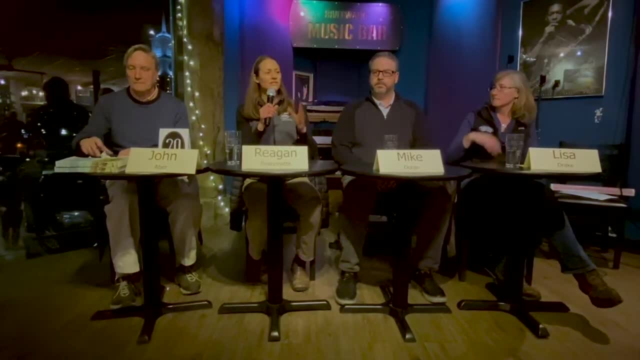 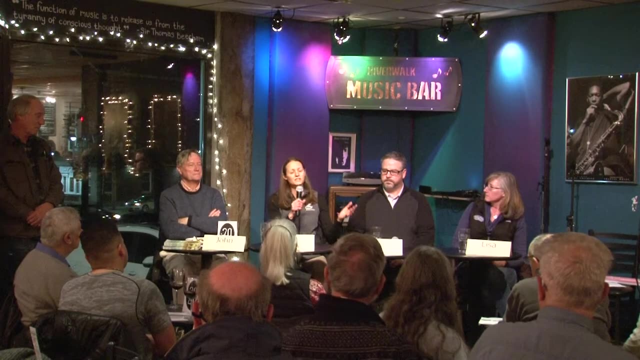 Half to more than half of it, maybe half to 65% of it, is cardboard and mixed paper. So we are seeing domestic improvement in recycling infrastructure. It takes time for new factories to be built. We're also seeing, for example, over the last year we've had a significant increase in 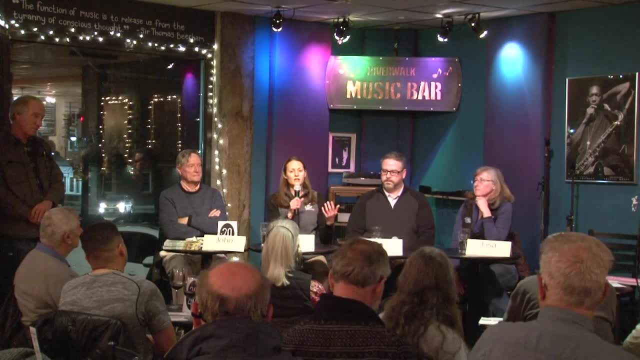 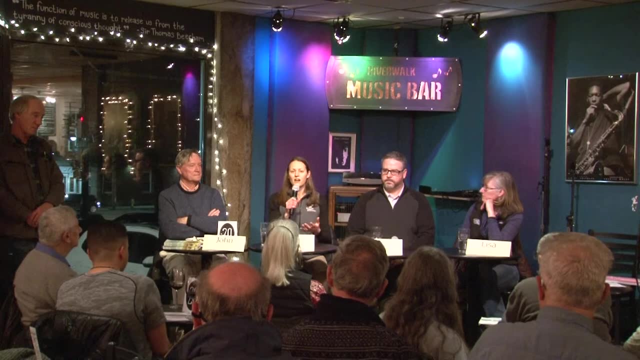 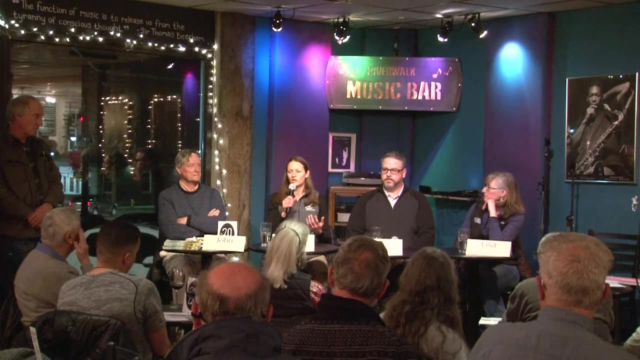 a number of new facilities across the country that will be used to recycle plastic, so those things are coming online, and i do think that the silver lining of the challenges we're seeing right now with recycling is that we as a country are going to be doing a better job of managing our 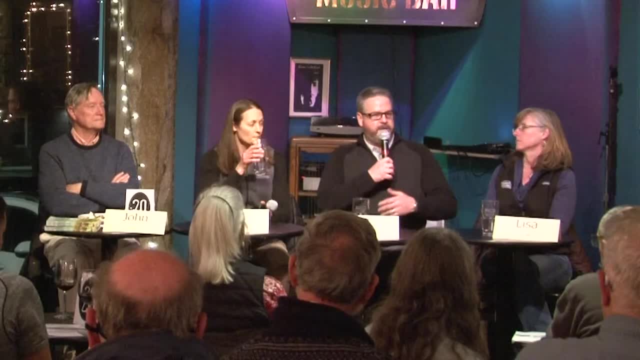 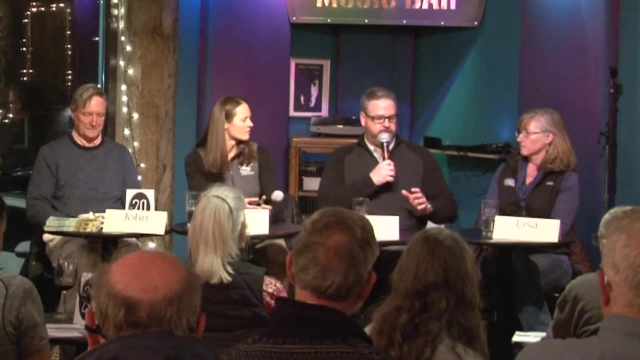 recyclables. you know our waste stream is obviously a lot. our waste and recycling stream is obviously a lot different than the. it doesn't have quite the diversity that that reagan does. it it's um. you know we're dealing with electronics and circuit boards and heavy metals, but there's the smelting. 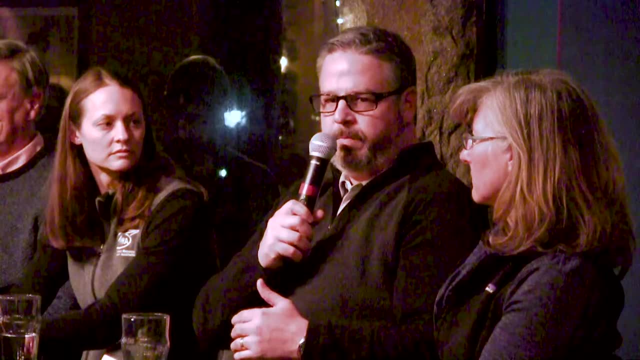 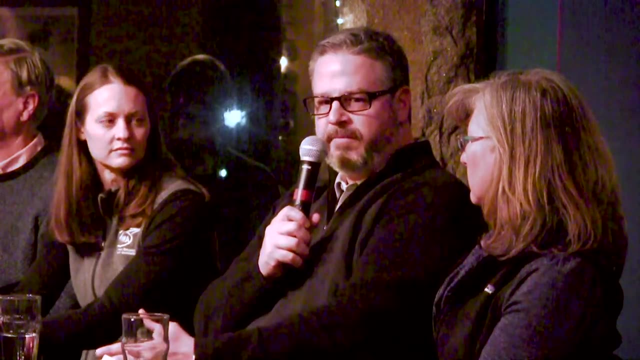 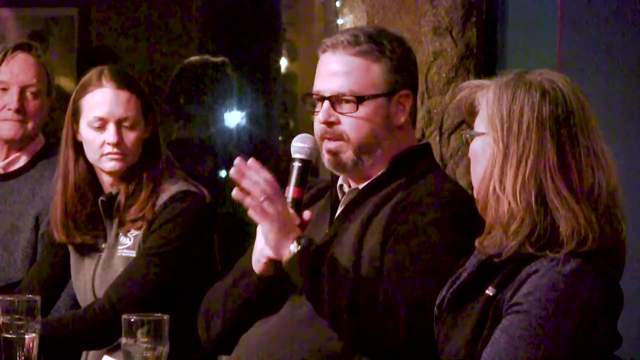 operations that have been around for years. the prices have definitely been affected, but as long as there's a market for it, let's say like plastics, for instance- um, as long as there's a market for that product, whether it's you know, china shuts down and um, there may be another outlet in another. 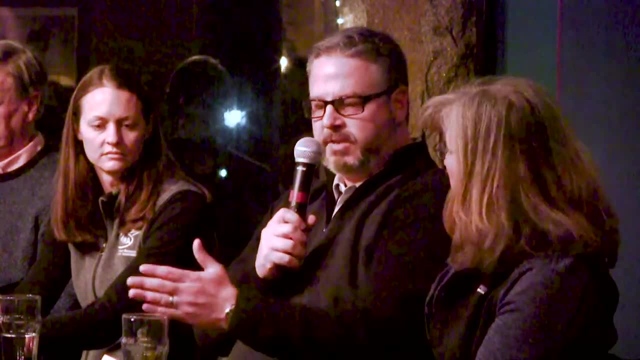 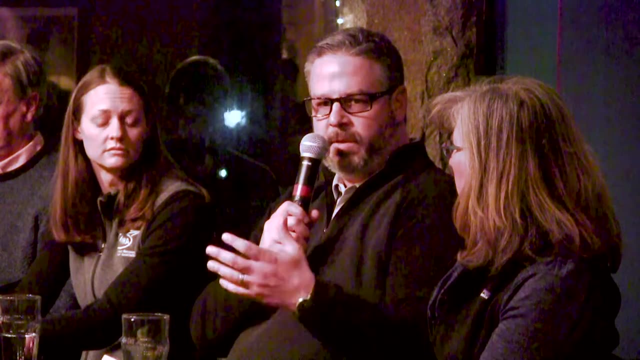 country and there's a broker that'll get the material there as long as it's it's. it's a vetted and outlet that is willing to recycle and reuse the material. those options there, but if those shut down then the alternative is landfill or hazardous waste. 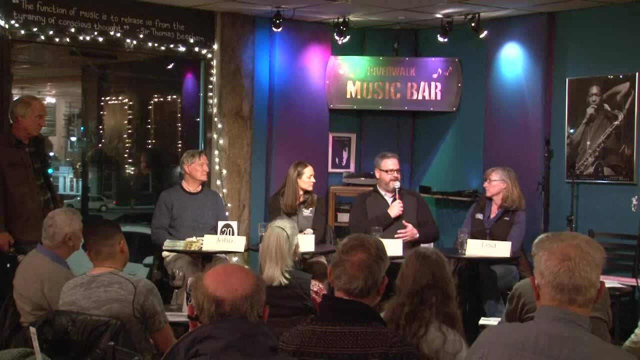 landfill, depending on the on the waste product. it's not as complicated, it's just. it's a matter of economics and it's a matter of are there markets for the materials and is there a waste stream for the material? and it's up to us to kind of manage and evaluate which which way we want to. 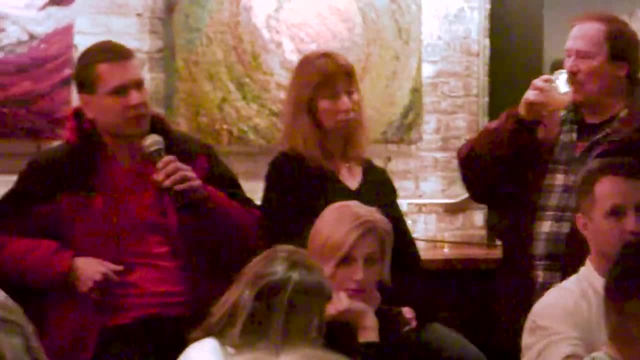 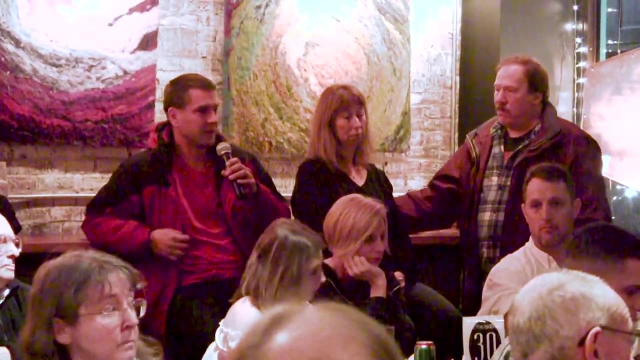 send our product. i'll try to keep it brief. i'm a selectman in hillsborough and on the solid waste advisory board, um, so we've uh stopped recycling glass a number of years ago because, as an nra member, there was no place to bring it. we stopped recycling plastic because the costs were just astronomical and 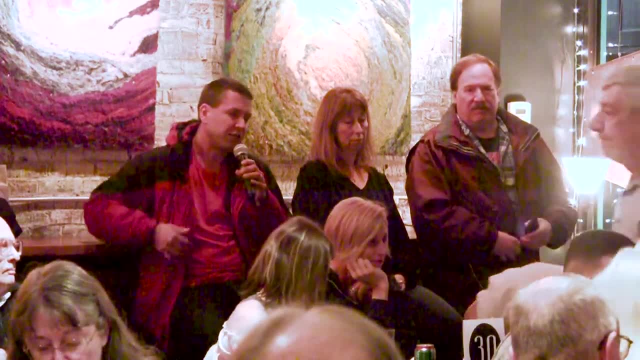 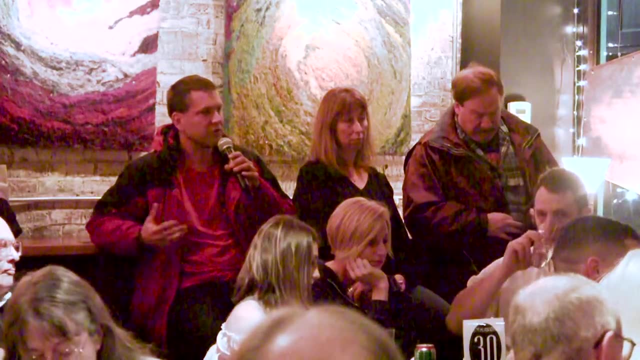 the unknowns of where it goes. we were trucking it up to right river junction. there was no place closer. so that's um quite a lot of trucking fees. it's three times the cost to recycle the plastic than to put it in the trash, can um so and we, we made the decision, the hard decision, to send it to. 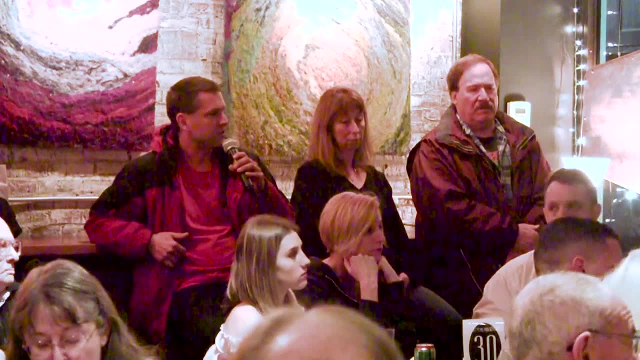 it's pembrooke or pentecook, the incinerator, which is where our trask goes, so at least we know where it's going, versus the. I'm told by this lady that none of our plastic has actually been going overseas because it's West Coast stuff. 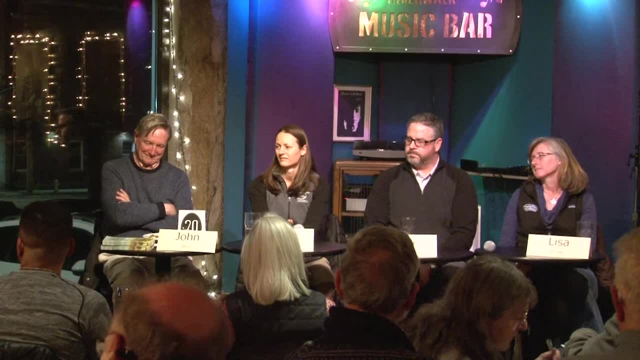 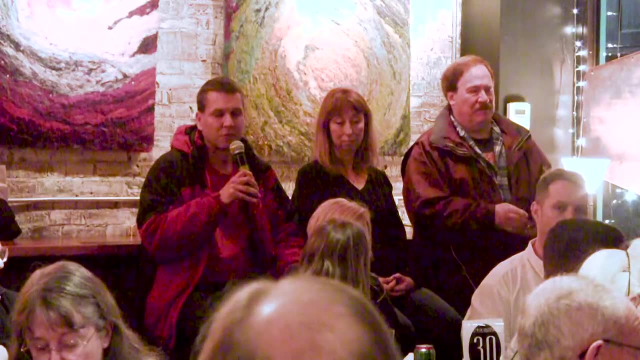 so that's good. but there is a bill that we started in New Hampshire to a committee to study the feasibility of a regional plastic-to-oil. Hillsboro is pretty small. The numbers we've gotten are too big for us probably, but not totally out of the picture. but as a regional 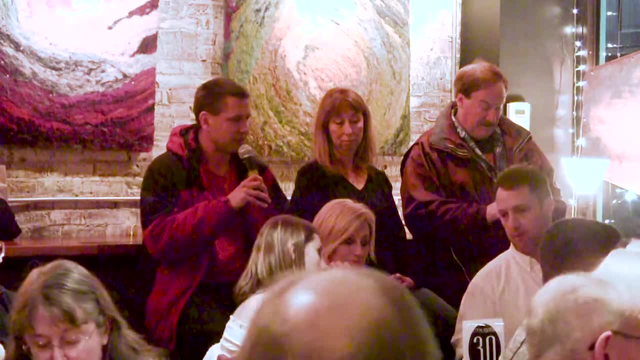 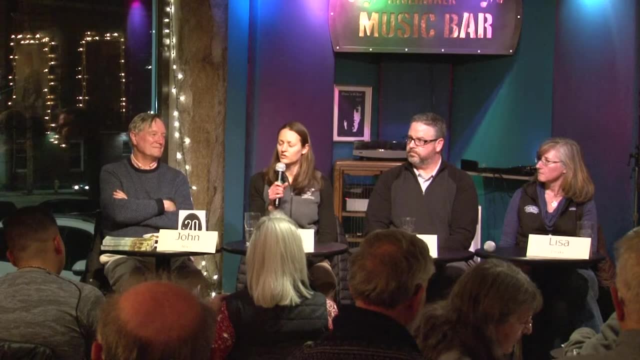 thing that might work for this whole plastic-to-oil thing seems like an interesting idea. so I don't know how many of those are questions and statements and things. What I can say is that again, it's all very individual to communities, but as a general rule, if you're separating out your material, we 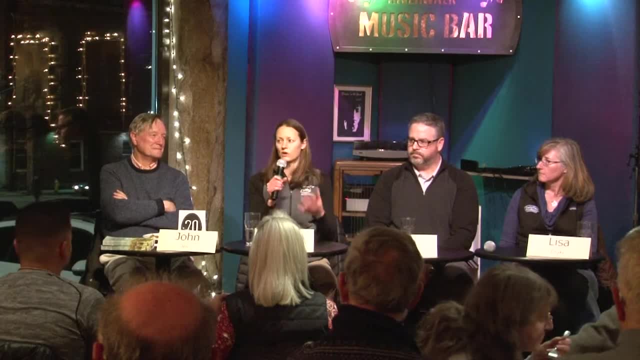 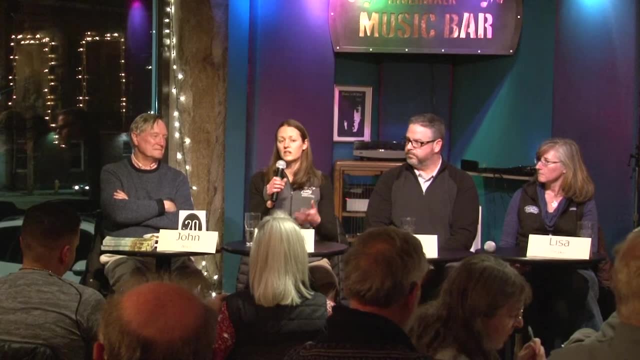 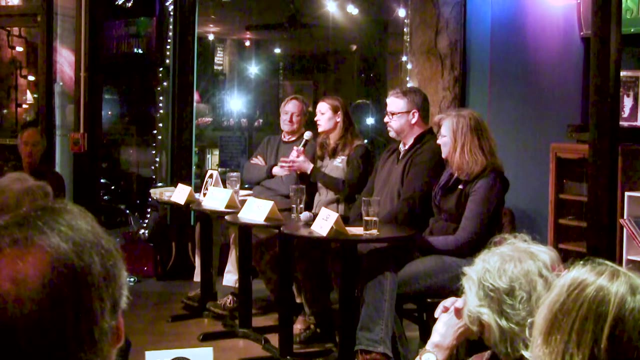 have yet to run into an instance where we've been unable to market that material. so there are a number of communities near you that are separating out their glass and they're either sending it to one of our consolidation sites to be turned into fiberglass insulation, or they're sending it to a 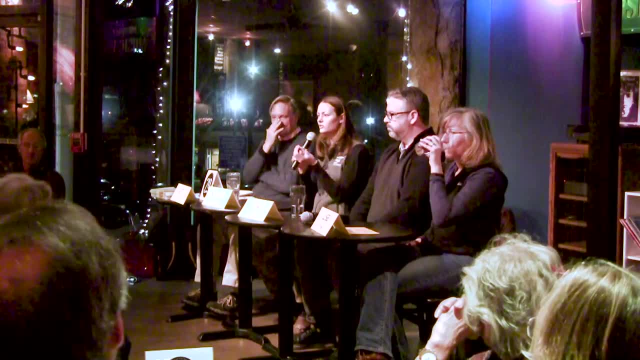 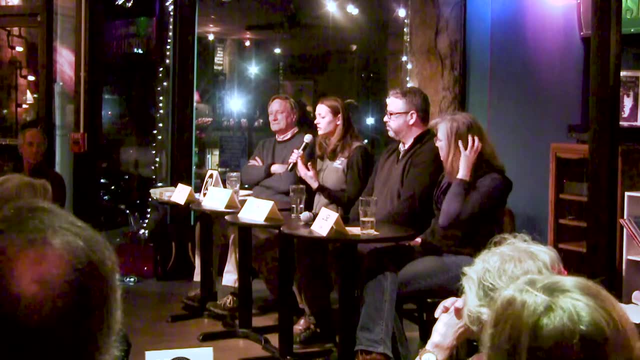 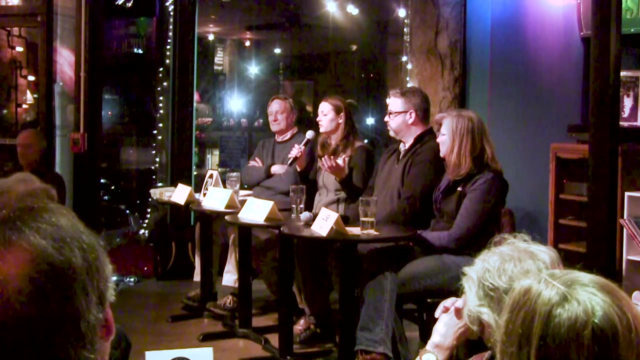 consolidation site where the glass gets crushed and used as an aggregate in road and infrastructure projects. So there are a number of communities in your area that are participating in that program. As far as plastic goes, there is a big difference between how you separate out your plastic. So, for example, if your community mixes all of its 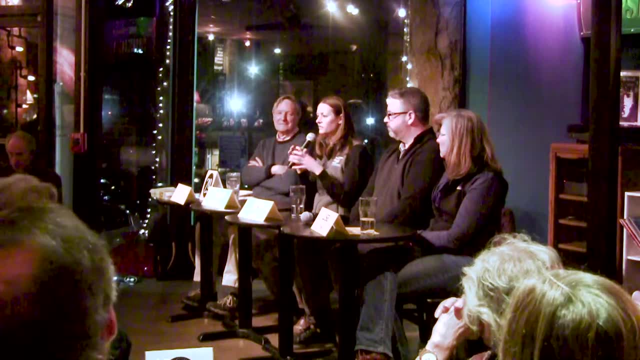 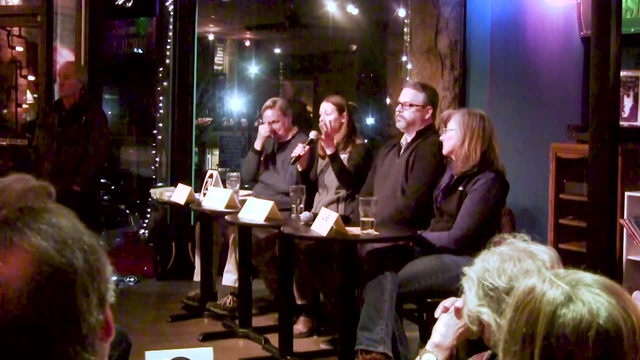 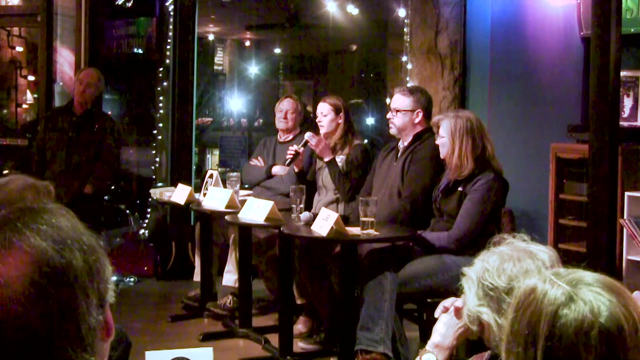 one through seven plastics together and then bales that together and sells that as a commodity. you'll get a lower price for that because again you're outsourcing it to someone to buy it and separate it for you. but right now, if communities separate out, we have many communities that switched from doing a one through seven mix and now they 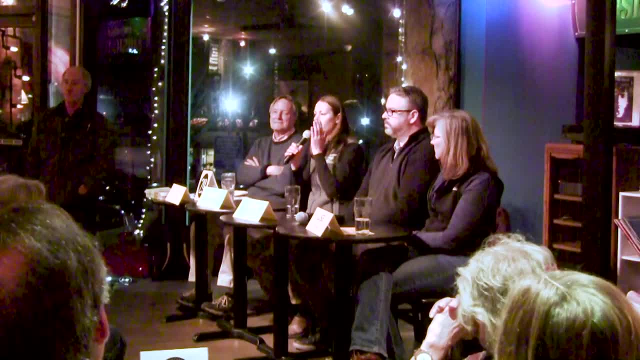 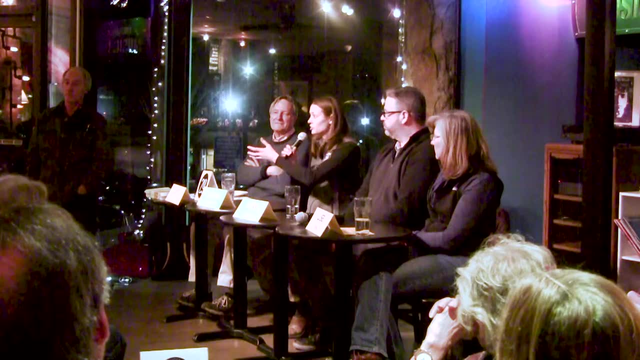 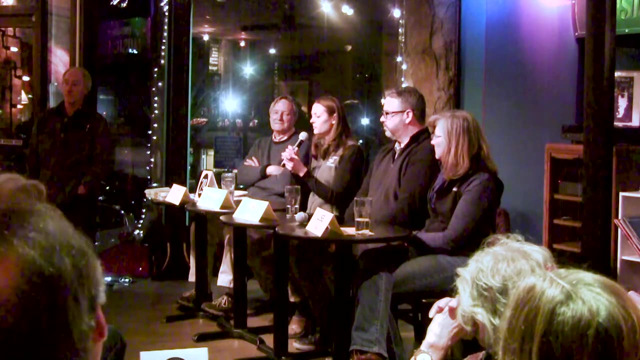 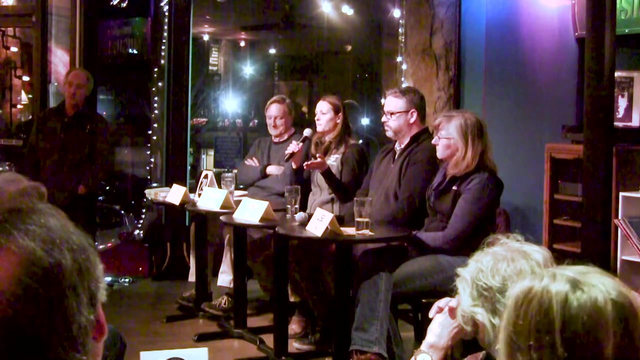 just separate out their number one soda bottles, their number two natural milk jugs and their number two colored, which is, you know, your detergent bottles. and if you just separate those out there's quite a bit of value in those material, whereas there's not as much value in the three through seven plastics. So right now, when you look at sort of the average blended ton. if you look at a ton of recyclables coming out of a municipality, the smallest by weight are your plastics and your aluminum cans and metals. That's where most of the value is right now in terms of financial value, whereas, as I mentioned, more than half of that pie is mixed paper and cardboard and you're having to pay to get it out of your 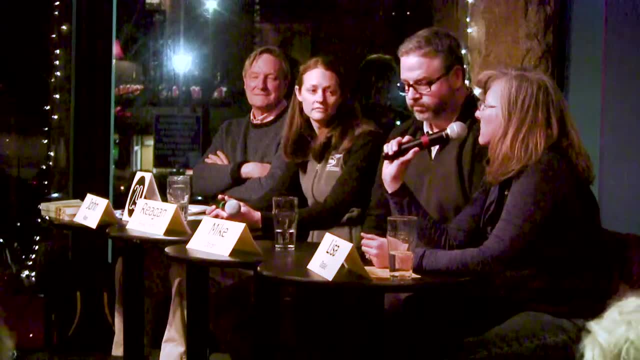 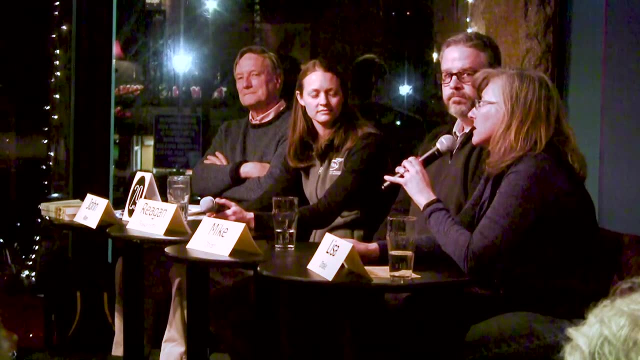 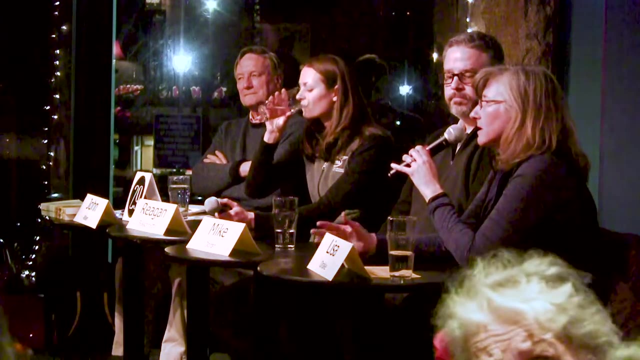 community to get your mixed paper recycled right now. I just wanted to add a thought. This idea of plastic to oil is interesting. You know we've also been watching development of chemical recycling developing as a technology. So recycling that is generally done today is a physical practice. It's you know. 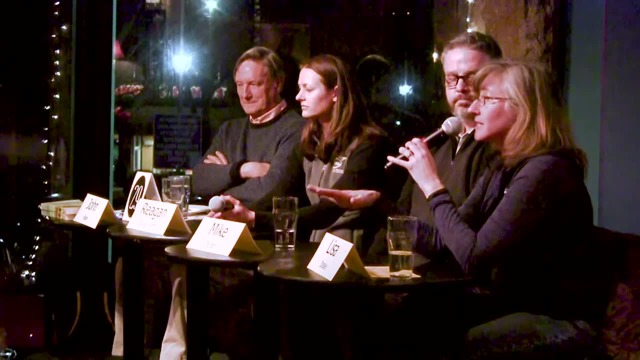 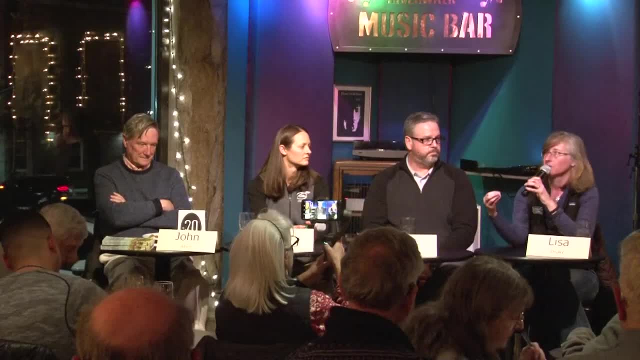 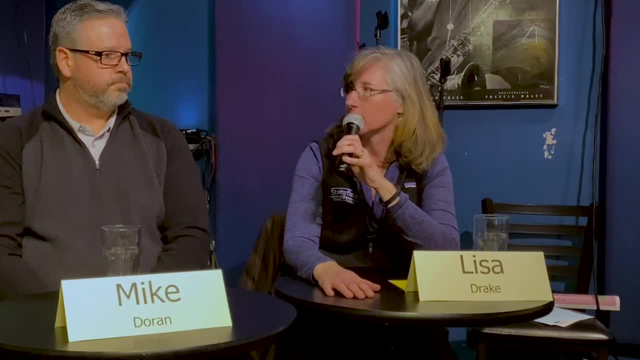 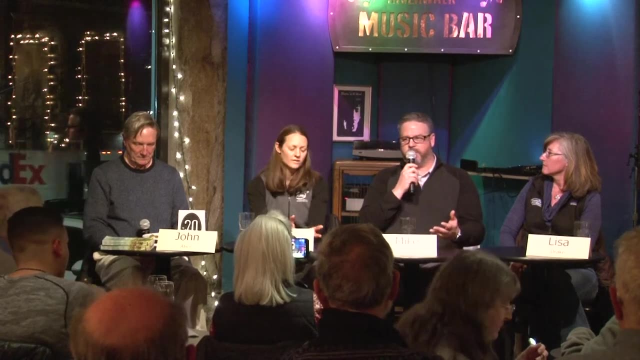 And so you know, by true выбrow orThis will bring in a lot of the재 position at the rapid forward movement. so people will come back through the re Diane. I would also say on the, the plastic, it really kind of depends off on the price of oil at the moment as well. if the, you know, if if all of a sudden fossil fuel, 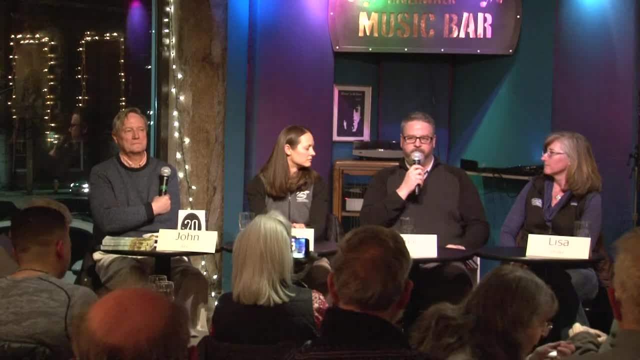 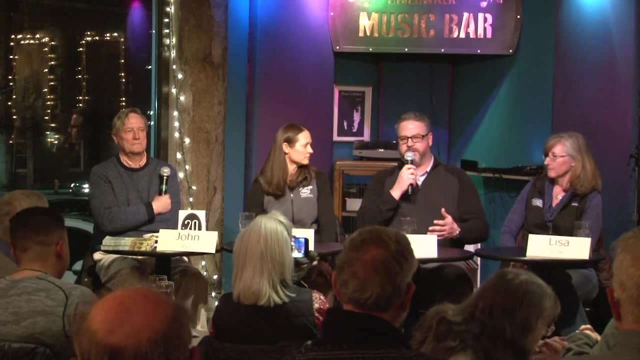 prices go through the roof. you're going to see a lot of entrepreneurs get into the plastics recycling business if they can recover oil from it. So there are other market forces out there, other than just how the material is sorted, how it's collected. it's where is the demand for the 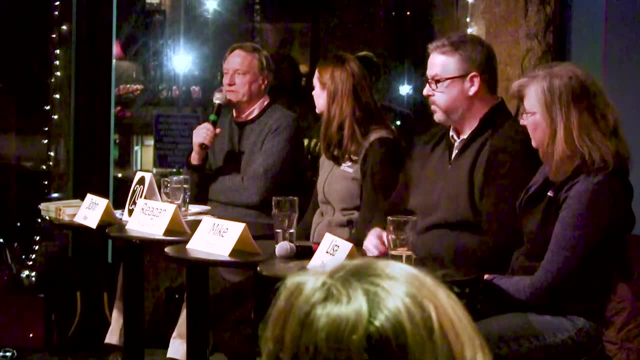 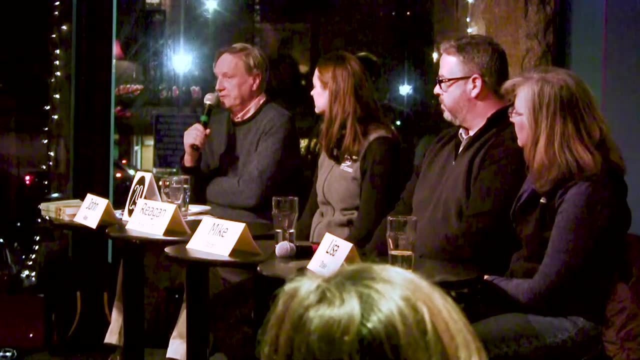 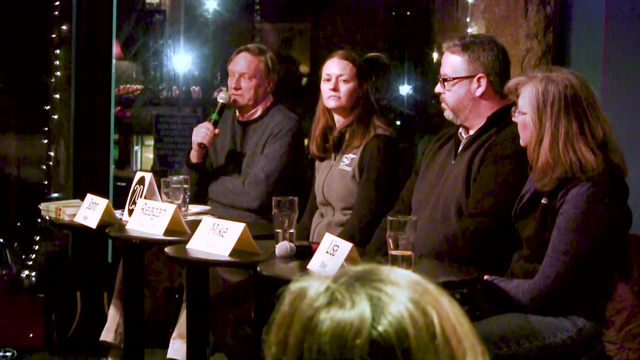 material and what drives it. a big part of most municipal waste streams is organics and durham, at least, is considering trying setting up a composting system, which most european towns and cities have. they almost always have an extra bin for compostable materials. durham estimated a 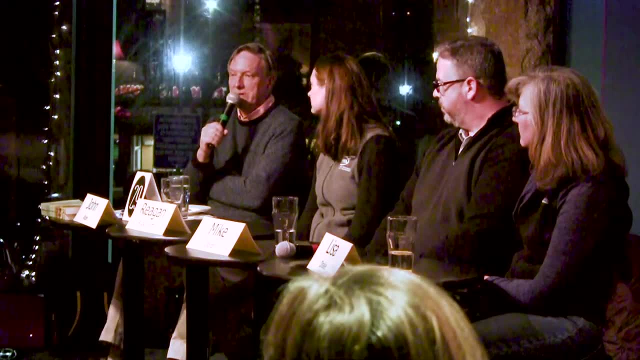 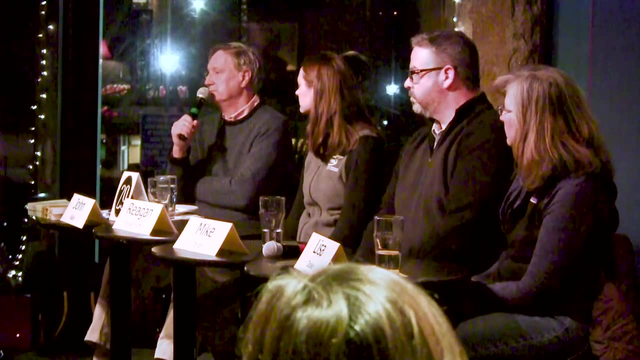 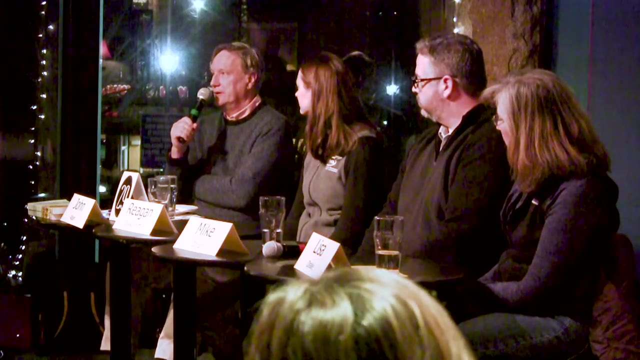 quarter of their weight is or is compostable. so, and that's probably not even dealing with some of the things like papers that are at least possibly compostable. so, um, and i know in vermont and massachusetts there's now restrictions on the uh putting of organic waste from restaurants into. 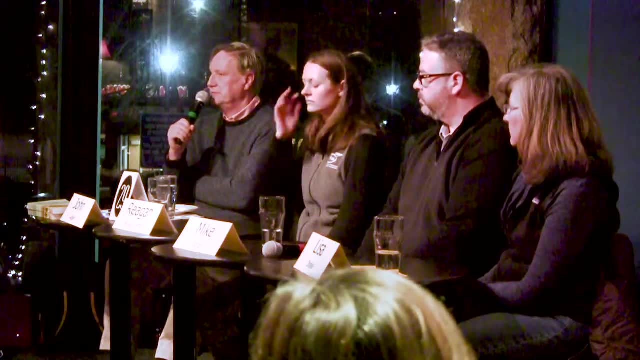 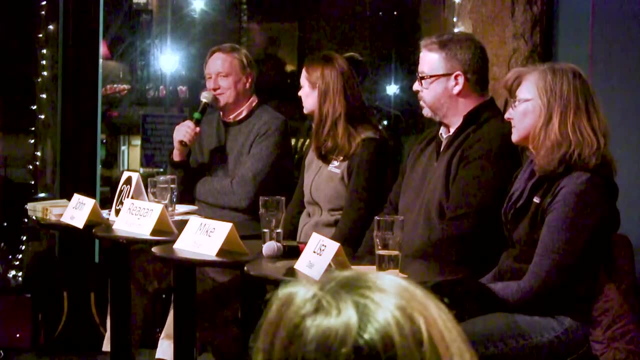 landfills and i guess that is going to probably get stricter so that there will be more material for composting. and there are some companies- mr fox in maine and there's city soil in boston- who are making, you know, a business out of composting now recently that 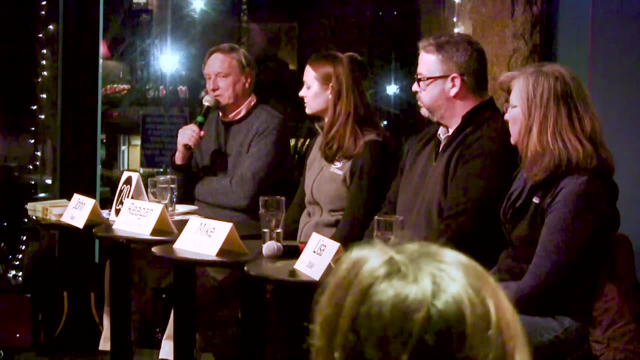 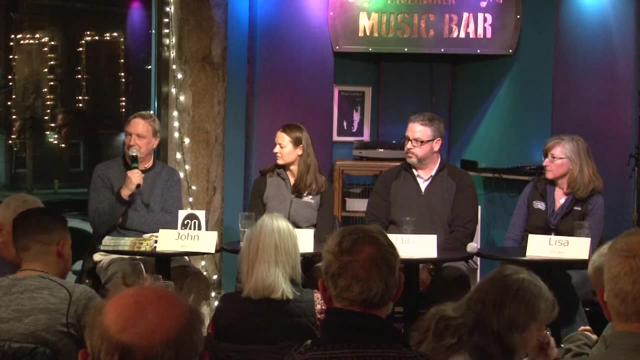 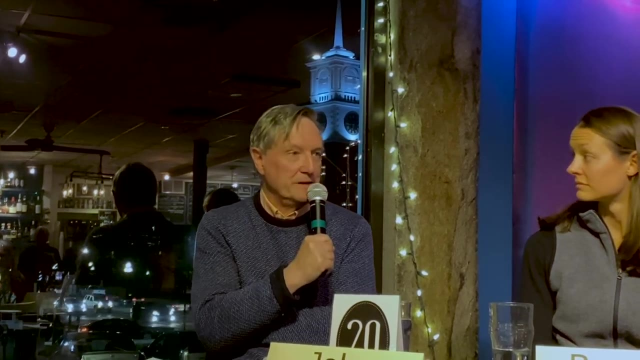 can also be turned into heat energy. it's a process only about 10 years old, so it's another thing, i guess, for municipalities to think about. it's it's another thing you would be asking your people to do, um, but one to kind of put into the bix because it could. 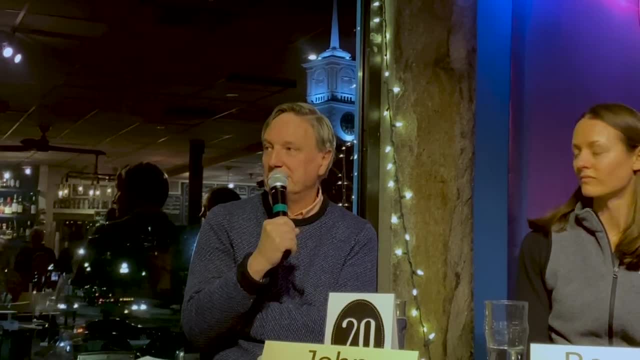 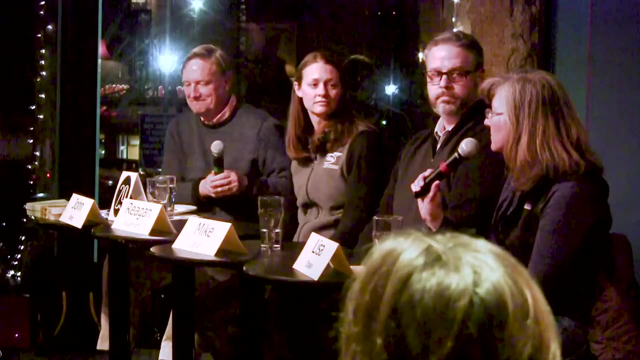 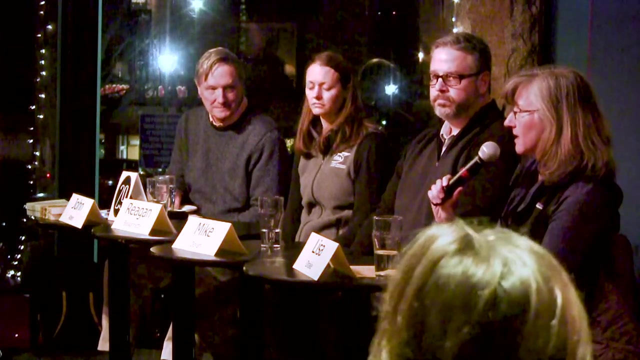 result in a major reduction in the total weight of material. you pay by the ton, right so? and it's wet and it's dense, so you get that out of there. it's, uh, weighs a lot less than plastic. yeah, also on the food waste front. so vermont has a landfill ban with food waste, as does massachusetts, and this is changing dynamics. 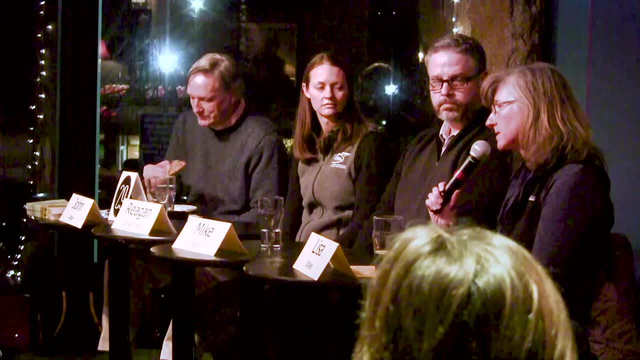 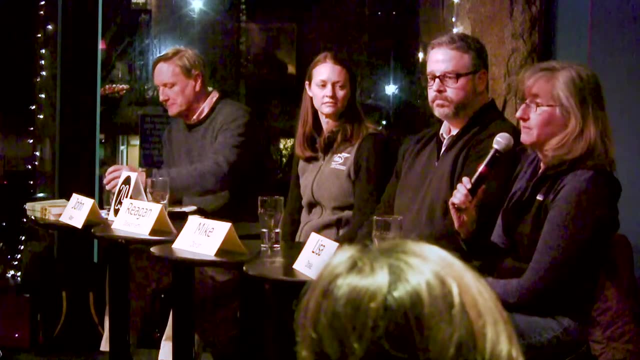 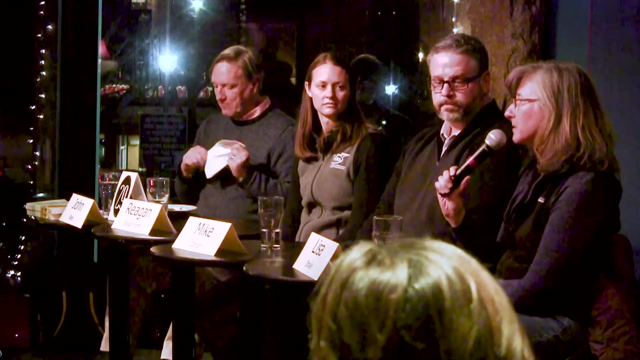 quite a bit, and so one of the things, in addition to composting food waste, is digestion and using anaerobic digestion to create a biogas that can be used as a fuel and um, so there's this is there's a few facilities in massachusetts that have been built over the last few years in order to do that. 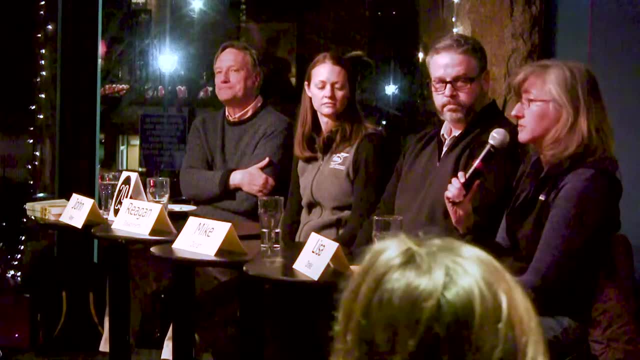 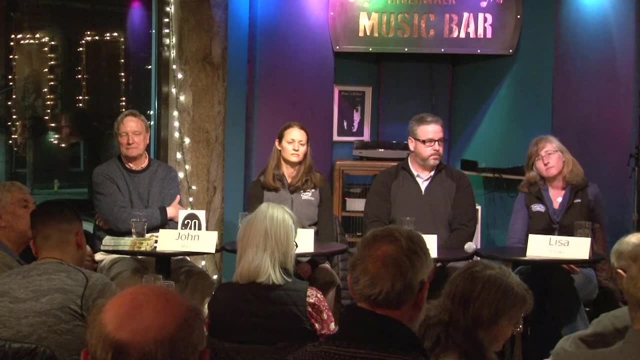 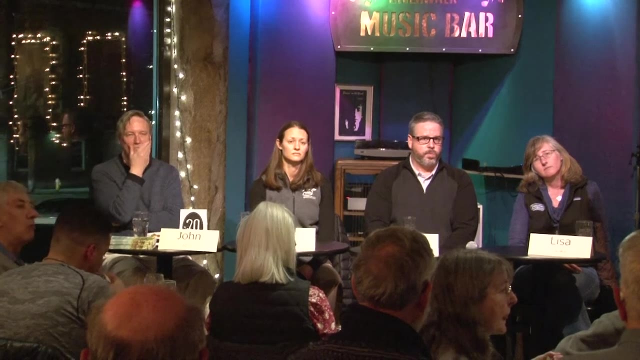 and to create an outlet for the food waste and to have a benefit of essentially creating a renewable energy from it. hi, i know that communities are between single source and um single stream recycling. i happen to live in nashua, which is single stream- but i am more than willing to take the effort and the time. 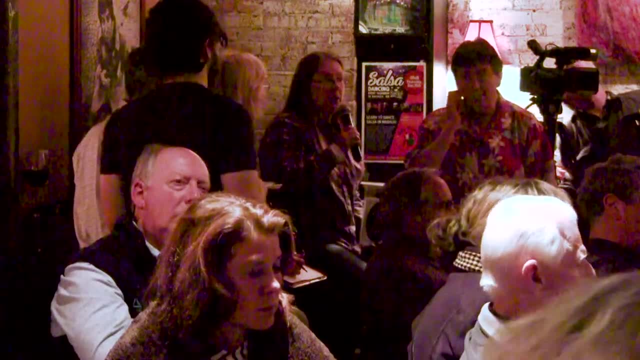 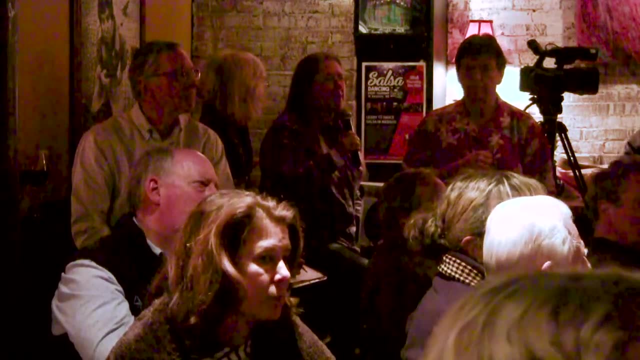 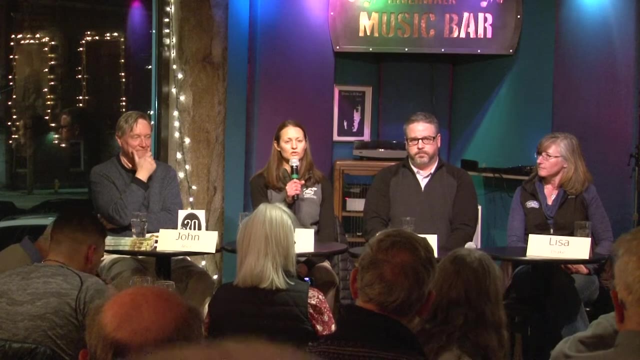 to drive my recyclables sorted well, somewhere else. are there options for those of us that are willing to do that, because i know a lot of places. you have to be a resident of that town to utilize that recycling service. you're correct that most communities you need to be a resident to bring. 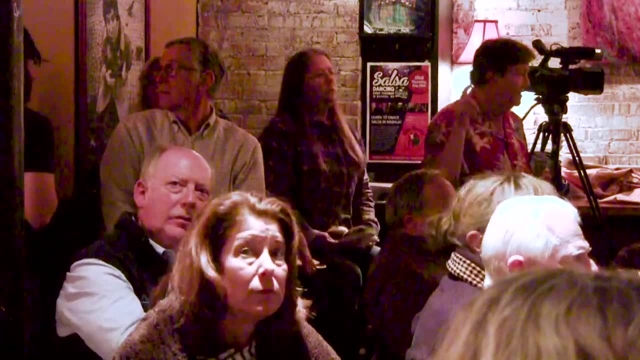 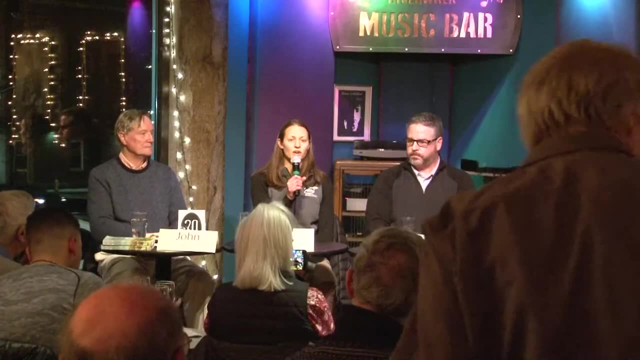 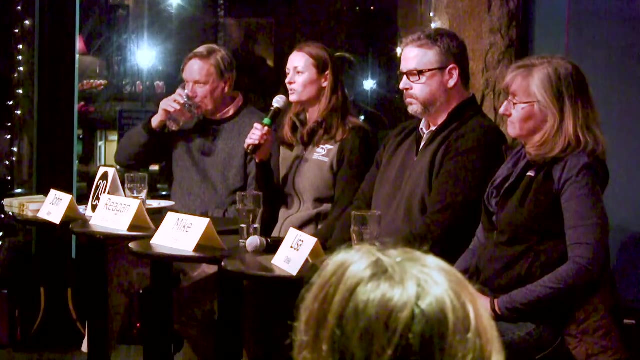 your material. um, i know some people. their community has severely curtailed their recycling, for example, and so they take it to a community where they work that is recycling, or maybe they bring it to a friend whose community is recycling. those are not feasible workarounds for most people. 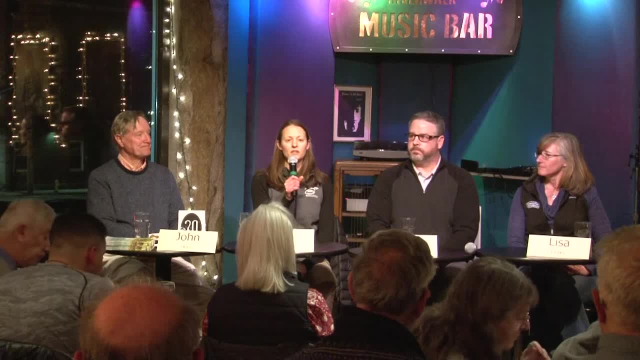 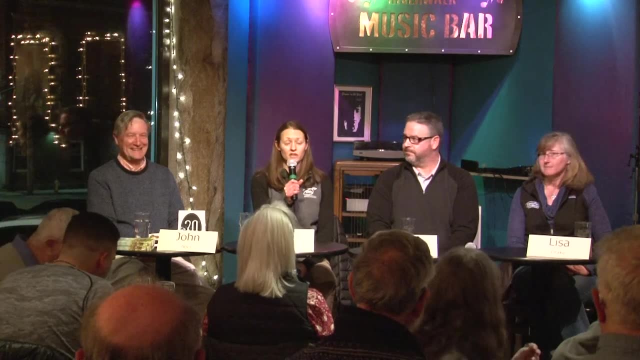 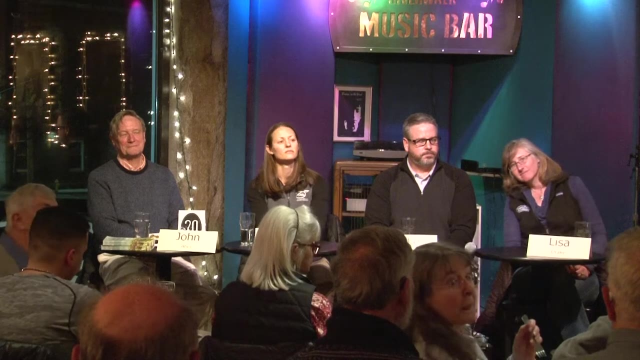 i believe that the city of lebanon's facility will take recyclables from anywhere, but you're having to drive your recyclables all the way to lebanon, so you got to take into account that factor as well. i understand that recycling is is so difficult and we have so much of it, so my question is about the other half of the equation. 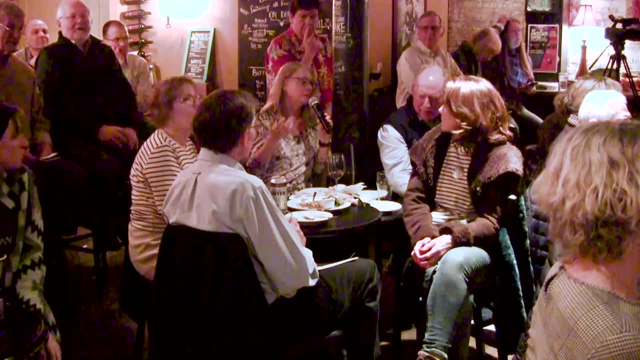 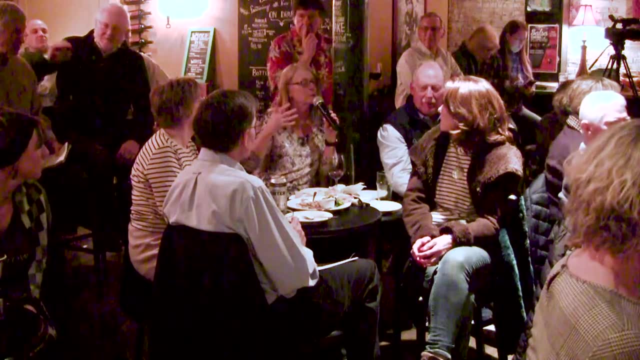 which is just simply reducing what we have, and i know um in new hampshire, for example, supposedly, but i haven't been able to find the details. there's a lot of work to be done to reduce the amount of trash that we have, and i'm just wondering if there's a bill out to just simply 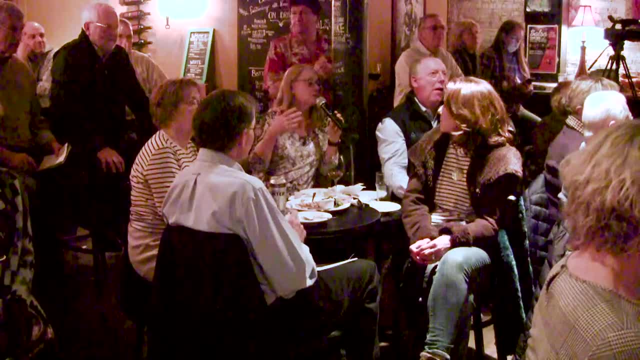 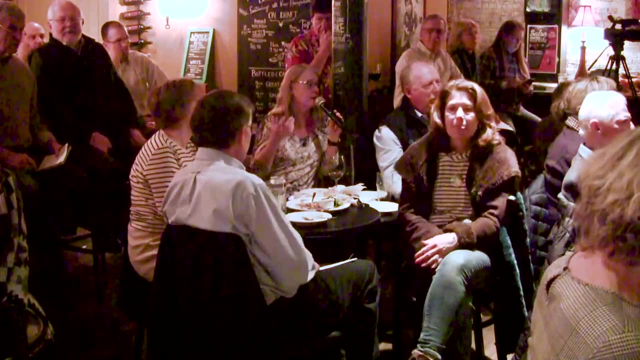 help us prohibit plastic bags from being used, and i'm just wondering if there are. you know, i was kind of curious as to what's happening with that- and if there are other things that we can do that just simply reduce the amount of trash that we have. well, i mean, there's certainly many things. 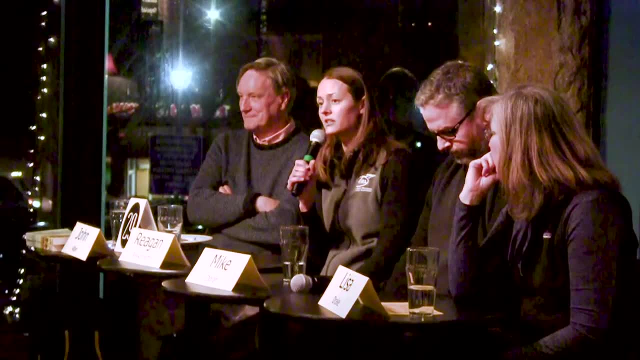 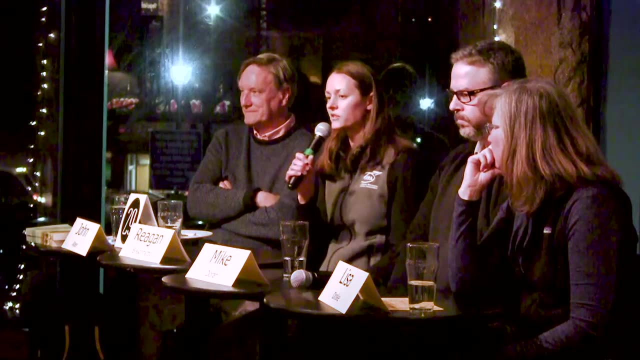 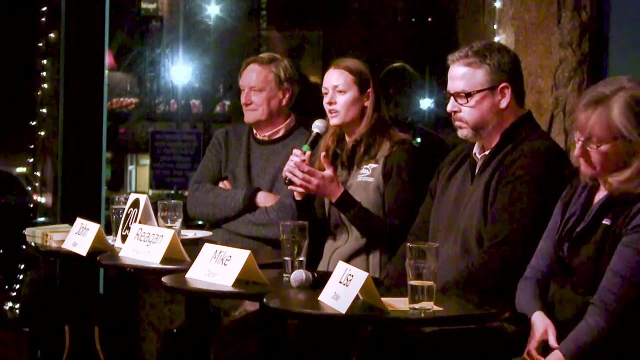 that individuals, that we as individuals- can do to reduce our waste. if you haven't heard the concept of zero waste, there's a lot of information on the internet about people who try to adopt zero waste practices. for example, um, you know, always bringing your stainless steel container with you and never buying a you know bottled water, just so you avoid that bottled water. 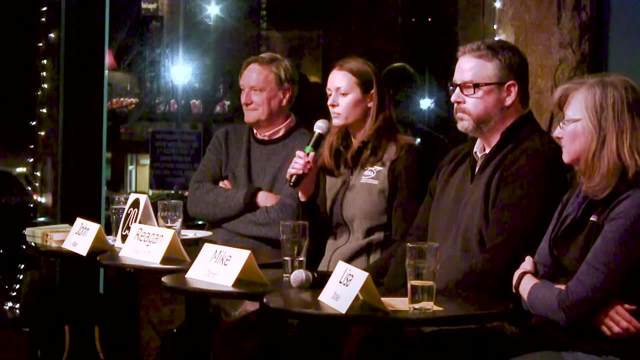 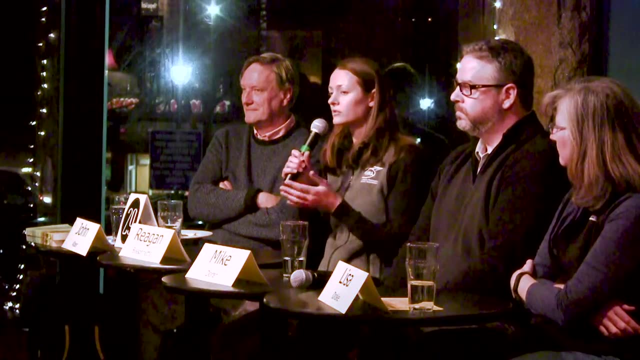 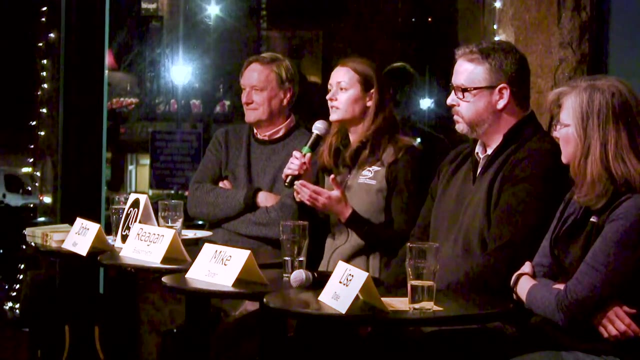 on a broader policy level, there is quite a bit of proposed legislation coming out right now that came out of a study committee that held hearings in the fall that was referred to earlier. so there was a. it was called hb 617, it was recycling and solid waste study committee, and their job was 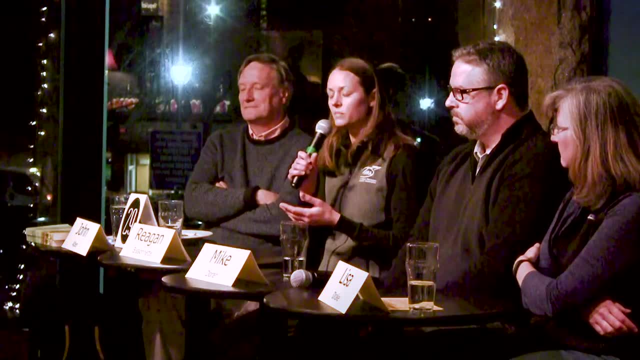 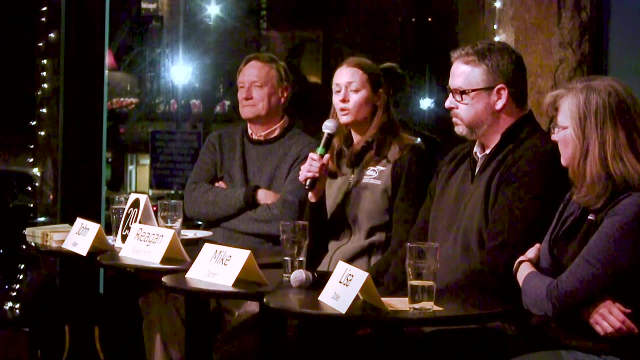 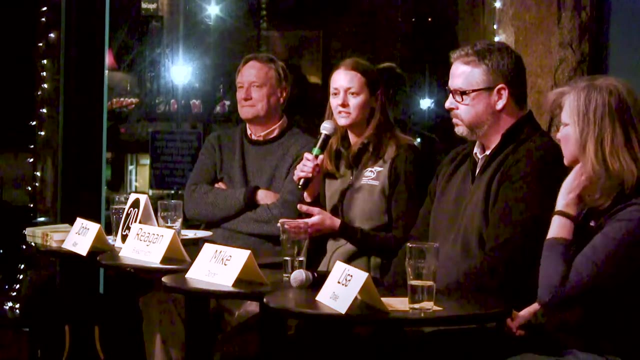 to look at the challenges that municipalities are facing with managing their recycling programs right now and then make recommendations for how the state can help, and most study committees. they might hold a handful of hearings and issue a report that's a handful of pages. this committee held an unprecedented 14 hearings and they issued a nearly 30-page report. it's a wonderful resource. 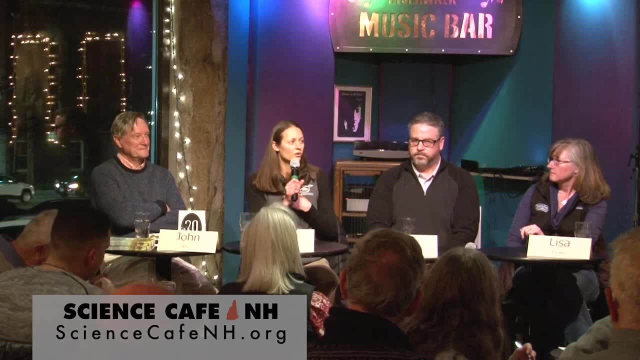 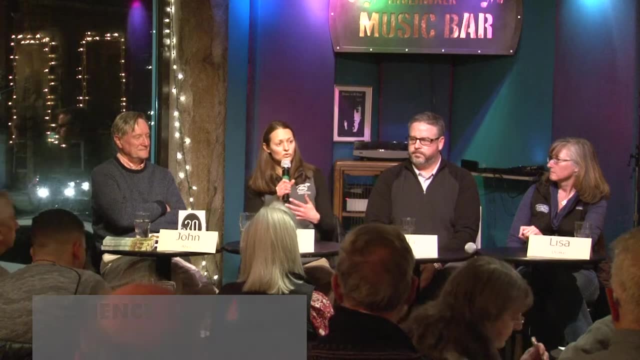 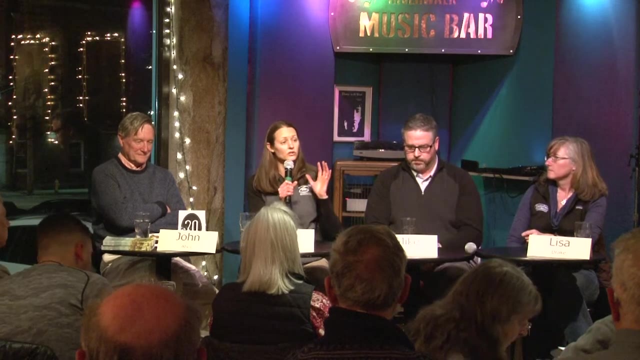 if you want to take a look at that, if you go to the home page of our website- it's wwwnrranet- we have links to some of that information on our home page, and now there are more than a half dozen bills that were directly coming out of the recommendations of that committee. so one of 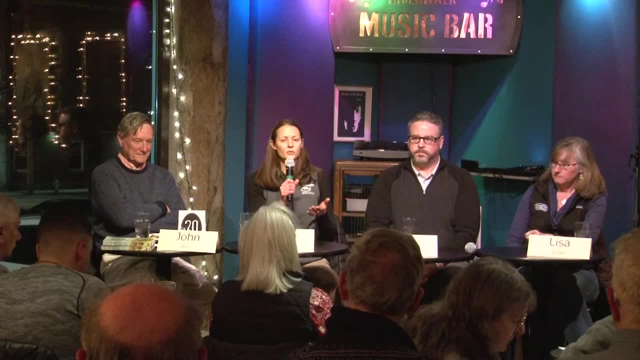 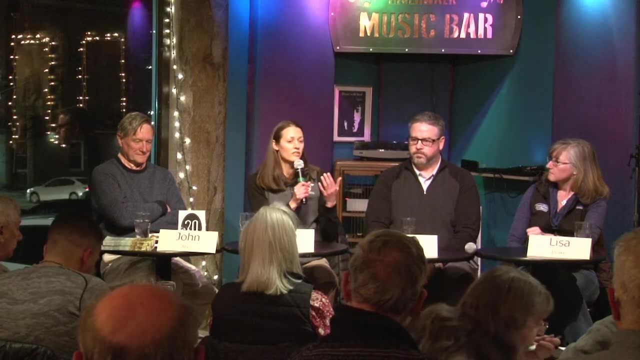 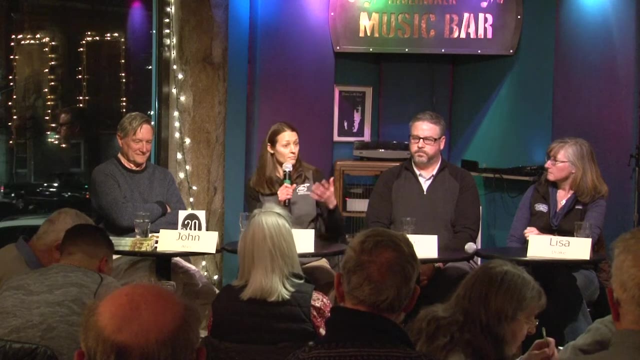 them, for example, is to evaluate the state's solid waste reduction goal. so we actually had a goal, step by statute, that by the year 2000 we were going to divert 40 percent of our waste either through recycling or composting or some other means. we don't know if we ever achieved that goal. 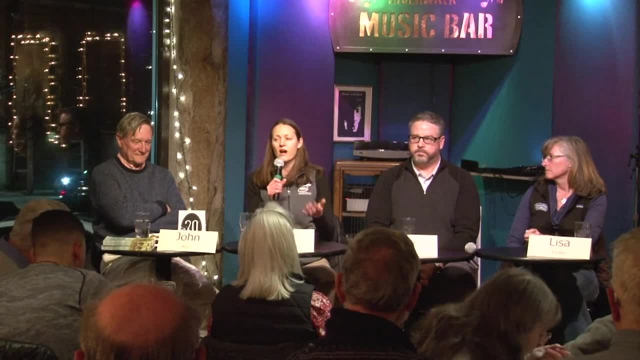 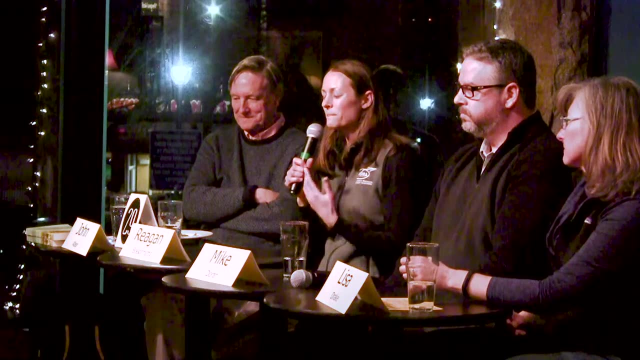 because the department of environmental services wasn't empowered to collect the data they needed to know if that diversion was happening. so one of the bills coming out of this study committee that just had a hearing recently would be to set a new goal for the state to reduce. 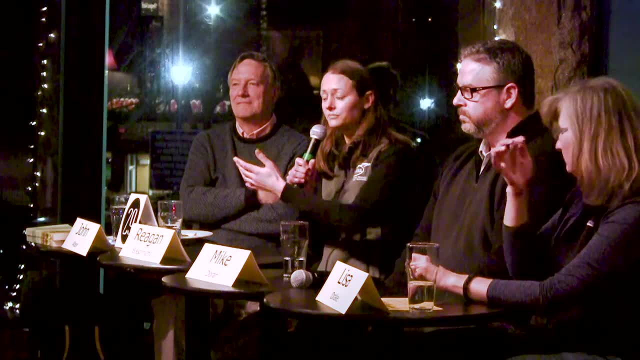 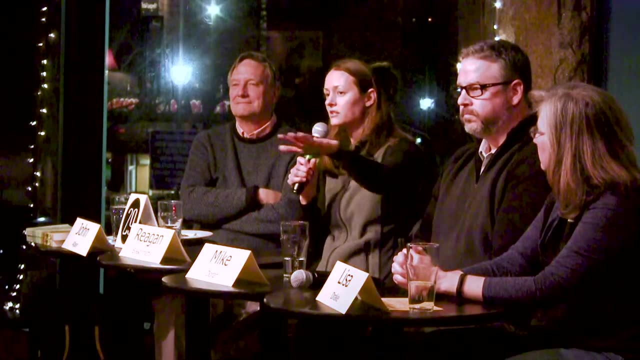 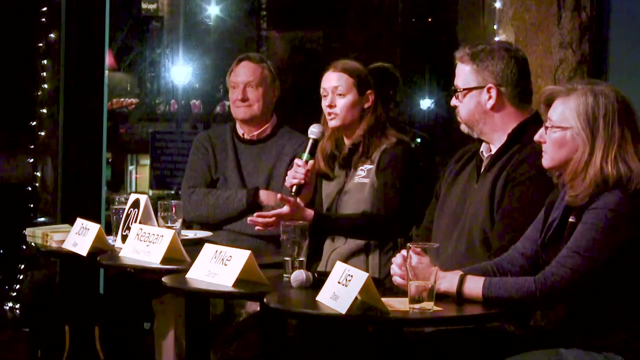 waste by 25 by a certain date, and that would be measured simply by taking how much trash was produced in new hampshire at 2018, starting at that level, and then we're going to try and reduce it by 25, and then, of course, the bigger question is: how do you actually achieve that? so there's another. 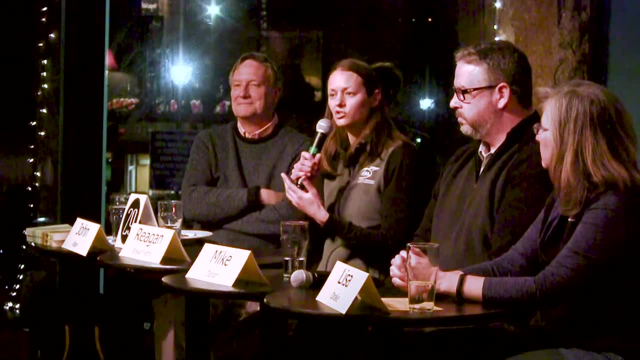 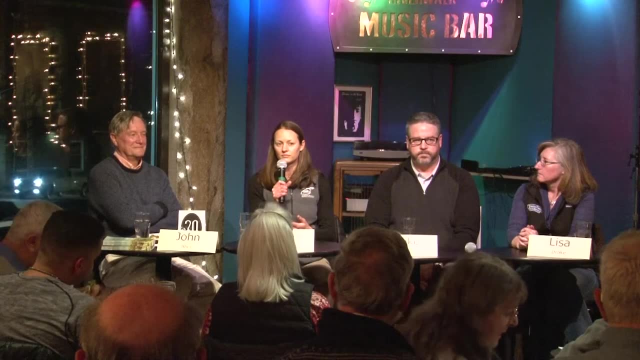 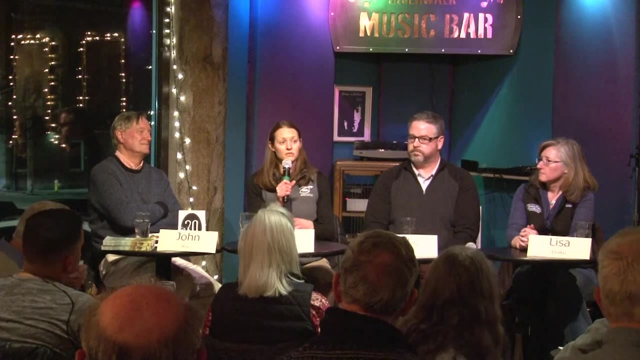 bill that came out, and this bill proposes to put a 1.50 surcharge on all waste disposed of in new hampshire, because it just so happens that in new hampshire half of the waste that's disposed in our state is coming from out of state and much of that is coming from massachusetts, because other states are restricting their landfills, restricting their incinerators, and so more and more waste is coming to us. so this bill would essentially charge a dollar fifty per ton on all waste disposed of in new hampshire, and then it would propose to rebate back to municipalities in new hampshire their dollar. 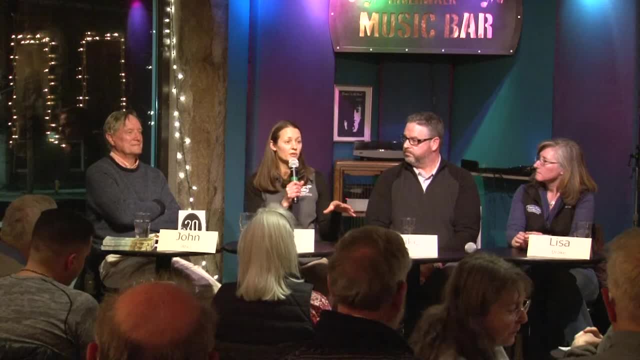 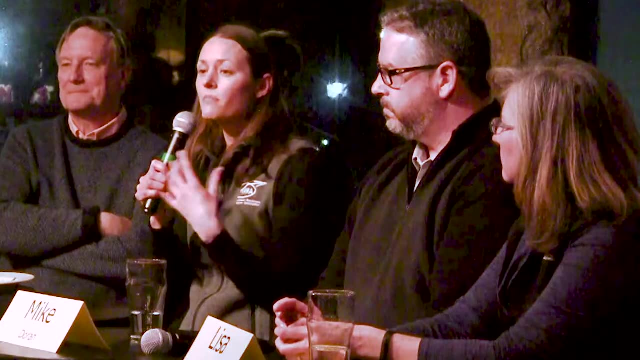 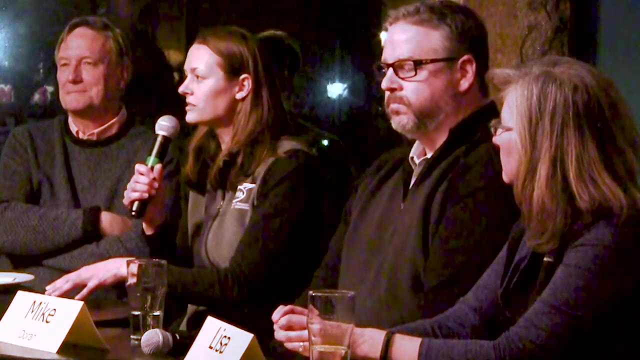 50. made whole, and then the remaining funds, which are coming from out-of-state waste and then also from waste generated by businesses in new hampshire or other entities. that money would be used to fund a new technical assistance and education group at the department of environmental services. 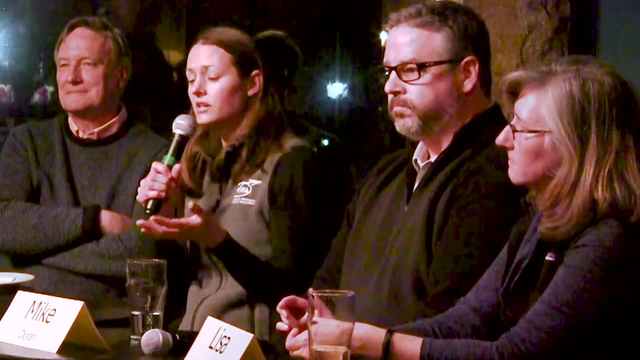 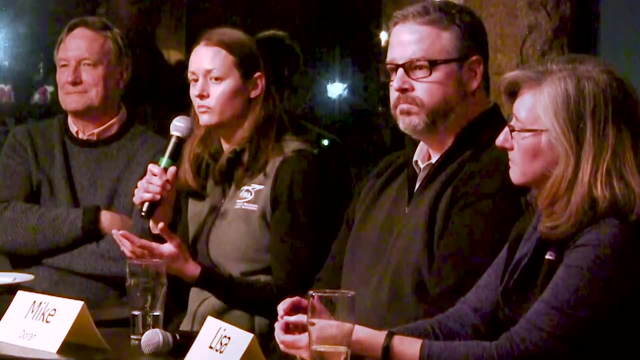 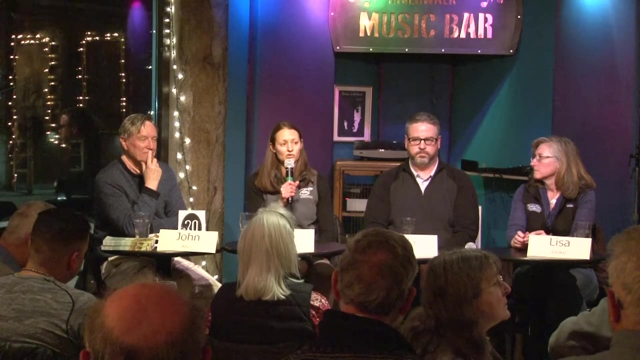 who would be able to assist communities with actually reducing their waste. and then also it would fund a grant program that municipalities and businesses in new hampshire would have access to for again working on reducing their waste, whether it's through recycling or composting or other measures. 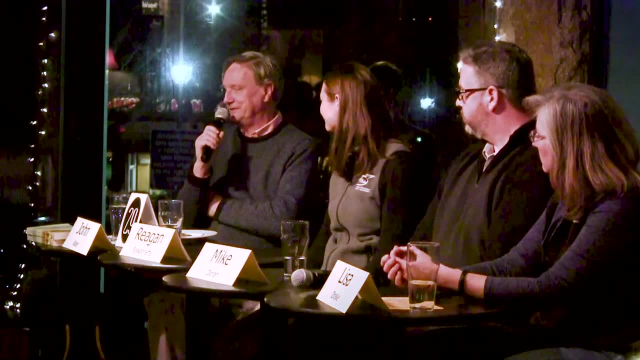 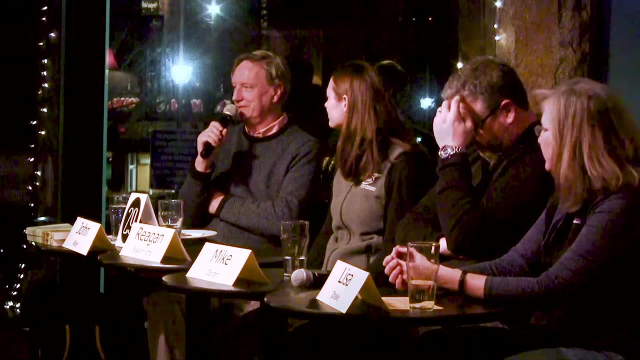 so i'm really glad i'm here. i'm enjoying this discussion a lot. ironically, i almost didn't get here because i got trapped behind a waste truck- garbage truck- that went off the road on 101 just east of manchester and i sat there. fortunately, i left 45 minutes extra time, so i was here on time. 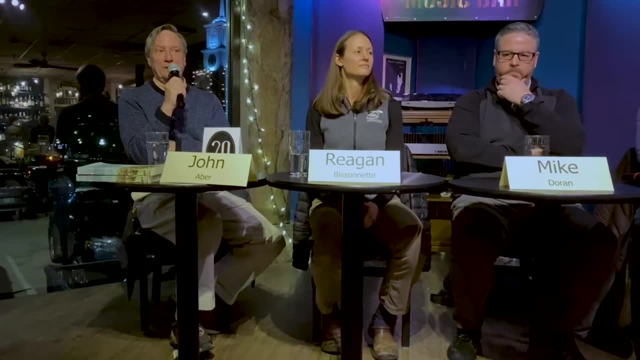 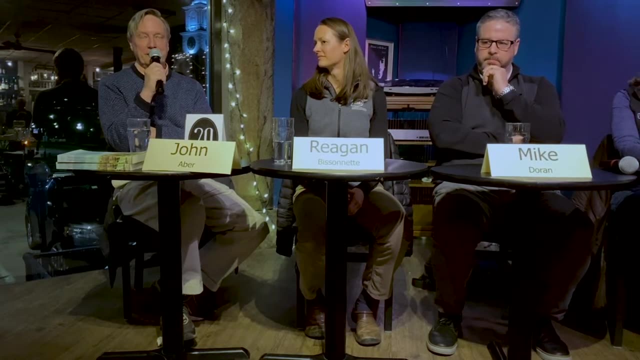 just thought that's a little bit of irony. but in terms of reducing waste streams, uh unh has some interesting examples, because the things that are controlled centrally a lot of the time are like the food, waste things from the agricultural farms and stuff. policies can be set up and 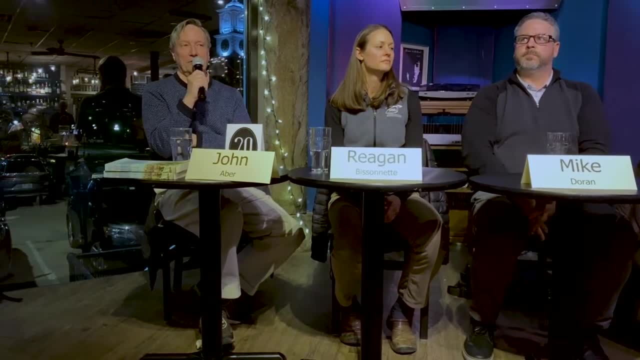 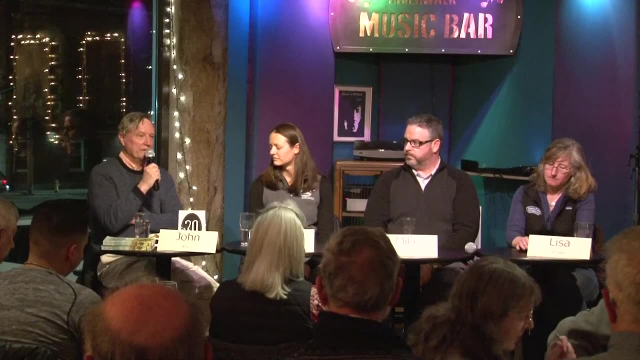 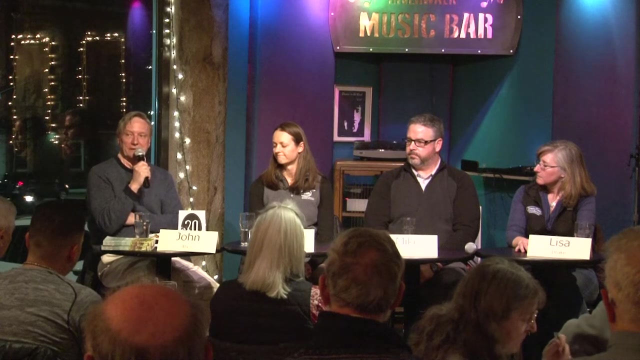 processes can be done fairly easily because it's a top-down thing. unh has not been successful in recycling except in these controlled facilities like the football stadium, where everything that comes in is compostable to get students to recycle. you know it's personal behavior and there's a very 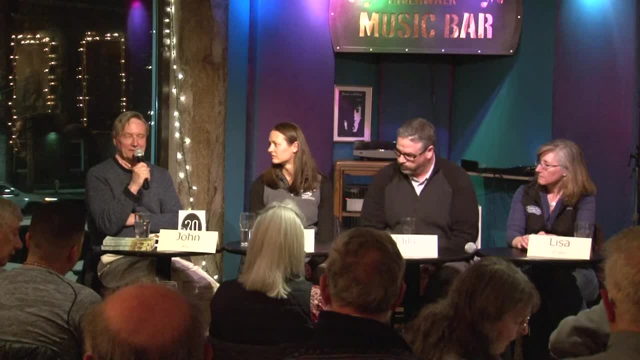 strong environmental ethic on campus. but you need the bins. you know i say it's bins in behaviors. you know you need the cash. i have three לו national regulations. you know vinegar is one. this is a national- to have the right infrastructure to make it easy and educational, to make sure. 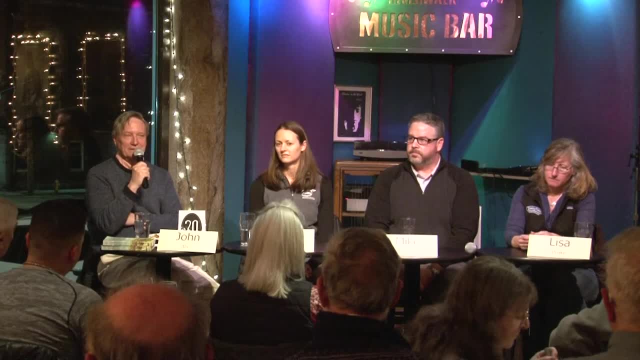 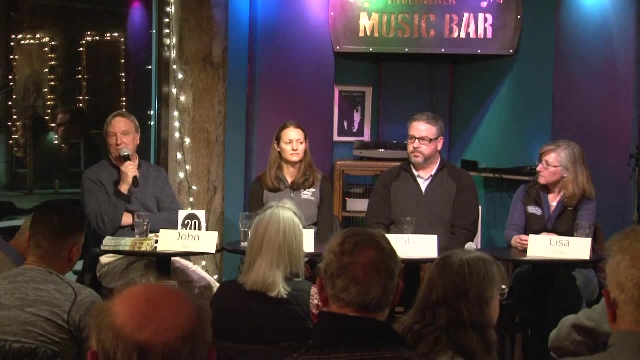 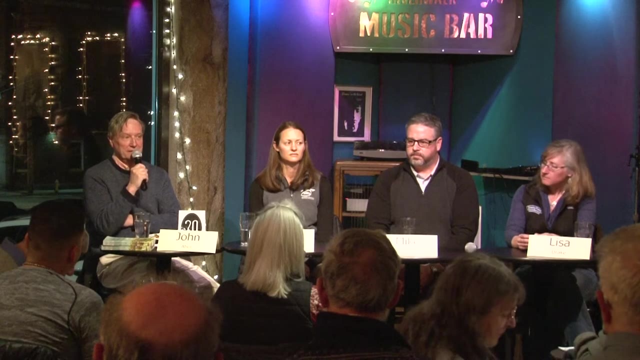 stuff goes in the right bins, you know, and then you're teaching kids and I think it's probably the same thing in municipalities. you know there are certainly financial incentives. Durham is considering pay per throw, which Dover does lots of heat around that, as you might imagine, but that in some cases has. 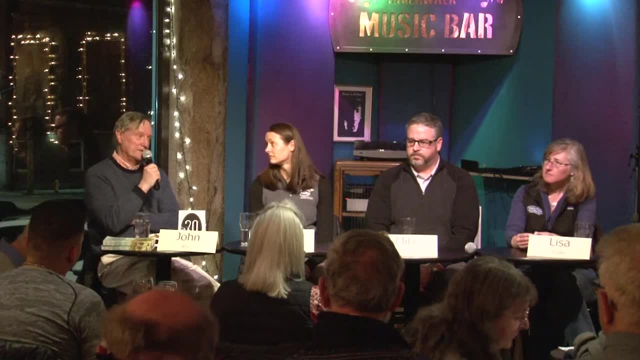 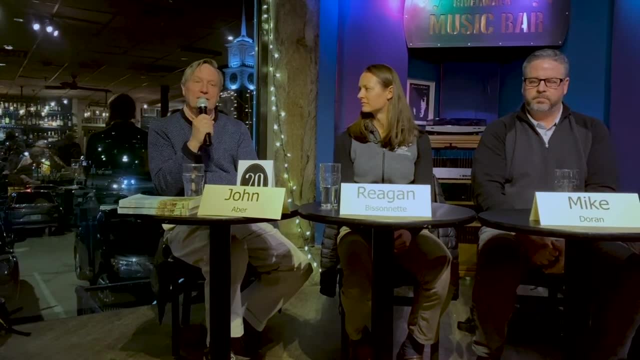 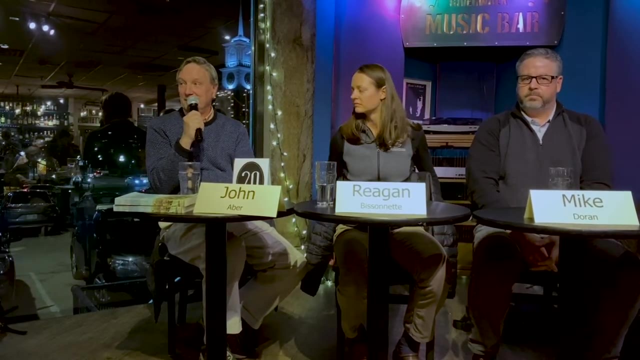 reduced the amount of waste going to landfills. whether or not it's actually going out on the back 40 instead might be a question, but the financial incentives or any other thing, because it's really it's it's, it is individual behaviors, I think, that are gonna help solve that problem and that's education. 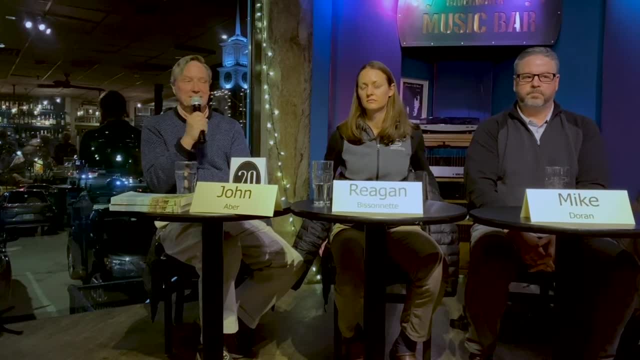 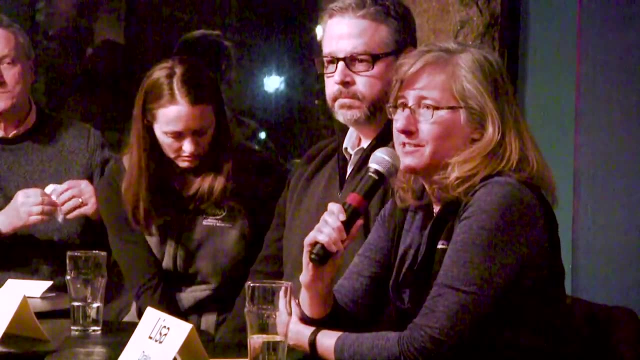 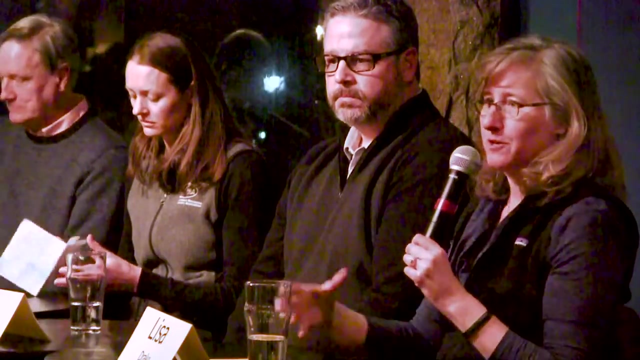 that's culture, that's all kinds of things, and maybe financial incentives like paper throw as a manufacturer there. you know we, we know that the most efficient package that we sell is what we call our tubs. you know, it's like a quartz of yogurt and two pounds of yogurt in one package. so from how much packaging? 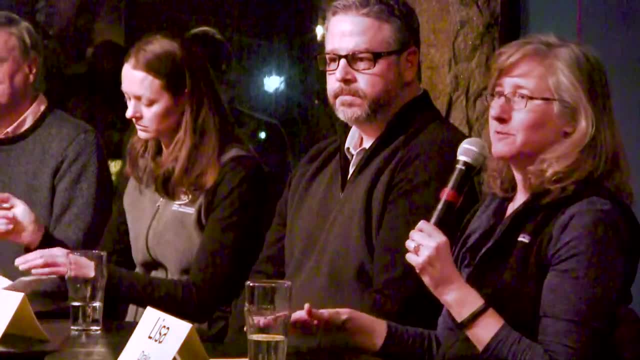 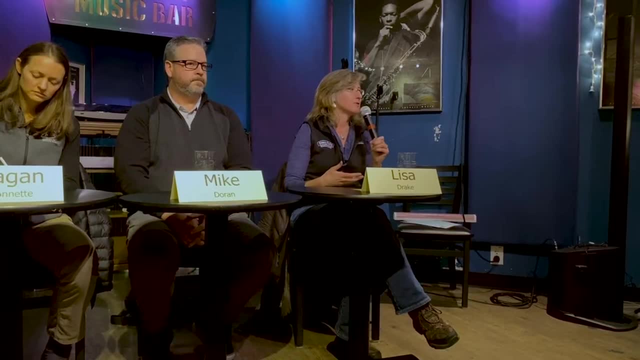 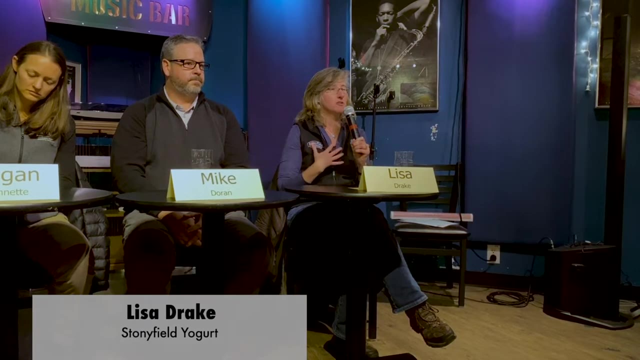 do we use per serving of yogurt. that's the most efficient package. so that's you're trying to reduce your use of materials and buying the food at the grocery store thinking bigger packages generally are are better. but the trend and then what we struggle with to some degree is Americans like convenience and so there's a lot of demand for smaller packages, especially when it comes to our kids and our baby products. of course, they're eating less in one serving as it is, but these things that you can take to go are really popular, and so that takes all kinds of. 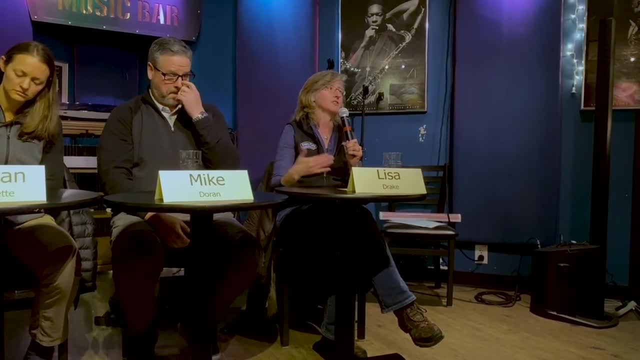 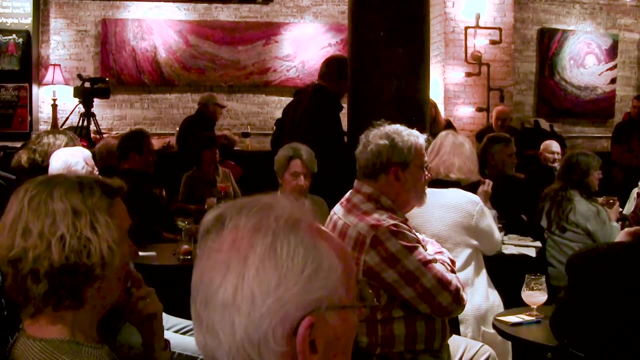 different materials and formats and generally are more packaging intensive. years ago I realized we had a lot of food waste and I started composting but it didn't work out. I used in my garden but still didn't work out. but recently I heard something else of interest. they said there is a 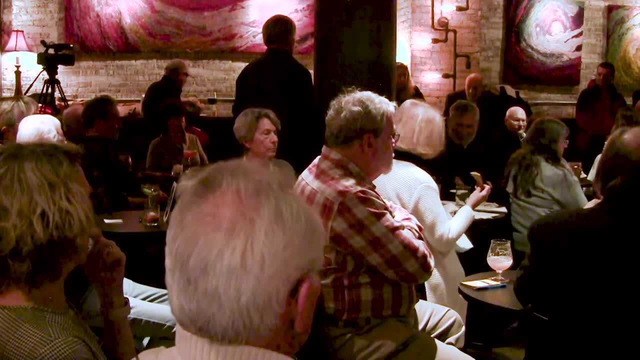 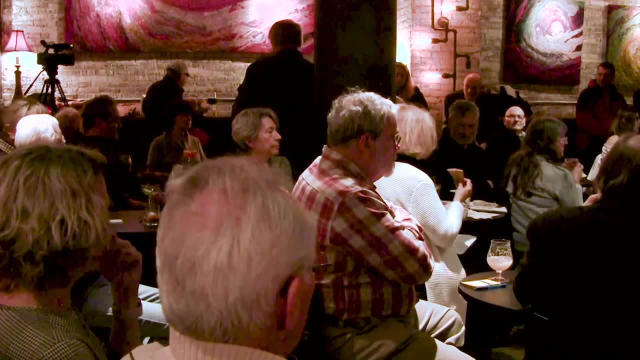 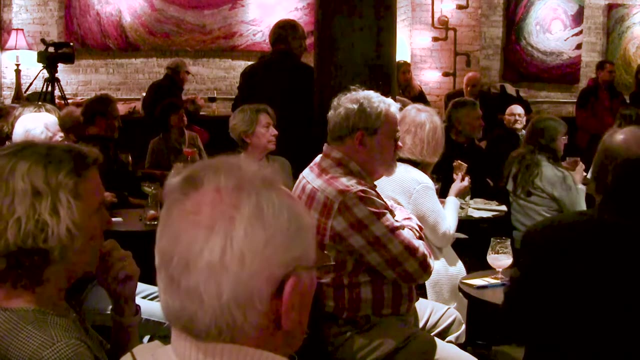 service where you pay a monthly fee, take all your compost, put it in a bucket or some kind of container and then they will compost it for you and then the result in compost that could be used in your garden you can pick up for free in the summer. does Nashua have any kind of a arrangement like that or any other? 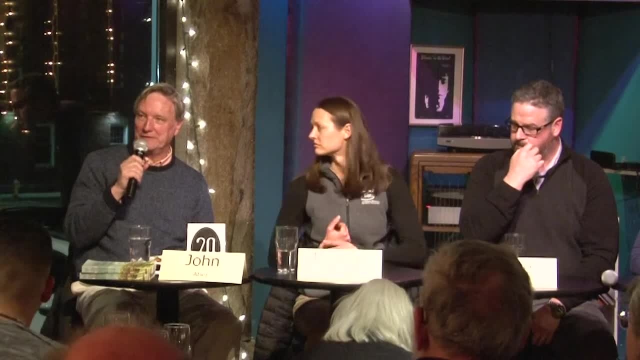 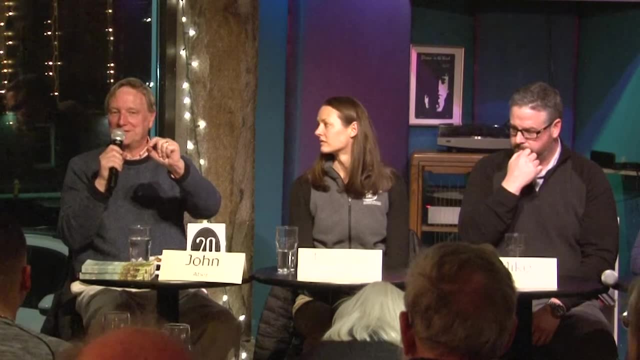 facilities. up our way in Durham there's a this mr Fox that actually had to locate in Maine because the New Hampshire restrictions on food waste being composted were such that it would. he couldn't do it in New Hampshire. it was really interesting story. a bunch of students got together, went through their 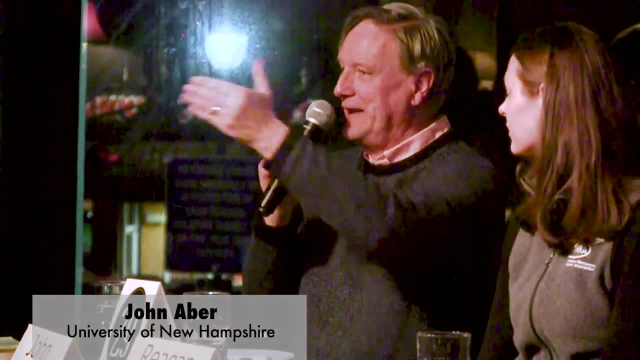 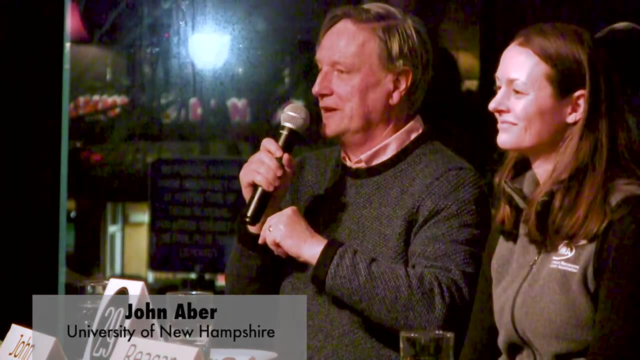 legislators got the bill changed in New Hampshire so now he actually could move to New Hampshire and operate. but buddy, he's already in Maine. but I saw his truck go through the neighborhood just this morning and he was picking up compost from various places. sounds like the same kind of process and I suppose will be. 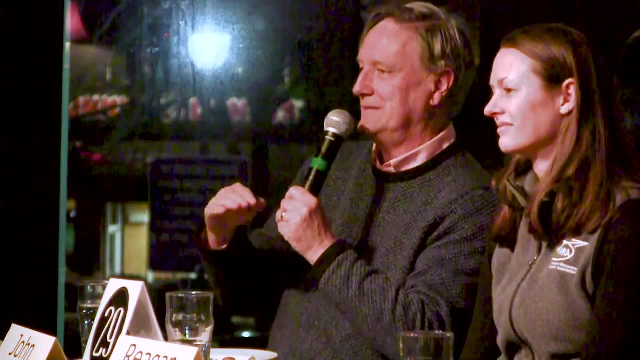 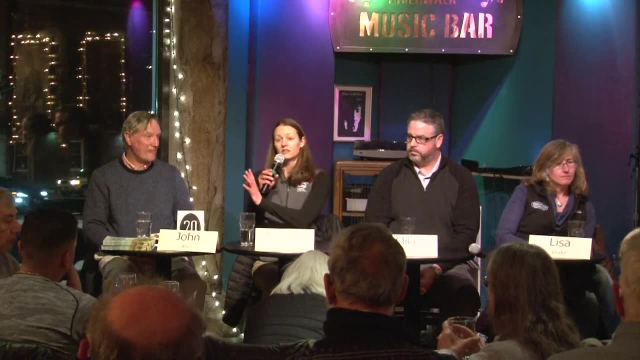 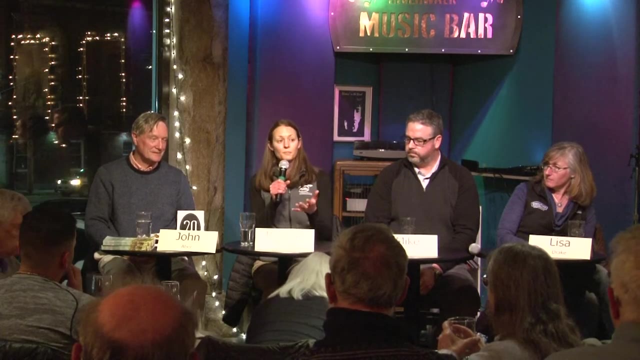 returning probably about 40% of that weight back as compost, because the rest of it disappears. a bit of a sad story, which is that in 2015, these UNH students did succeed in having a bill passed in New Hampshire that directed the Department of Environmental Services to update their composting regulations. they haven't been. 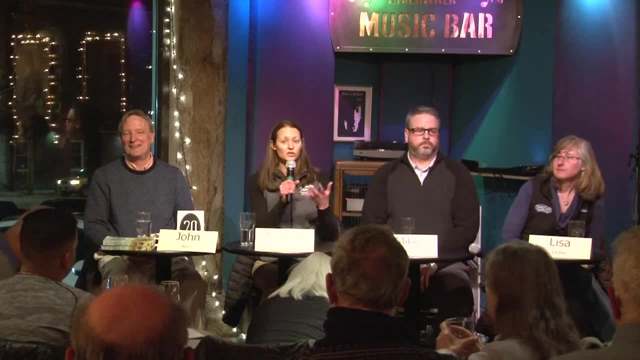 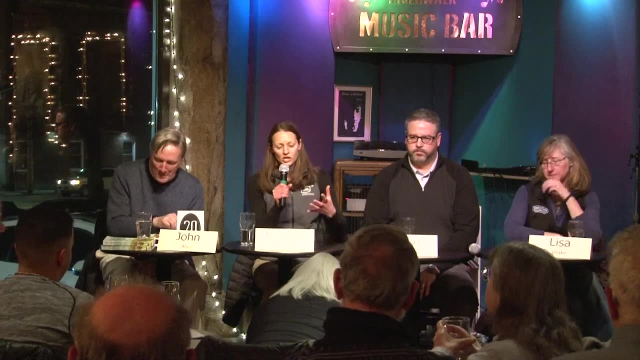 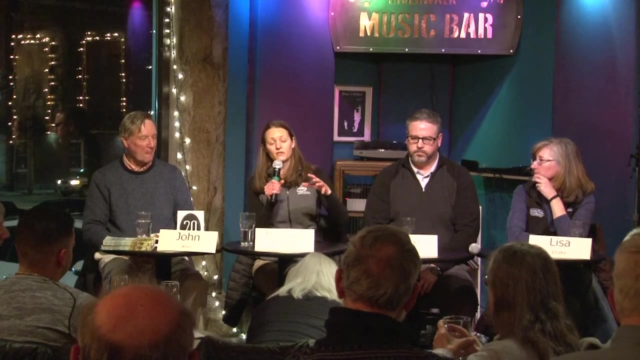 able to do that yet because the department is so severely understaffed and under-resourced. so they've- they've held stakeholder group meetings, they've worked on, I think, drafts of updating their composting regulations, but it actually hasn't happened, and one of the proposed bills coming out of the study committee from the fall is: 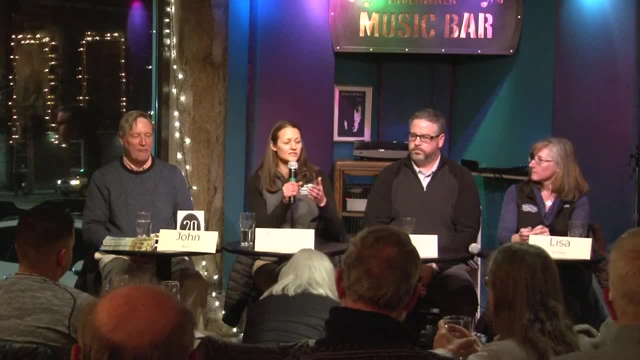 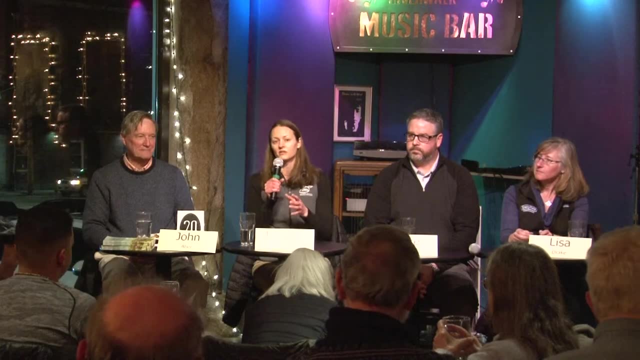 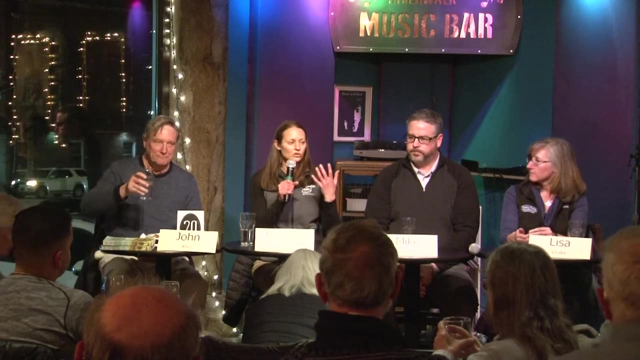 to direct the Department of Environmental Services that by a certain date they must update the composting regulations and it's not that you can't the issues with meat and dairy. so the way the regulations are in New Hampshire if you want to compost to meet or dairy, either at a commercial or municipal, 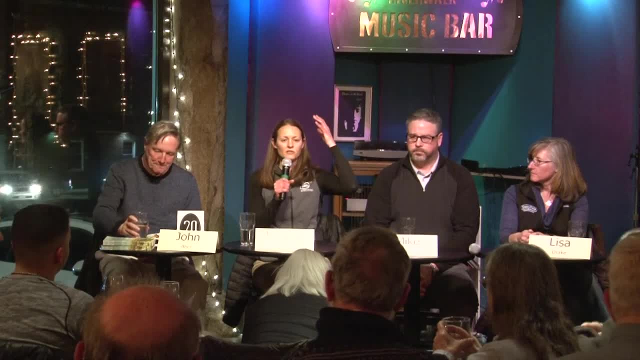 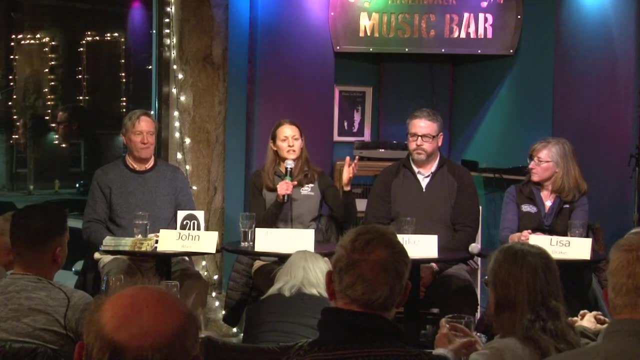 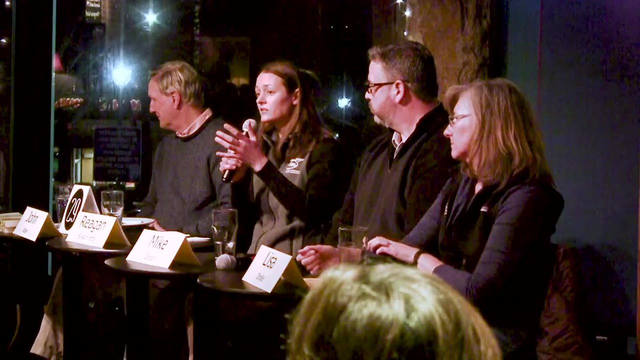 level, you need to have a certain type of permit that requires a very extensive review and approval process through the Department of Environmental Services. so right now, I think we have only six companies or entities in New Hampshire that are permitted to compost food waste, and only one of them is allowed to. 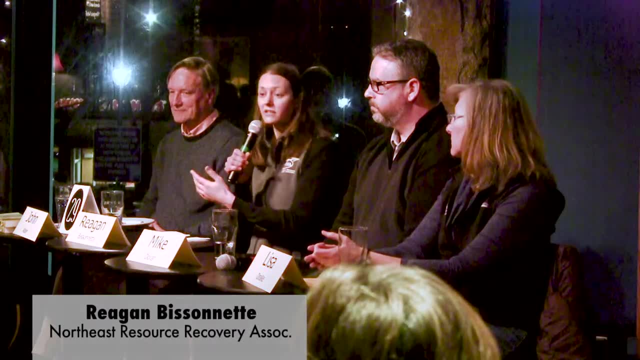 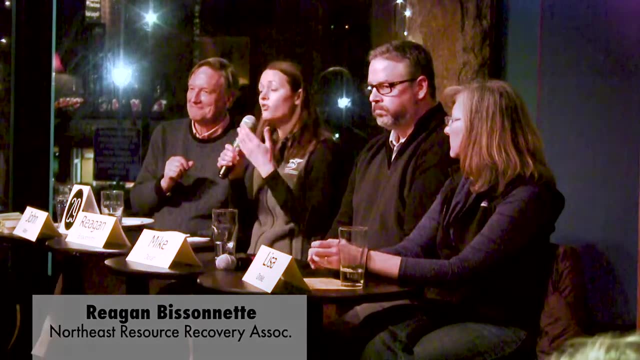 compost meat and dairy. and that's Star Island, because they got a special exception, because they didn't want to have to take all their waste off-site. but hopefully that legislation, or hopefully those regulations, will get updated soon so that it is more accessible for communities that have a 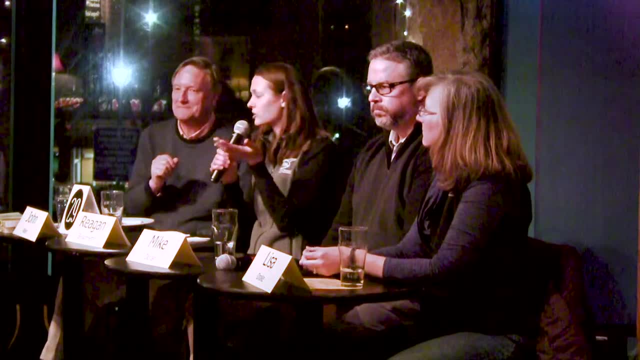 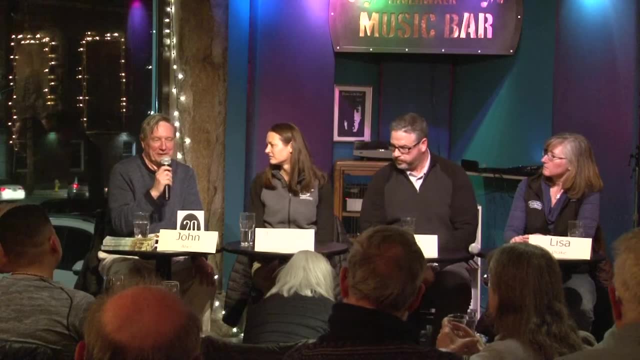 not that super extensive permit, but a different version, a different solid waste permit that they could more easily compost meat and dairy with appropriate guidance data coded. that the students- one of my graduate students was one of the people involved in that- and they sold it to the legislator and the 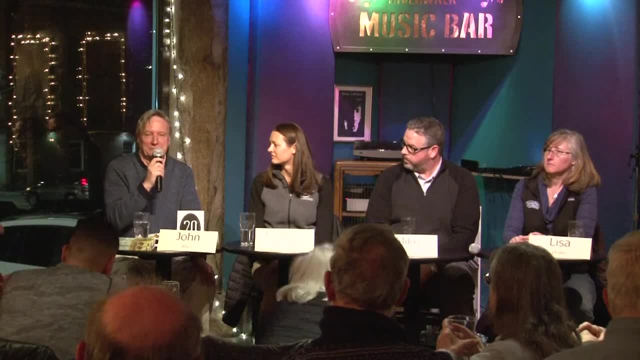 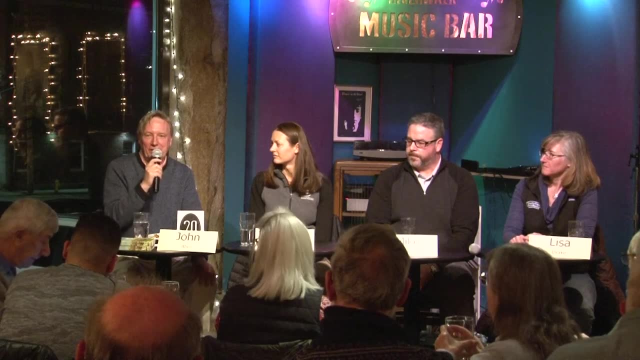 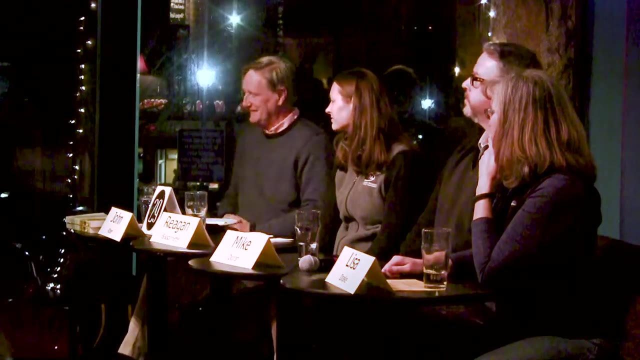 legislature as reducing inhibitions on on Enterprise, that there were too many regulations in place and it was freeing up innovative entrepreneurs to be able to do this new thing in New Hampshire, which I thought was very savvy of them. quick question for Mike: if we're a non-profit, are we able to try to? 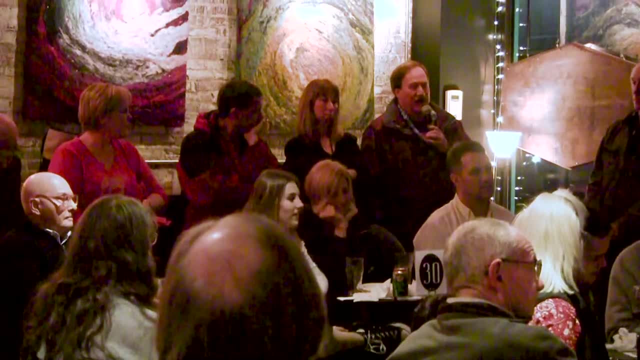 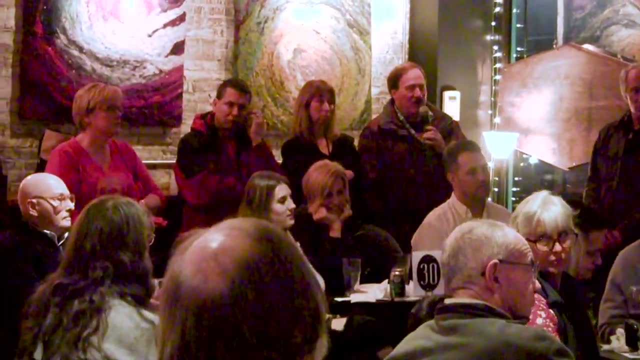 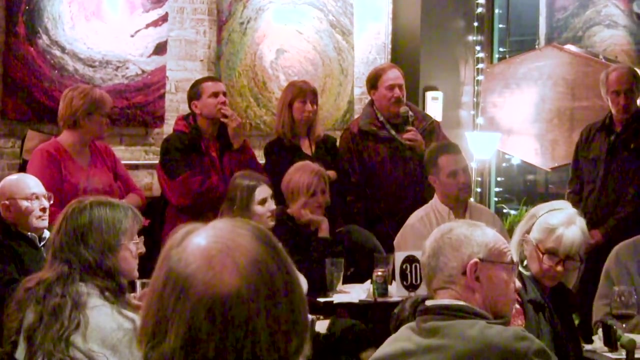 collect or have monthly or quarterly- like electronics- people to drop off. is there problems with privacy getting you the the items? are there some different ways we can try to Channel? maybe raise a little bit of money on the side as a non-profit, but just to try to get you some things to work on over there sure. 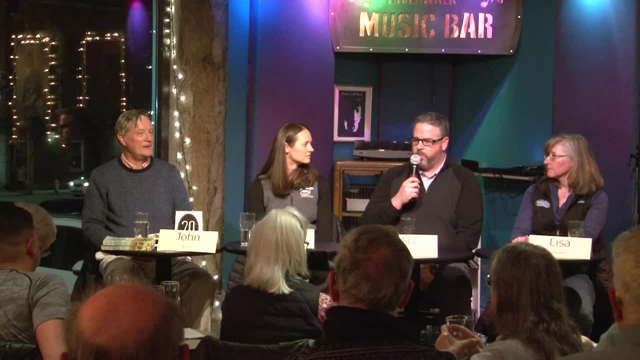 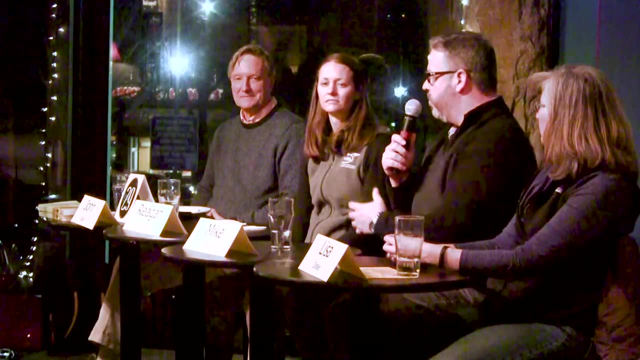 so in that case, what we would do? we, we work with groups that we do, like a recycling drive. so let's say you, you know, we would partner with a group and they set up in a high school or a church or parking lot and then promote the event and we would provide the you know. 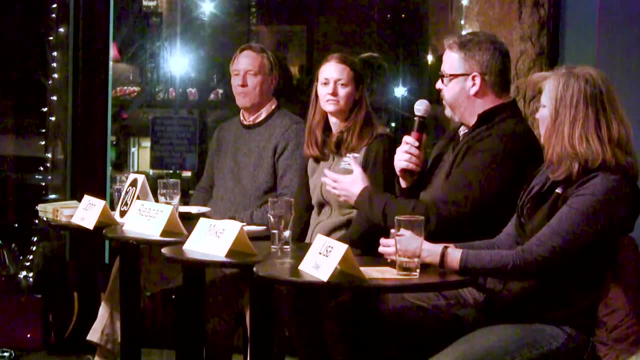 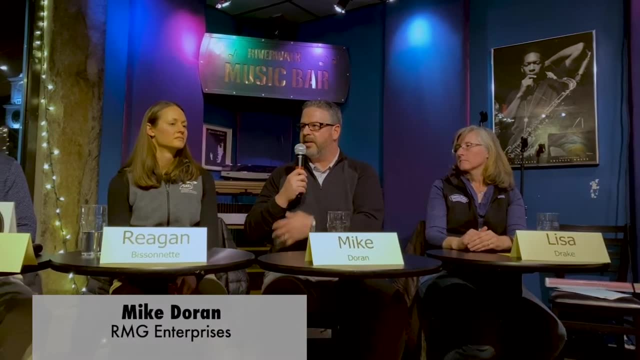 the trucks and the supplies to collect the material, and work out a, an arrangement with you that we basically like giving you a wholesale rate on the, on the, on the processing and collection of the material, and then you can work with your- you know your customers and, and and try and raise a little bit more. 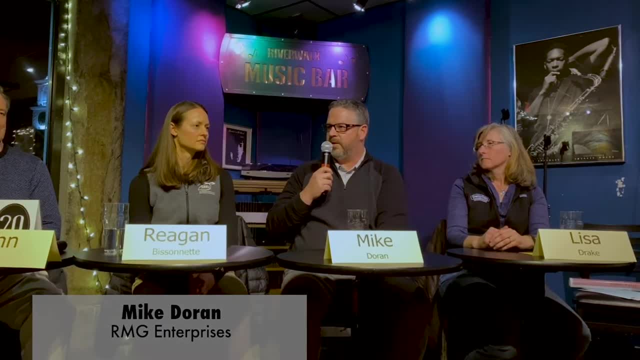 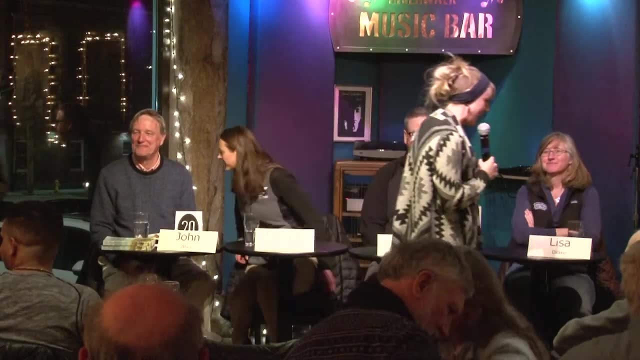 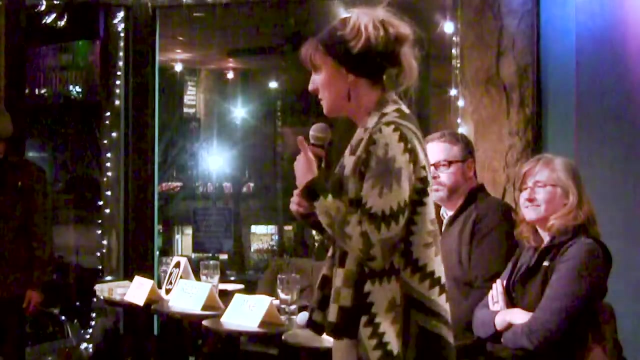 money. but yeah, come speak to me and we can discuss how how that works. that is definitely a possibility. good evening everybody. thank you science cafe for having me. my name is Stephanie Obear and I am the director of program development for grown ashawa, so let me tell you a little story about waste food waste, so 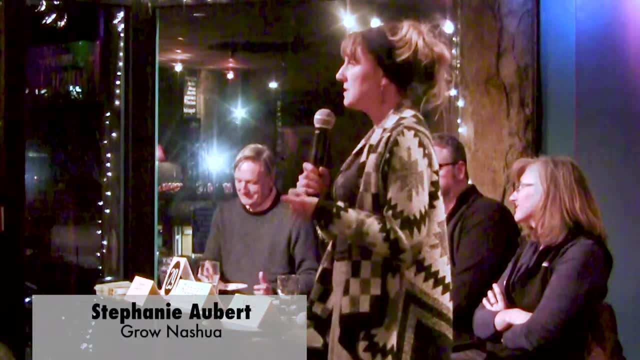 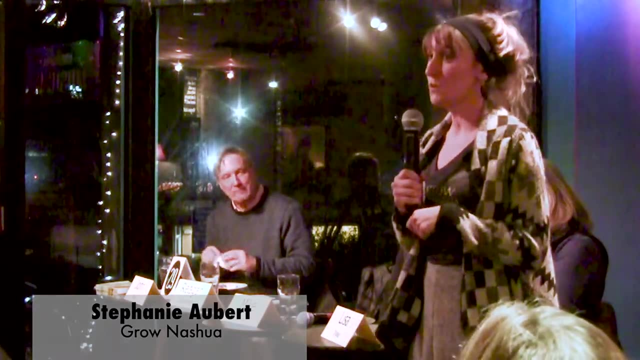 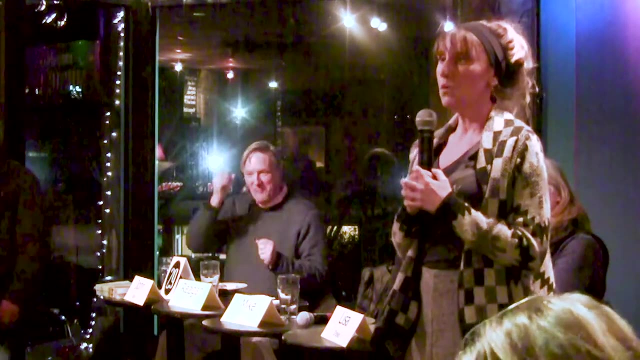 grown. ashawa has several programs. we've got our growing spaces program. we are going to build our seventh community garden this year, 2020. we have a growing education program and that serves the elementary schools in nashua. we teach about growing food and we have gardens at several. 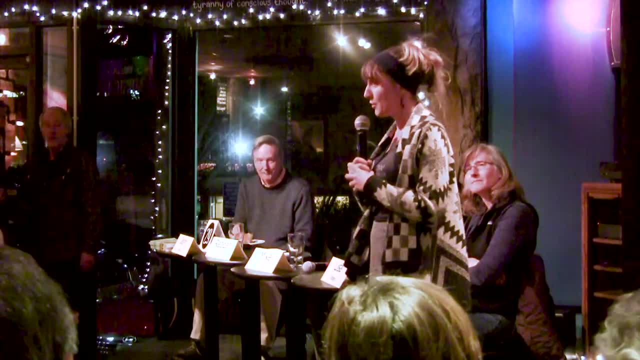 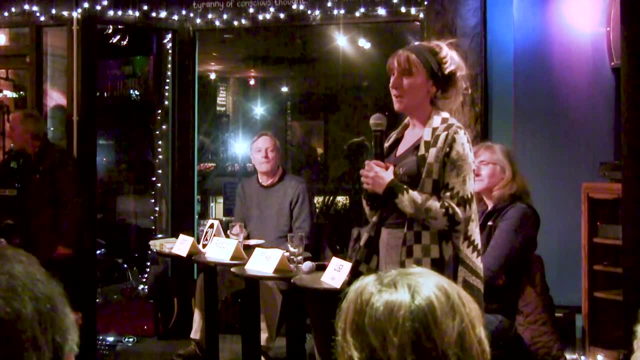 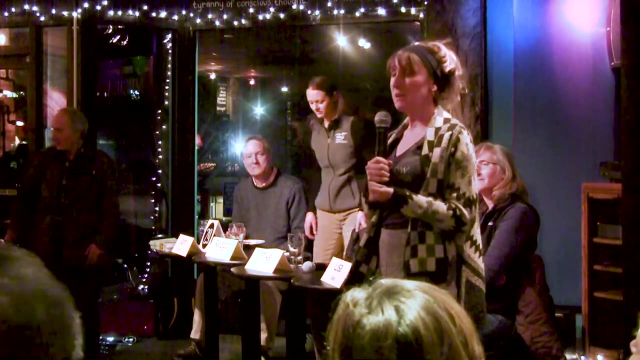 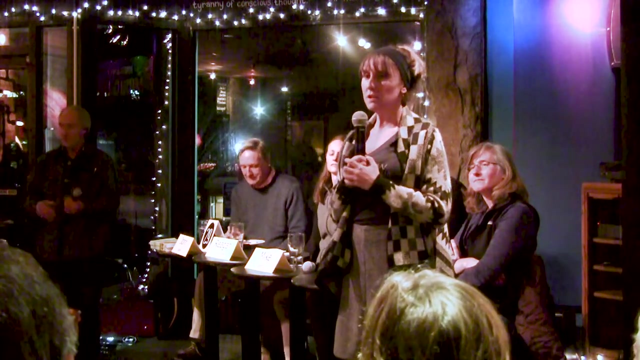 of those schools. we also have a curbside compost program began about a year and a half ago in my in grow nashua as executive director's backyard. he decided it would be a really neat fundraiser to a be able to hire a local fellow and provide a fair wage job but also to collect food waste from. 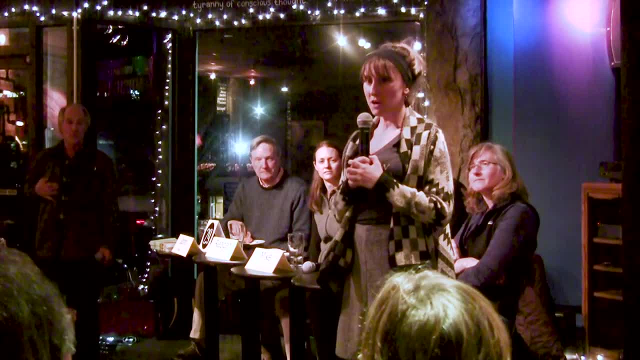 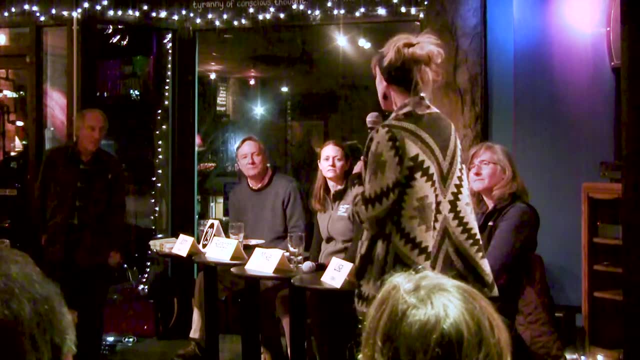 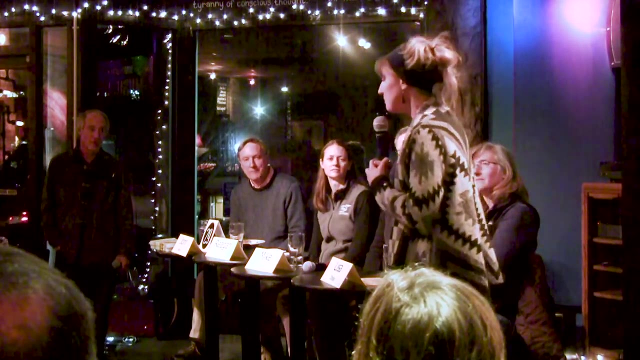 residents in nashua and compost in his backyard. so that was a success. but what he found was he didn't have enough space and he actually didn't have enough carbon to break down the compost. he was getting a lot of the nitrogen, the food waste and it was causing a mess in his backyard. 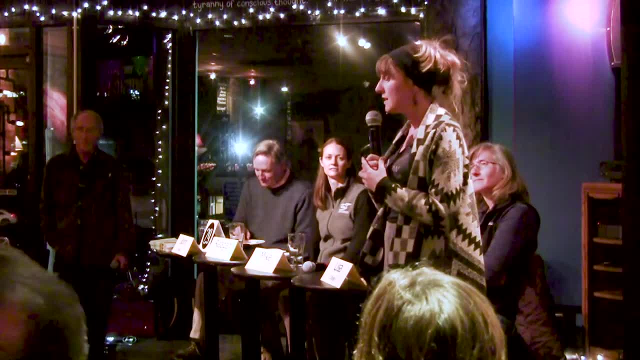 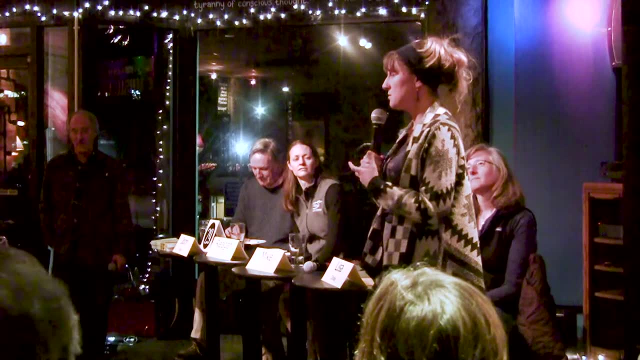 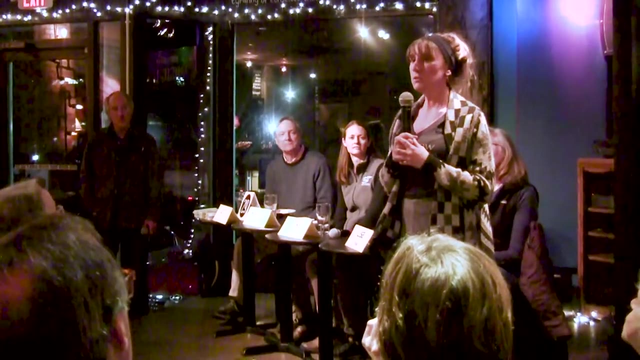 so then we're able to up with whole cycle. it's a an industrial or or commercial scale compost facility in mass or in maine, and so we're able to send our food waste that we collected in nashua up there to compost, to go through the compost process and then collect some, some of the byproduct to give back to our clients. well, what we found out? so whole cycle teamed up with agri-cycle. agricycle is a company, i believe, in massachusetts, and recently we renamed our program from food waste recycling or food waste pickup to curbside compost, just in. 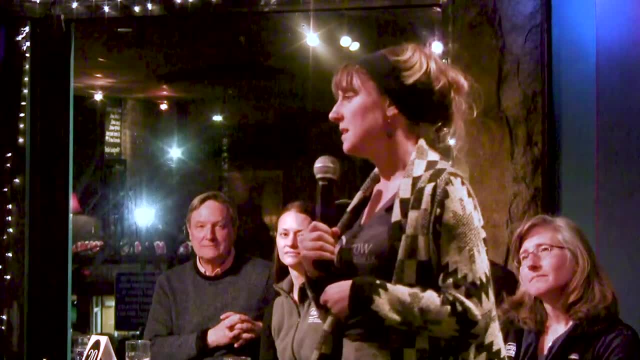 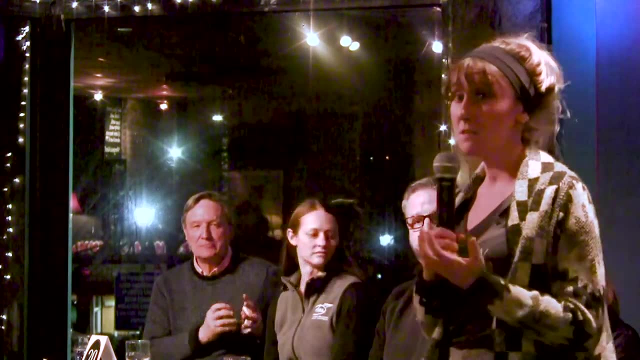 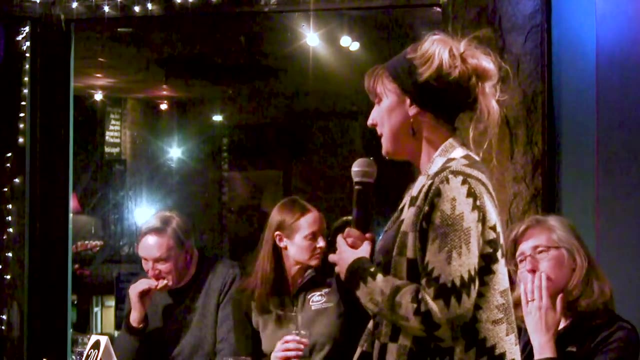 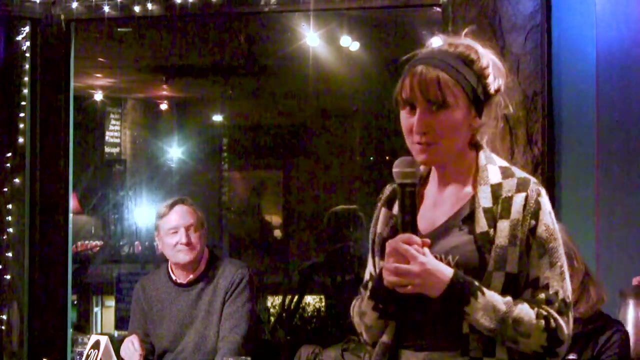 time for us to find out that our food waste is actually going to a biodigester or an anaerobic digestion facility, which is great news for climate change mitigation. it's a wonderful, It's a really neat program, but we branded our program as Curbside Compost. 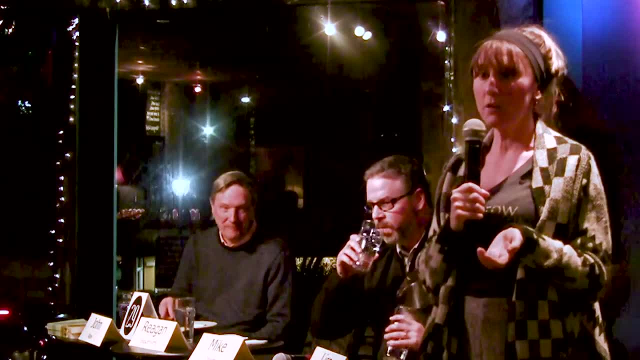 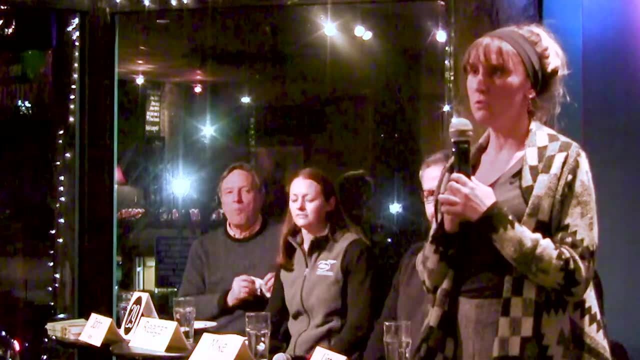 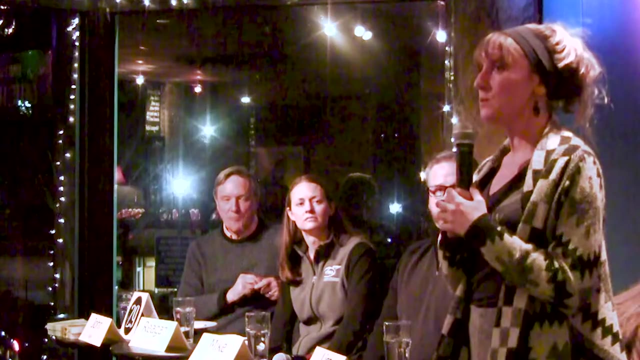 The cool thing about Agri-Cycle is, with their bio-digestion program, they got a state-of-the-art de-packaging machine that is able to de-package things like your salad mix or things that come in packaging, And so we're able to appeal to some larger clients- the soup kitchen, schools, faith-based. 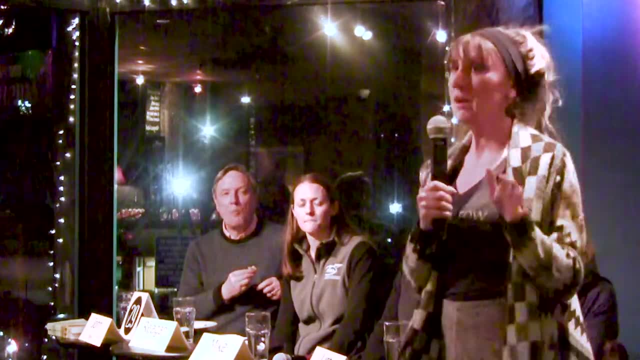 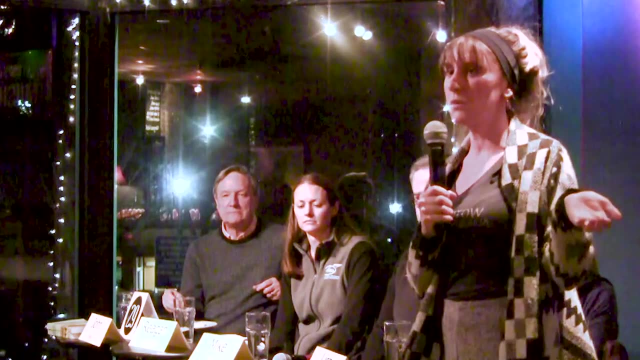 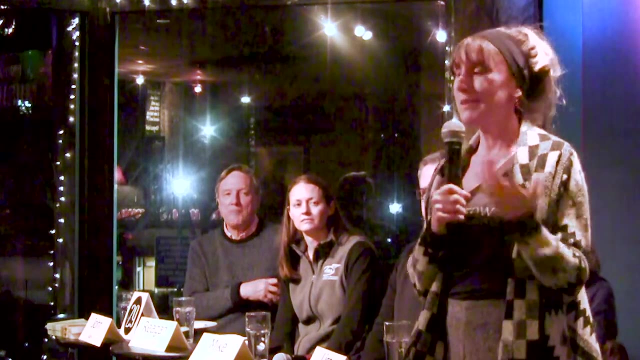 organizations, restaurants who don't have time to empty their rotten salad bags out, And we're able to offer that service and continue working with Agri-Cycle, but then also have our compost program with Mr Fox. So that's kind of all I have for you. 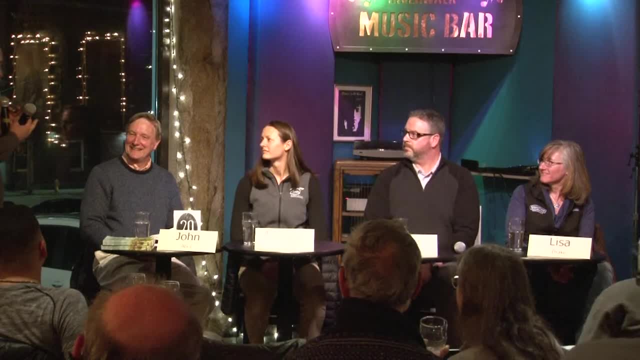 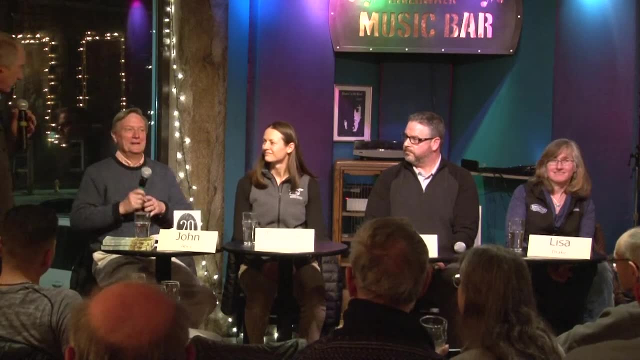 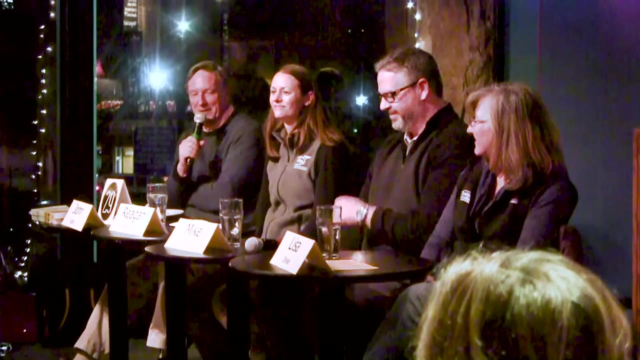 I want to ask: what is the right recipe for starting compost? Oh, How can the homeowner? what can we do? right, How can we get started? Well, you buy a carbon-nitrogen analyzer. No, No, But the comment about too much nitrogen in the food is a real one. 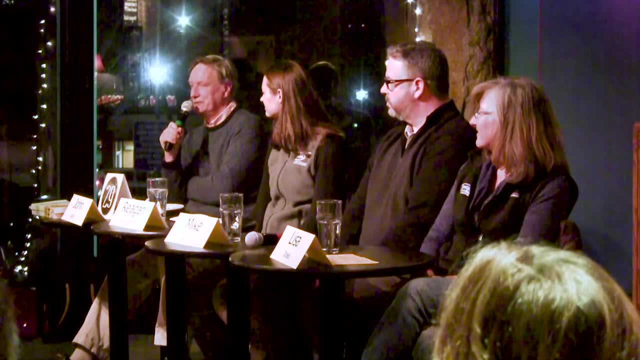 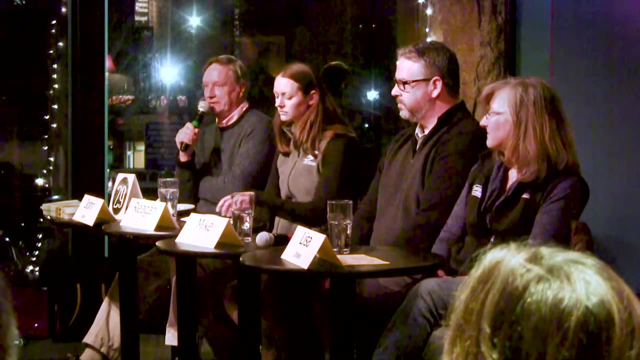 You need the right balance of carbon and nitrogen, So good carbon sources would be paper, cardboard, wood chips, whatever. At the Organic Dairy we take the stuff out of the barn which has been. We use wood shavings as bedding material. 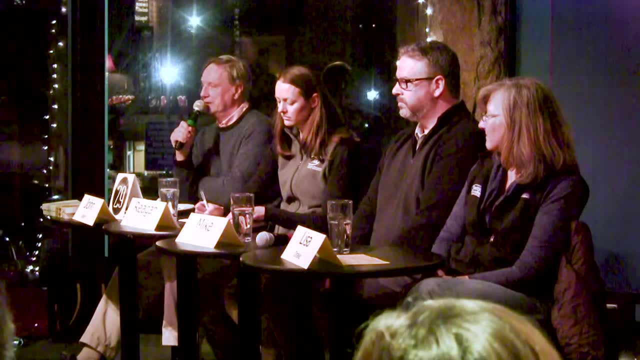 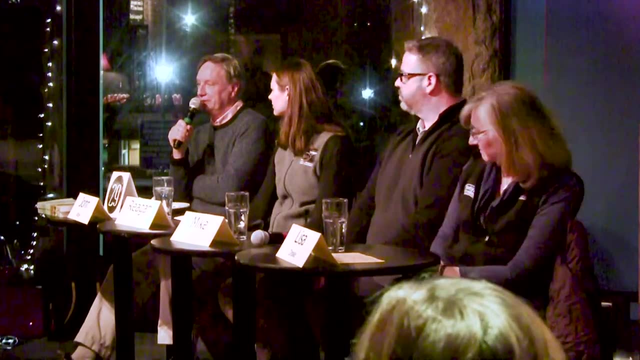 So it's probably two-thirds wood shavings, one-third manure Works really well. At the equine facilities they use hay and that stuff really cooks. In fact, once it got too hot we had to cool it down because it was going to catch fire. 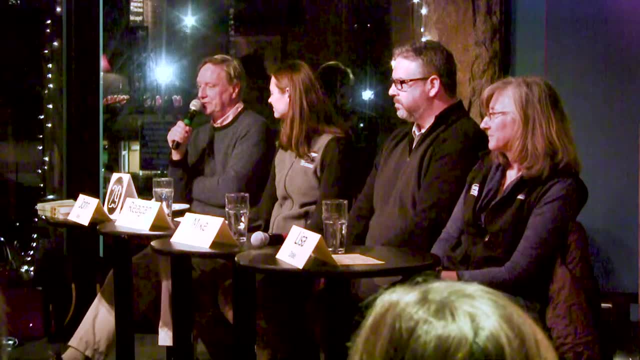 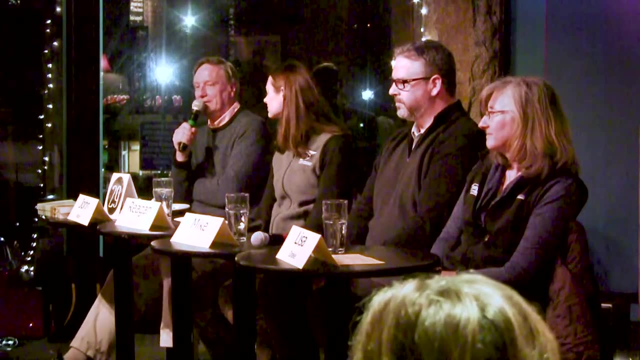 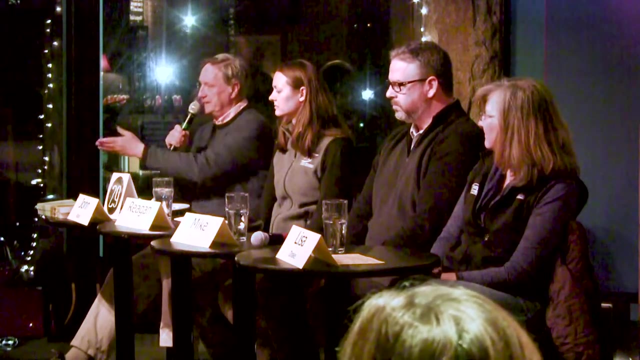 It got up to 170 degrees, So the student who was managing it was out of town. Fortunately his parents were watching the pile for us. So yeah Right, Amount of carbon-nitrogen. So food waste by itself probably needs grass clippings or leaves or something like that. It sounds like we've got some experience here in the front row. But yes, you do need. If you just do food waste- which I've been doing for years- in one of those big black bins, it disappears completely because there's no fiber in it or very little fiber in most. of it. You need fiber to form the organic matter, to form the humus. So you need leaves, You need grass clippings, although grass is pretty high in nitrogen as well. I forget the oxygen. Yes, you have to have oxygen, which is why people turn their windrow piles. 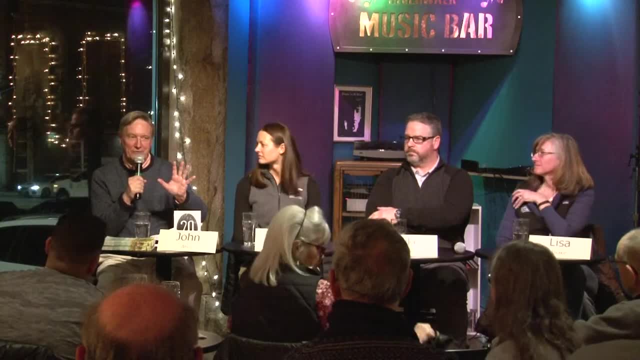 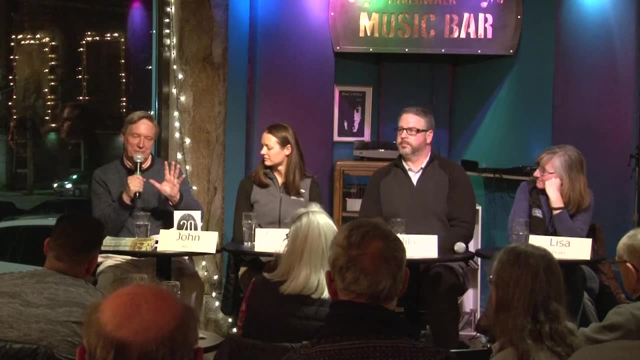 And I'm going to put in a plug here- if you really want to think about getting energy out of compost- and I know the digesters have kind of a checkered history- aerated static pile composting. That's all I'm going to say. 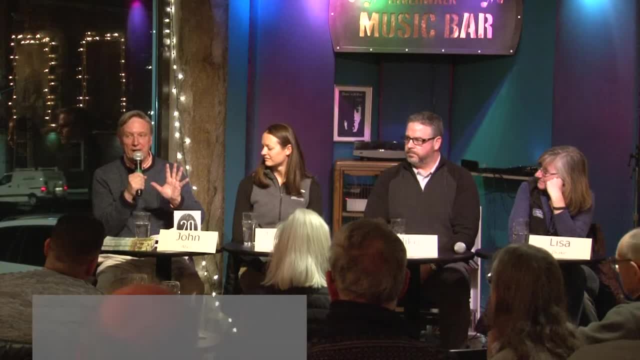 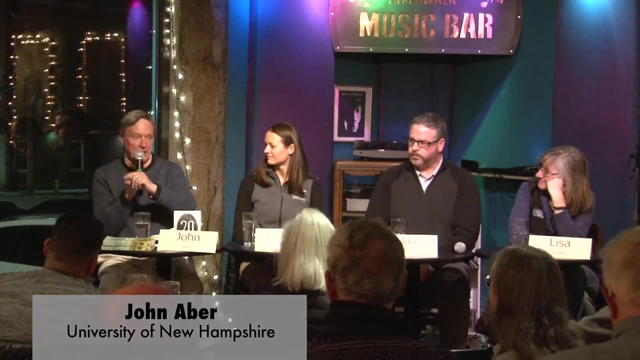 You can look it up. It's a pretty nifty way of getting heat energy out of this, if you have the right mix. There's a heifer farm up in Vermont. Ooh, It works too. All right. There's a heifer farm up in Vermont which was the first one to do this about 10 years. 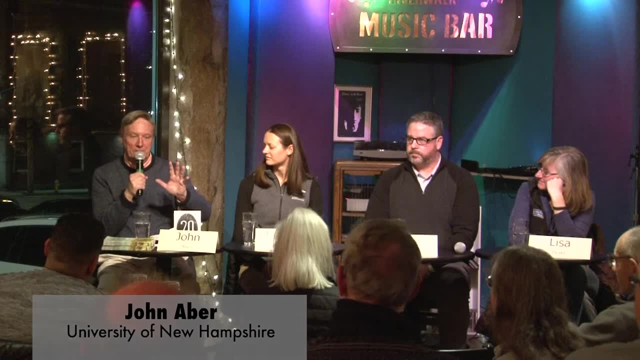 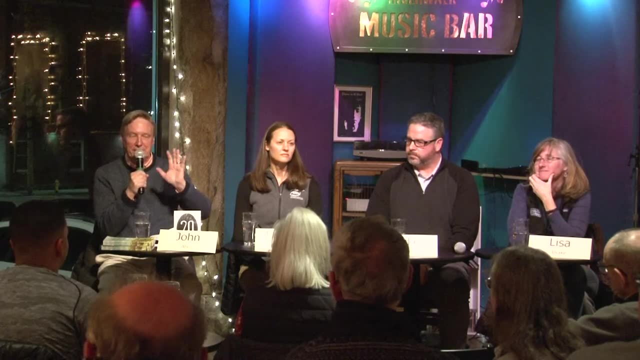 ago working with AgriLab Technologies. They get $10,000 a year worth of heat out of their waste through this method, So it's a fun thing to look at, And UNH has the only research facility that does that, so I think that's kind of cool. But yes, you need the right moisture content, you need oxygen, you need the right balance of carbon and nitrogen, something like 20,, 25 to 1 on those, And you can look up how much carbon and nitrogen there is in different sources and mix it. You can get really specialized on this too. But yes, you need all of those components in the right mixture. Is that a good enough answer? How long does it take? Whoa, So if you're a commercial composter, like Mr Fox or like City Soil Boston, they will. 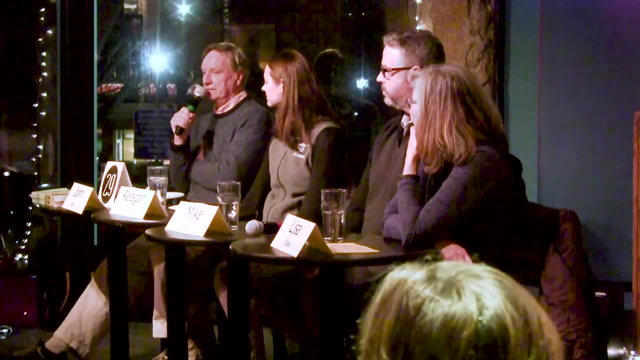 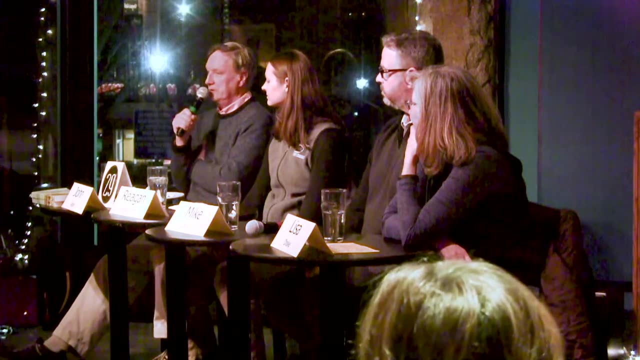 turn a pile around in 21 days. Now they can do that and we can do that at the place, at the Organic Dairy, because it gets to 150 degrees And it stays there for three weeks. So you lose about 30% of the weight, 40% of the weight, in that three-week period. Now, if you want to maximize energy from it, you might keep it longer, But these places they have a capacity issue and they want to get as much stuff through as they possibly can. So 20,, as I understand it, three to four weeks is the standard retention time. 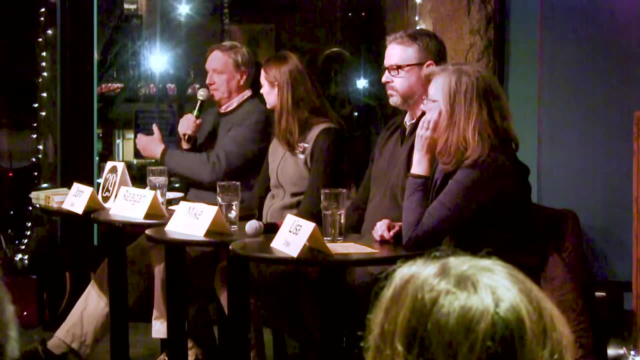 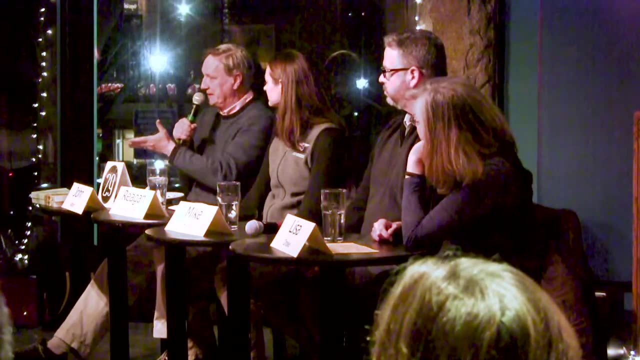 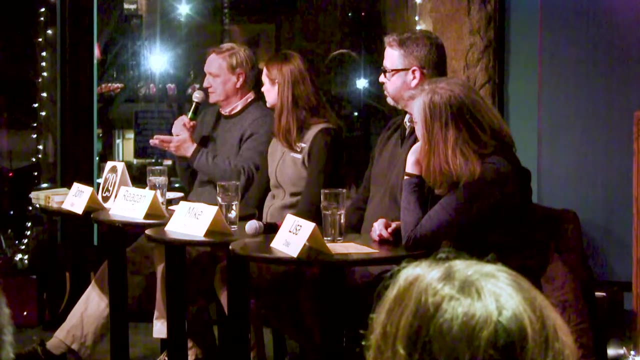 And then they'll offload it from this aerated system and it'll cure separately, I guess, for several months. Sometimes it has to be screened in order to be saleable compost, But it's a pretty high-cost, high-value product. when it's done, sell it to gardeners and landscapers. 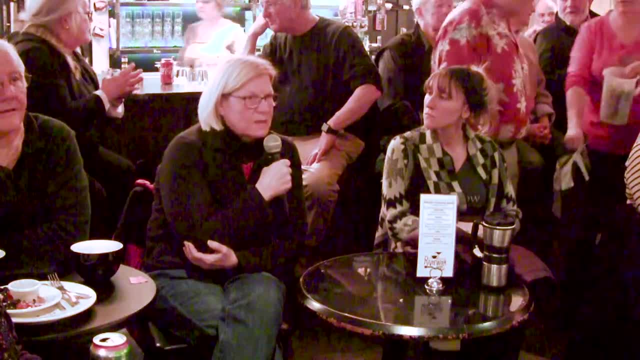 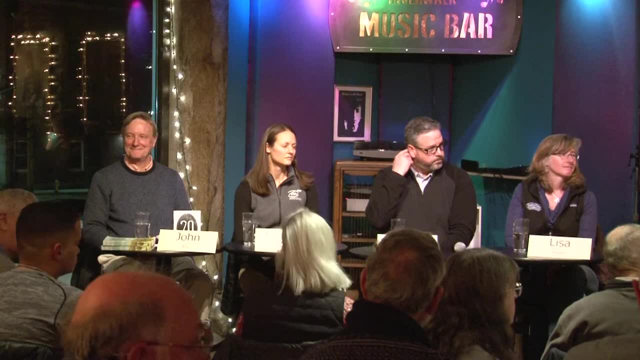 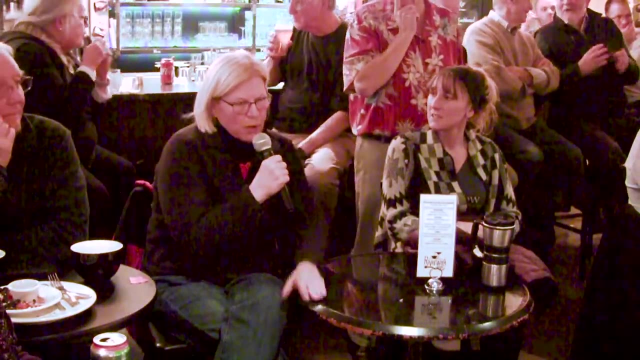 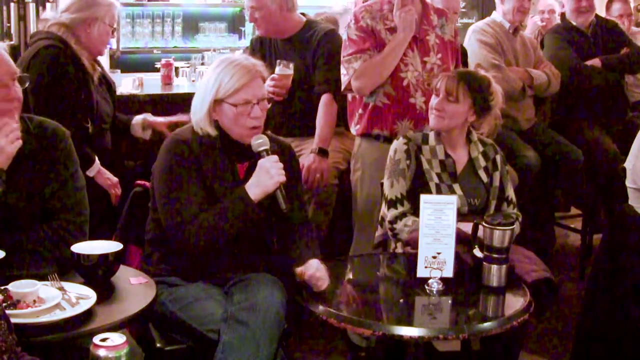 Can any of you speak to the textile waste that we have and recycling of that? We've done composting for a number of years. I've gotten to the point where I actually help take care of a property in another state where I bring some of the yard waste- more the weeds that I don't ever want to see again. 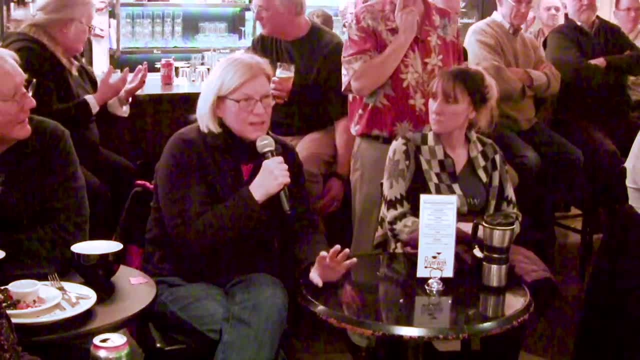 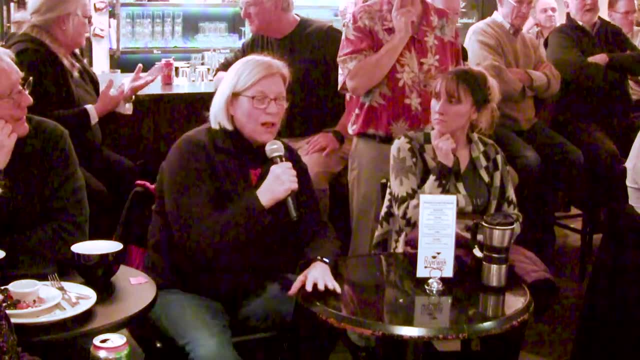 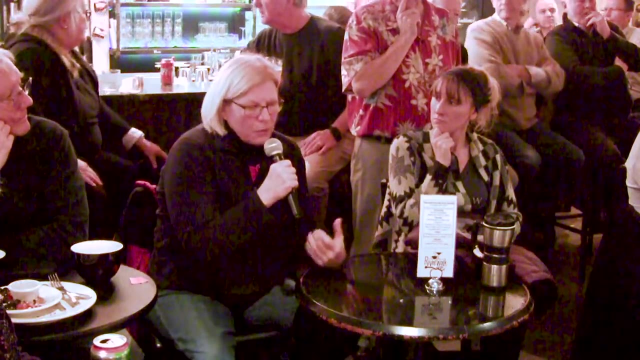 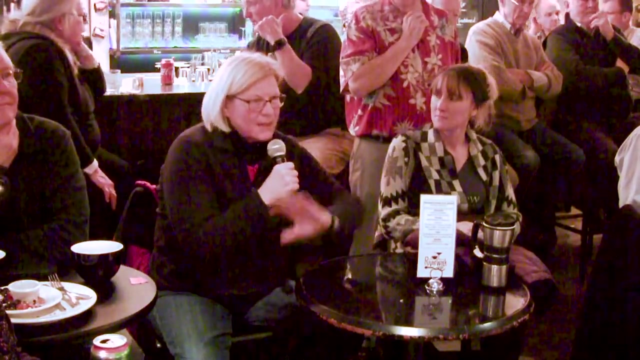 or invasive species to the dump where they recycle, Because I don't want that in my compost at all, that I would reuse, And that goes for the same for my own yard. I've got invasive species. I just, If I don't want, I bag it up, I take it to the stump dump. somebody else can deal with. 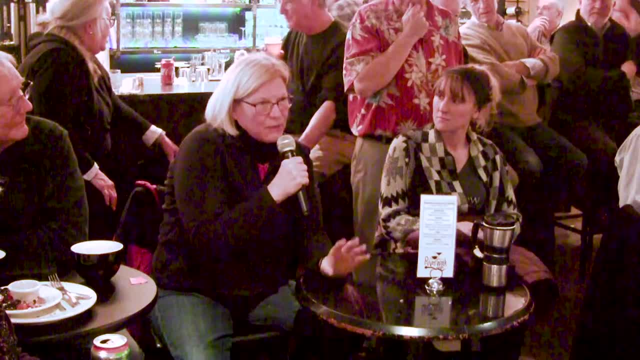 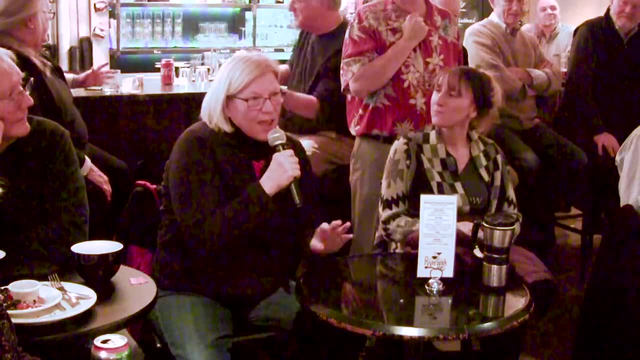 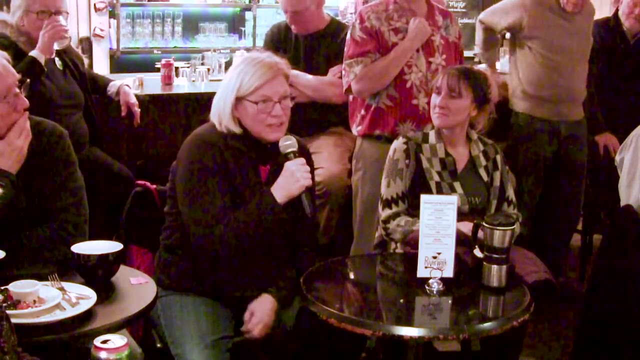 it. However, I feel bad for those people who take that compost and might have at the dump and use it in their yard and maybe they might have an invasive species that they might not want. The commercial composters with the large piles and the high temperatures will kill most of. 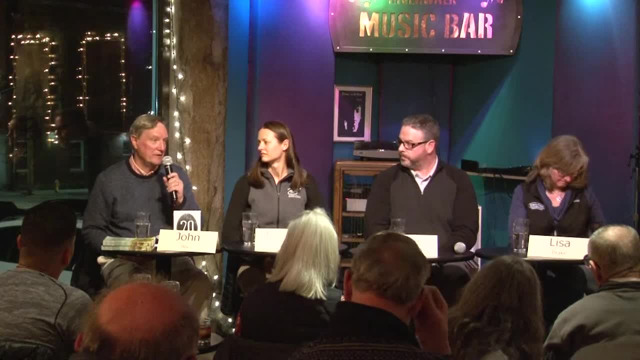 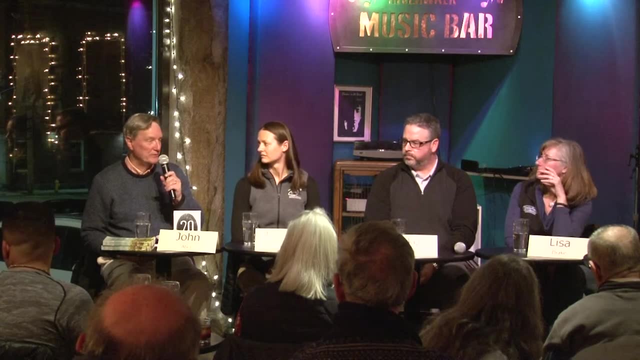 those things, They'll kill the seeds, they'll kill the bacteria, they kill. That's why, in order to actually use compost on an agricultural situation or in a garden, it has to go, I think, above 130 degrees for three consecutive days or something. because, 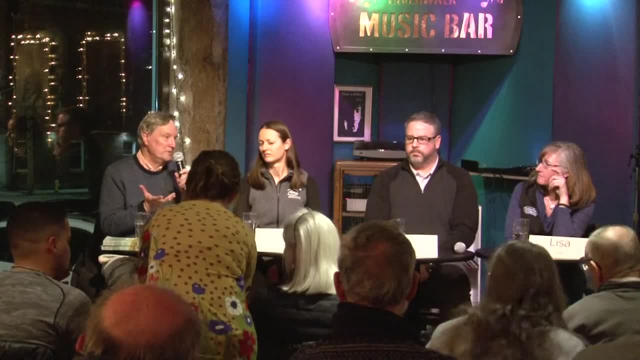 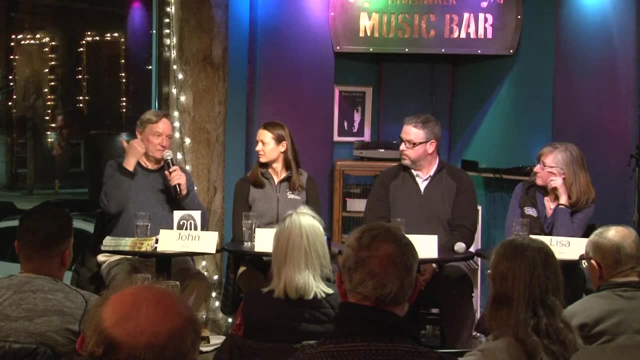 that effectively sterilizes the material. Backyard compost piles will never get that way. My wife is a master gardener person and she says: see that fungus on that. That's going to the dump. We don't want that in the compost pile. 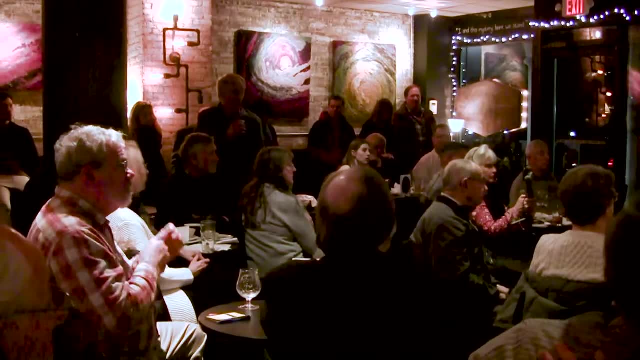 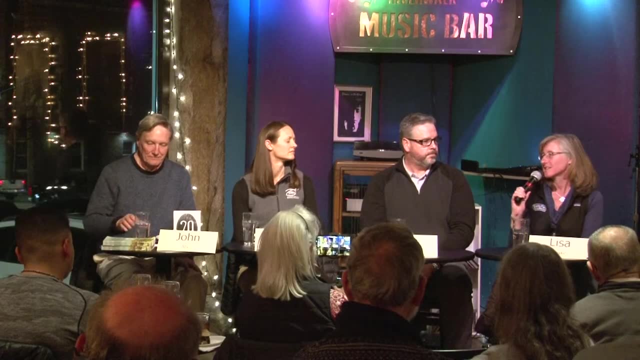 So in Durham they burn that stuff. On the textiles question, do you have any? Sorry, Do you have any things? I just have an anecdote. I don't have a great answer, but I have an anecdote Just on the textiles thing. I don't think that there's great textile recycling going. 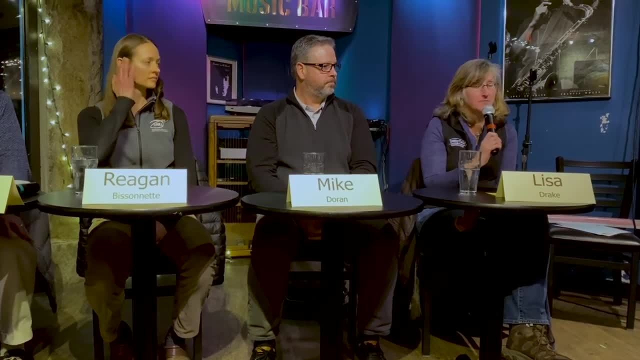 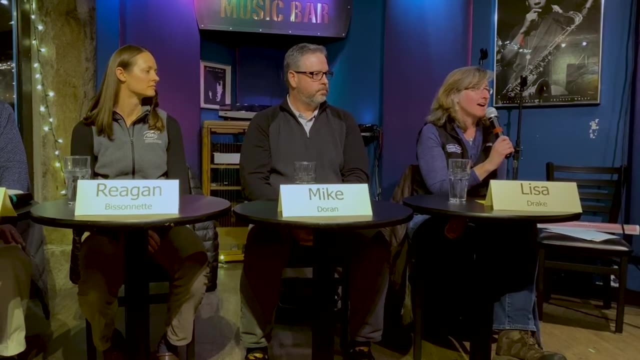 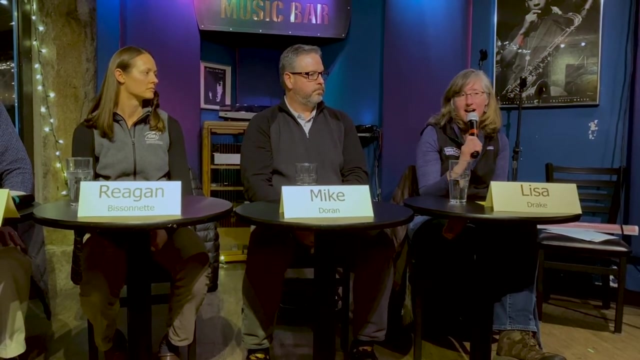 on in the world, but correct me if I'm wrong. I did get the opportunity to visit a facility owned by the Eileen Fisher Company. This is really interesting. Eileen Fisher is fairly high-end fashion. I don't know if you've heard of her. 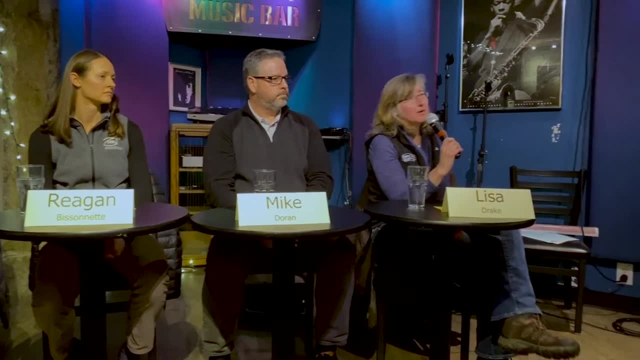 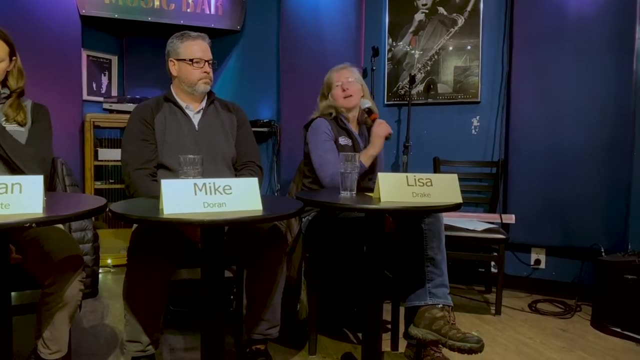 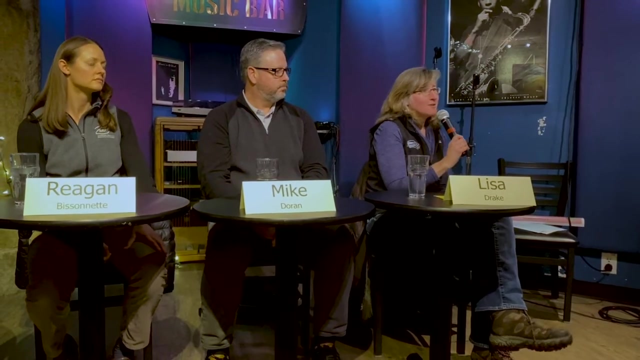 She's a great, But they, If you buy Eileen Fisher products, it's designed to last nearly forever. It's designed to be timeless- I guess is the better way to say it- stylistically and quality-wise. But if you are done with your Eileen Fisher clothing, you can send it back to their facility. 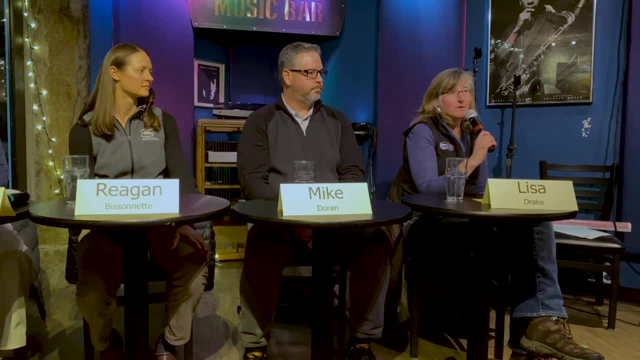 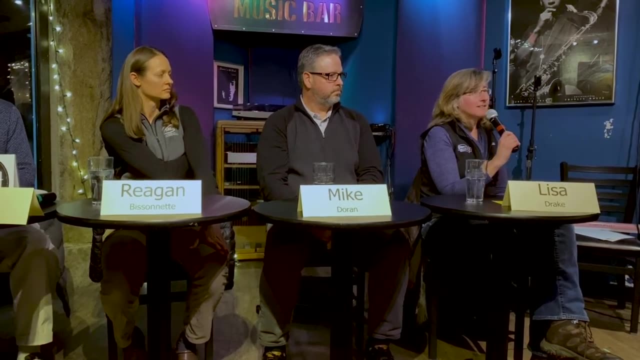 and they take it all in wherever it comes from and they go through it And if it's something that's still usable, they have reselling stores where you're buying secondhand Eileen Fisher clothes, Eileen Fisher clothing. they of course clean it and refurbish it and sew buttons back. 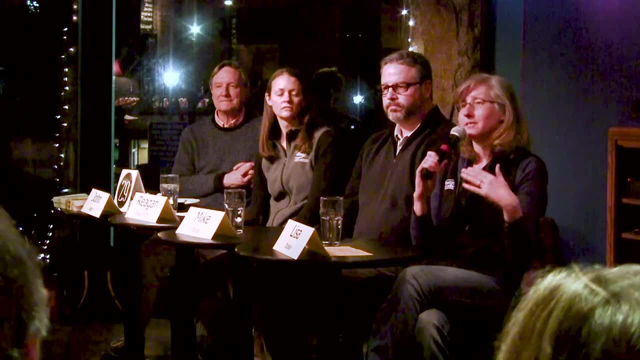 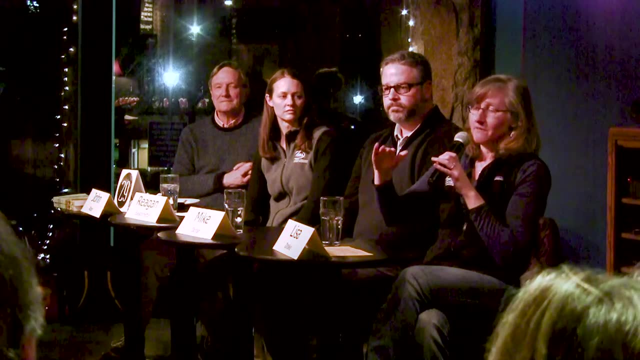 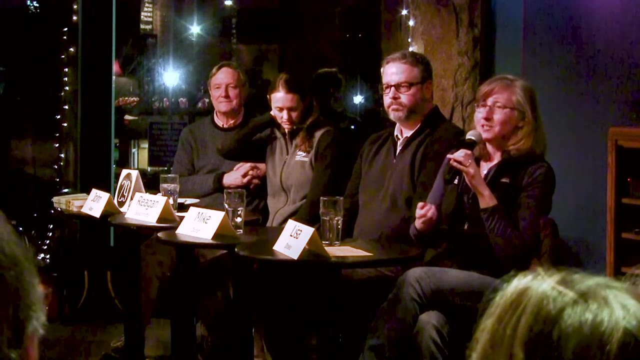 on and things like that. if needed, If it's not good enough to resell, then they have all these other things they start to do with it, And so they have designed styles where they have some very basic items that keep coming back. They sell a lot of these basic black pants. 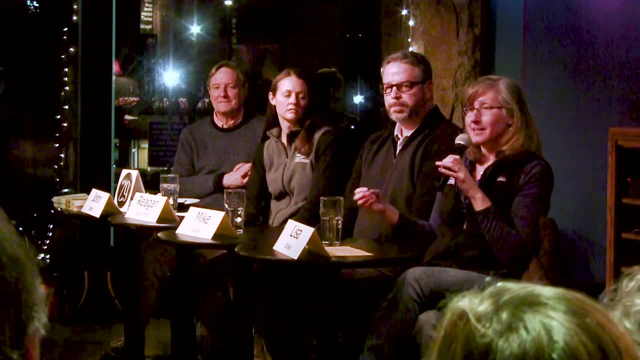 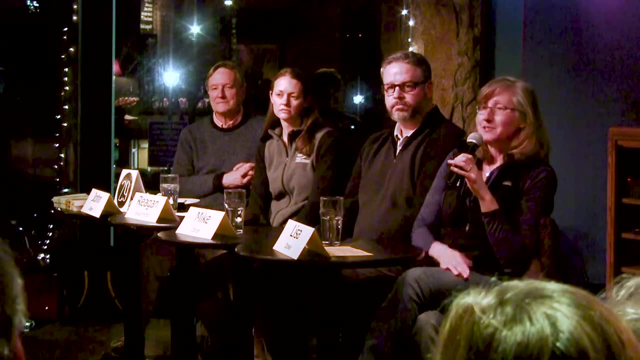 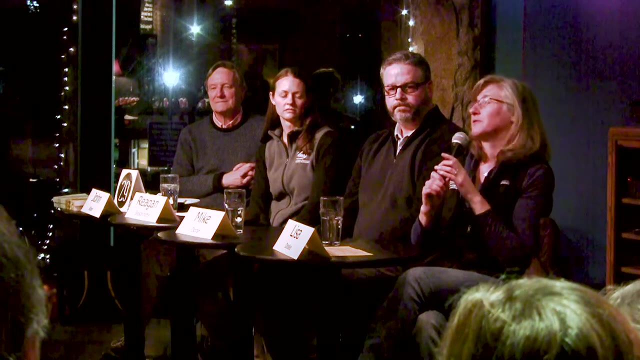 And so if they receive some that has a hole in it, they're not gonna resell it, but they take pieces of the fabric, they cut it out and they start making new items. And then, finally, if the fibers are completely not usable for clothing, then they have invested. 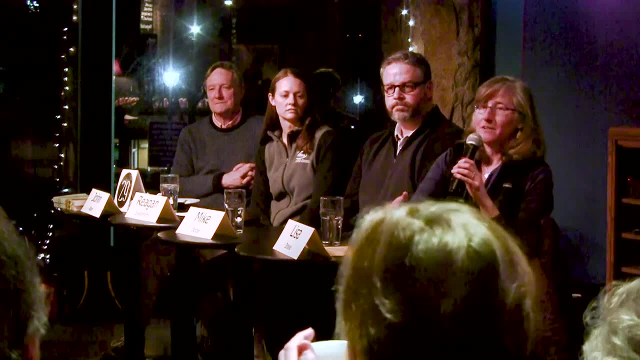 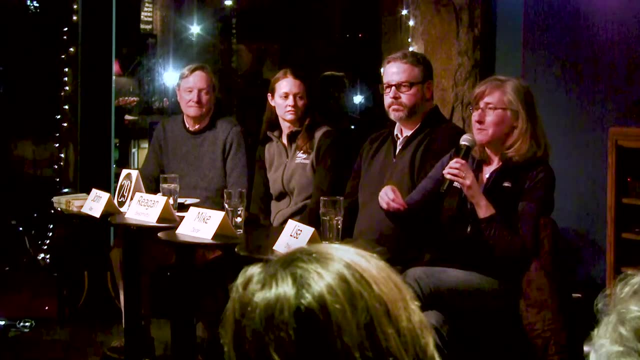 in some machinery that essentially weaves fibers back together to make these kind of really neat, intricate designs from all sorts of different fibers and different colors and whatnot. And then they're making like pillows, pillow covers. And then they're making like pillows, pillow covers. 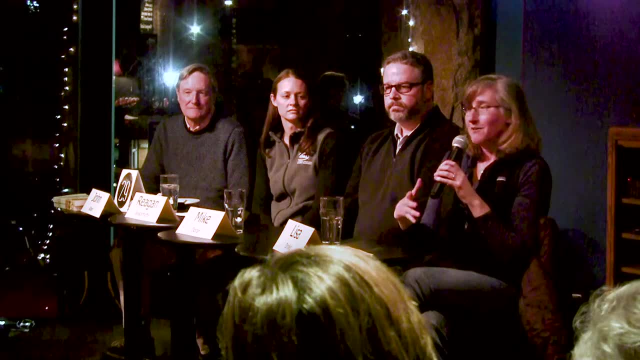 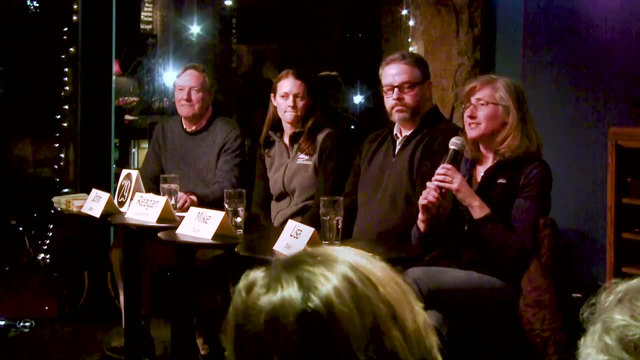 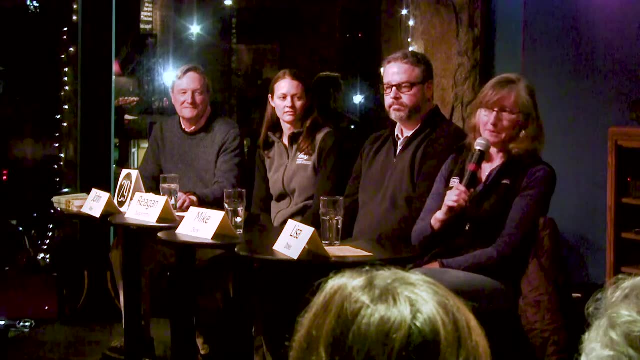 And things like that that they sell for your home, And these also are very expensive at the end of the day. so this is not a cost saving, a moneymaking venture for them, but it's a very interesting experiment about what you. 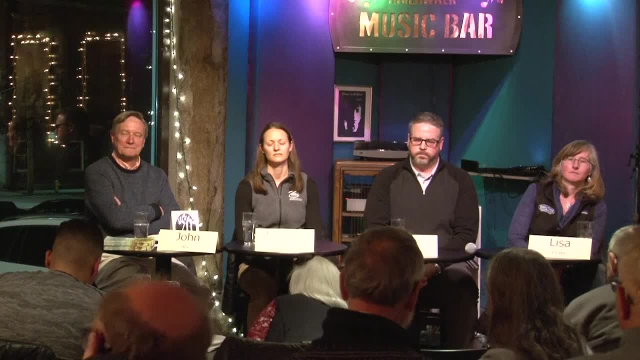 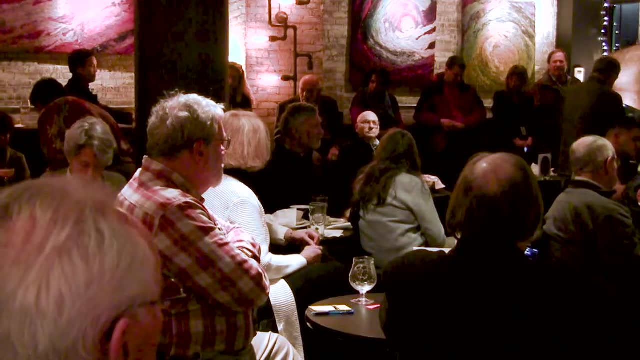 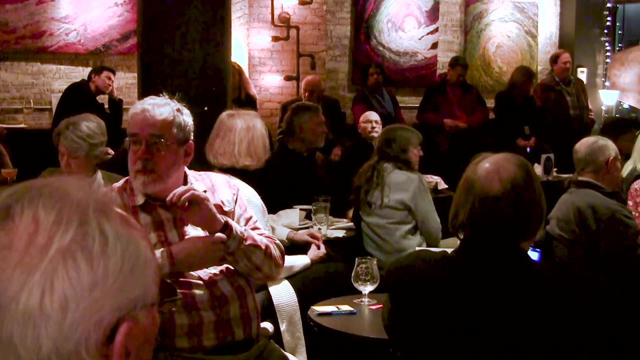 can do with fibers. I have a question and an observation and a comment. About 35 years ago, some of my business colleagues were working on something called waste to energy. This was after the big runup in oil prices And we eventually gave up on it because it seemed to become not as viable. 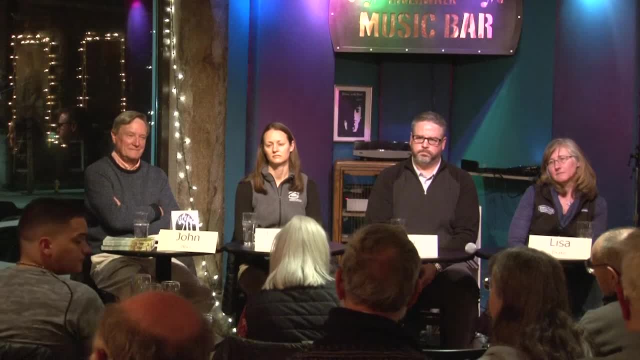 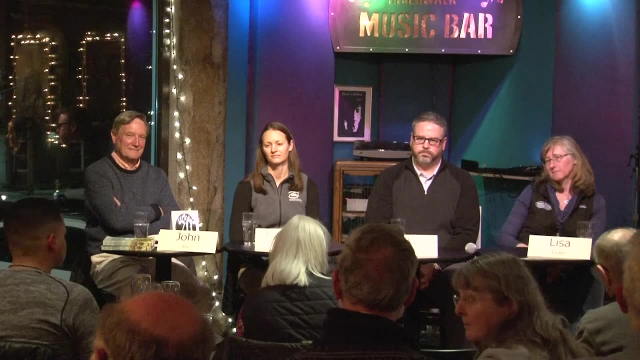 I have a feeling there is a waste of energy and we don't like to talk about it because it doesn't sound as good. so I like your comment about that. The other comment I'd like to make is: what drives me crazy are all these people? 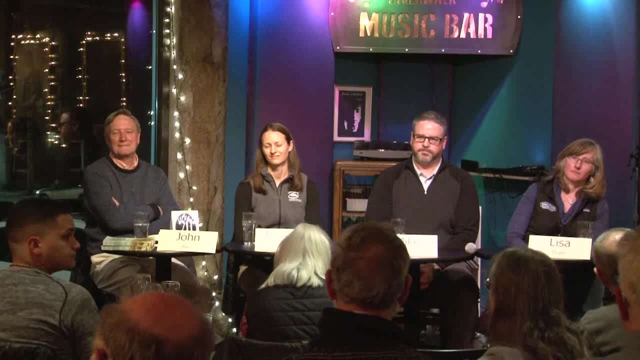 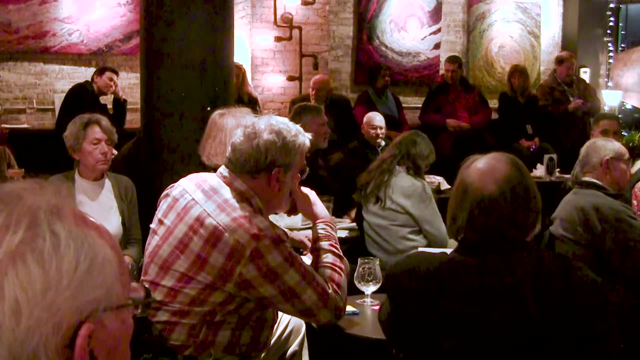 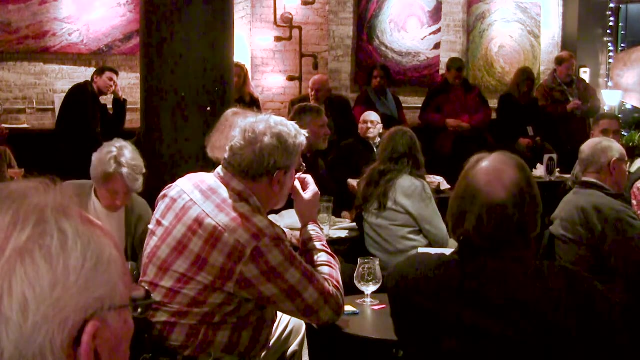 running around telling me I can't have a plastic bottle for water. Frankly, that's the easiest recycling thing on the planet, And I'll quote from this same business. according to this guy that I talked to a little while ago, they process 7 million soda and water bottles a day. 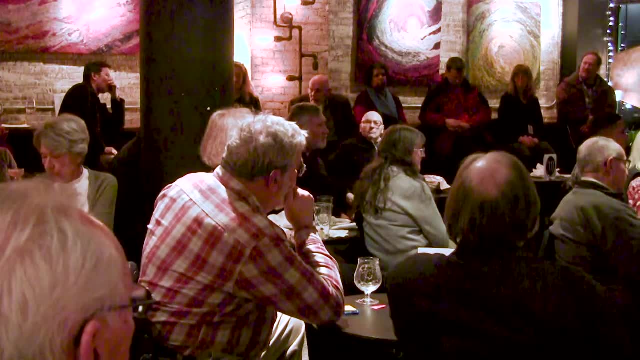 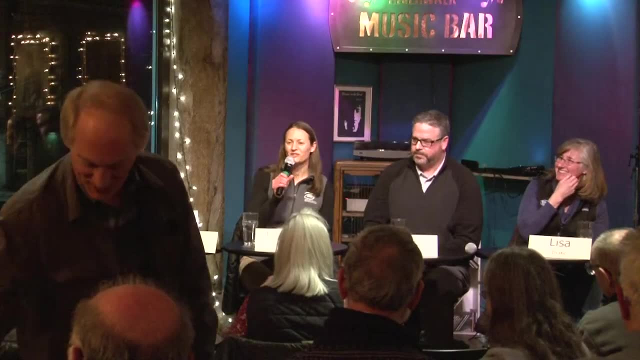 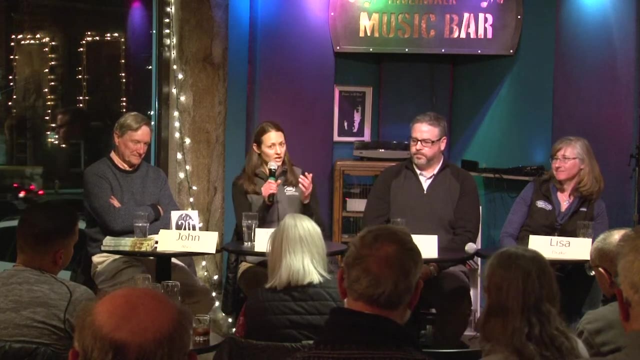 and cover all of the Northeast, So can't we talk about that? that that's okay, that is recycled. Do we have to have paper water containers? Well, as I mentioned earlier, when you look at the most financial value in our residential recycling right now, it is in Those number one and number two plastics. Your soda bottles are the number one peats. You've got your number two milk jugs and your number two colored sort of detergent bottles and such. There is a strong market for each of those. It's some of the remaining plastics that don't have as much of a strong market. There is actually a good market for number five plastics, but not as much. We don't see as much of that getting recycled in New Hampshire, for example. if you're source separating. 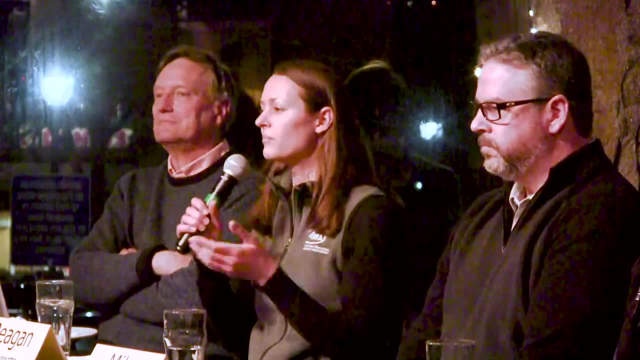 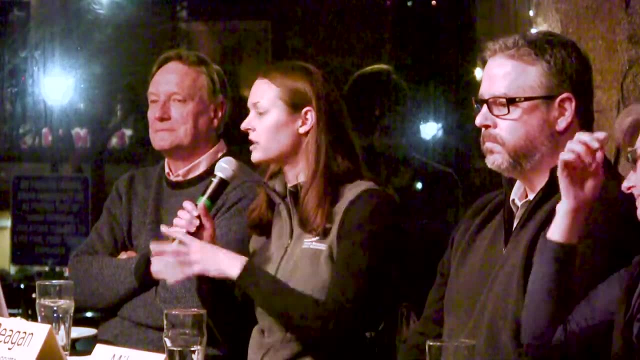 But if your single stream recycling is getting exported out of state, which it is, there very well may be good markets for the number five plastics, But at least if you're talking about rural communities that source, separate number one and two plastics have very good value. 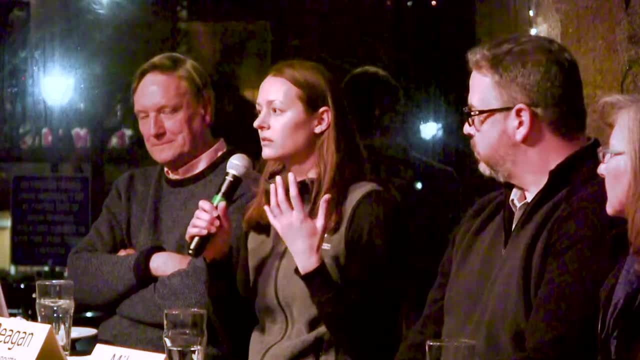 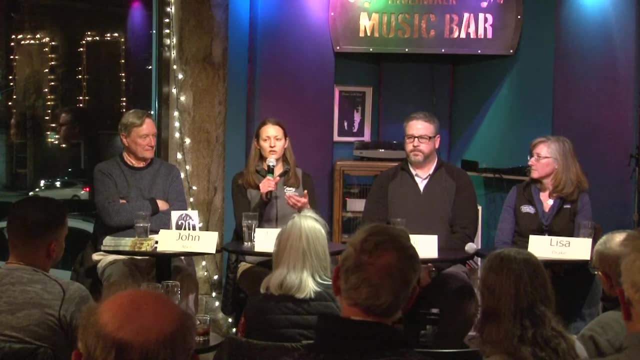 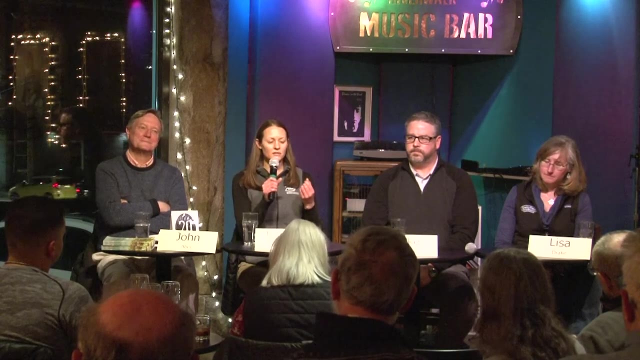 And, interestingly, you may have heard that a number of big conglomerate companies have been putting out goals that they would like to achieve a certain amount of recycled content in their plastic packaging by certain years And there was a very interesting study that was done by 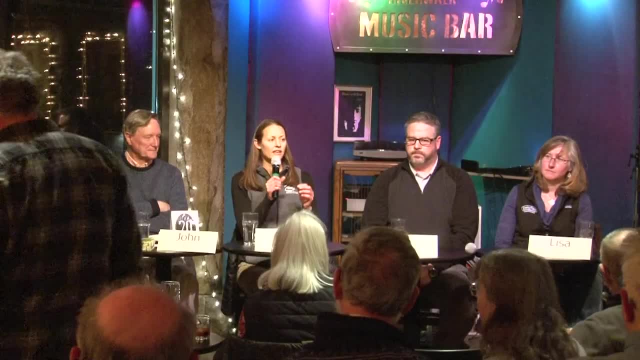 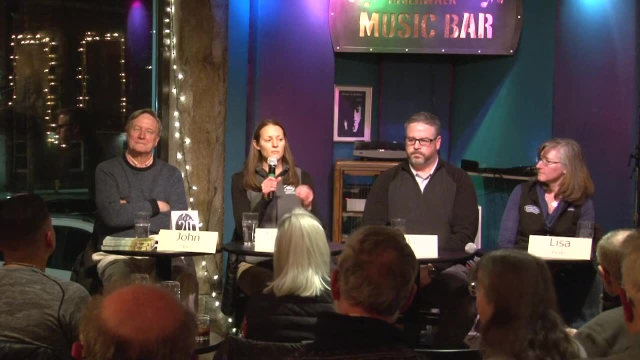 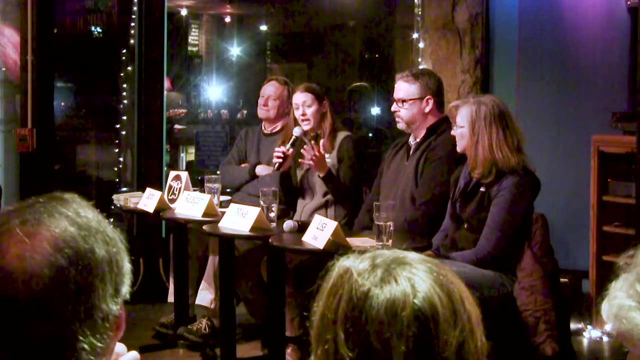 I believe it was by the Recycling Partnership, where they looked at the available supply of plastic that is currently being recycled versus the amount of plastic that would need to be recycled for all those companies to meet their goals, And there's a huge gap. There's a huge gap because, even though your soda bottle, 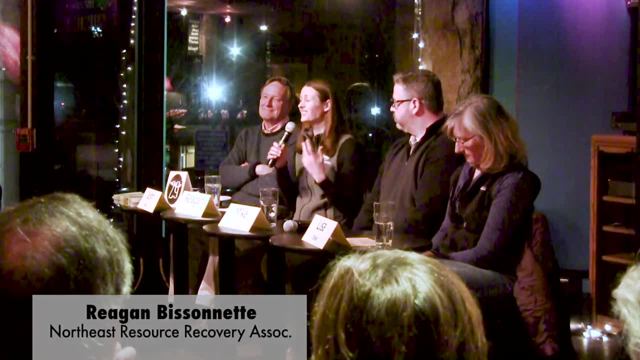 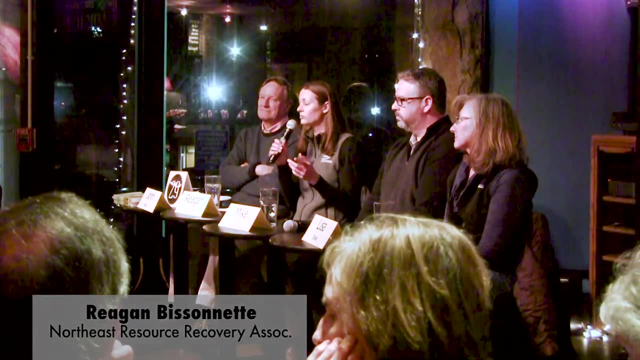 your water bottle in plastic is highly recyclable, a lot of it still is thrown away, So we actually need to dramatically improve the recycling rates for those number one and two plastics in order for these companies to even be able to achieve their stated goals. 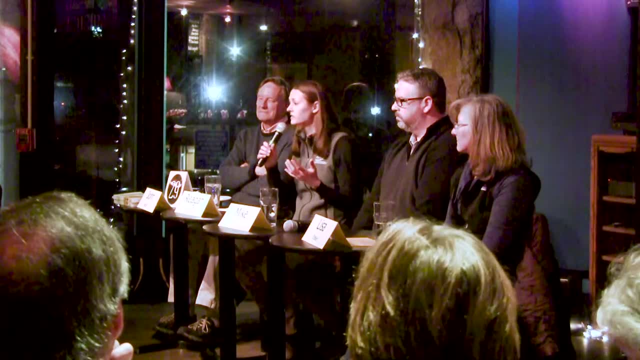 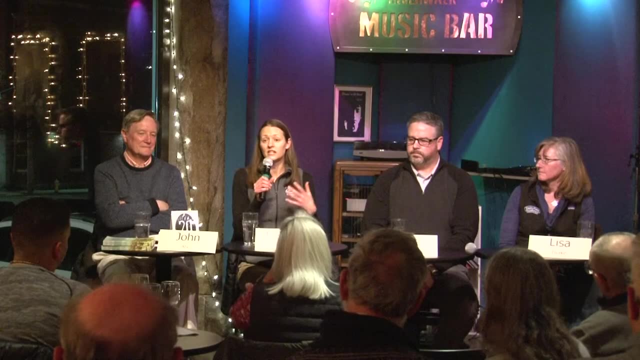 So there's quite a big push across the country to include to improve curbside single stream recycling so that those companies can actually get the feedstock they need to increase their recycled content in their material. Just to pick up on that a little bit: 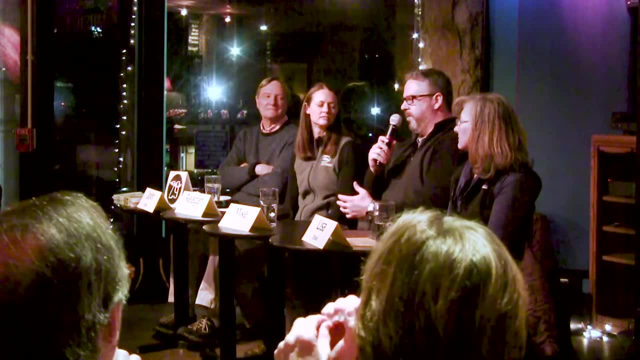 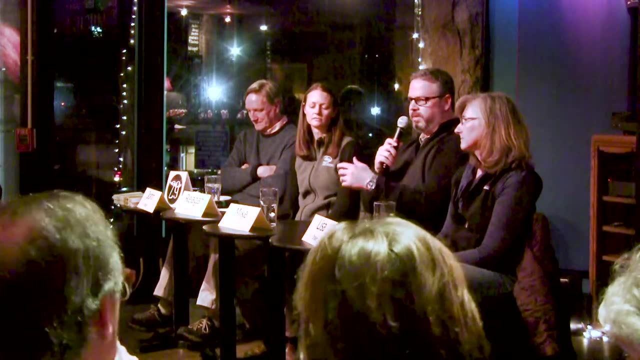 one of the, so some of the companies that we have worked with in the past, some of the waste management and recycling companies, a lot of what you're talking about, like the bottles and even the plastic bags. like I know, part of the plastic bag ban was because these bags. 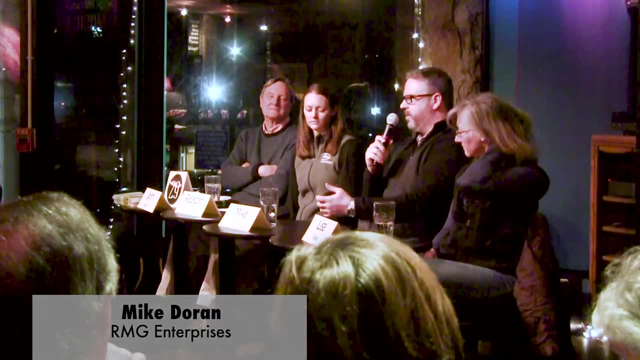 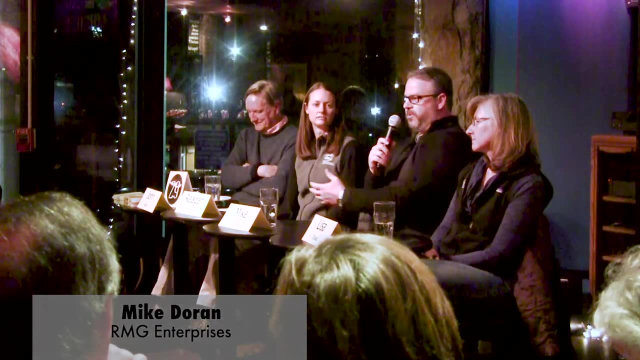 once they go into like a single sort facility, they get wrapped around the screens- okay- And then you have to shut down the operation to clean off the screens because you're not recycling any of the other materials, So it's a contaminant to the waste stream. 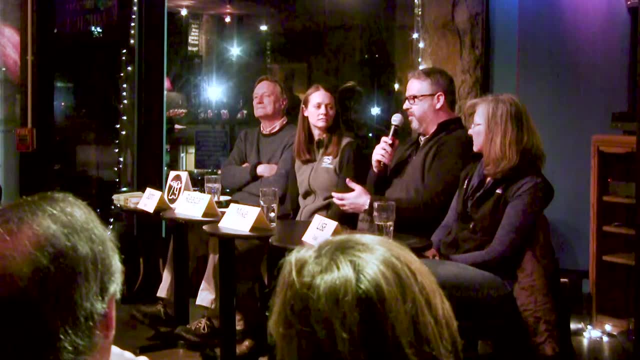 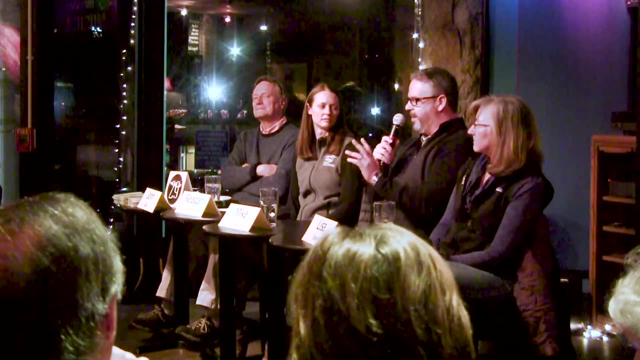 Even if it's recyclable. it's the operational challenges that come along with some of these products And I think the water bottles. what kind of? was the? I don't know this for sure, but part of the genesis of the banning the water bottles. 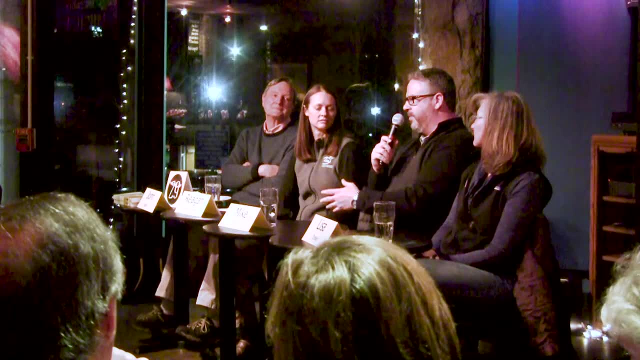 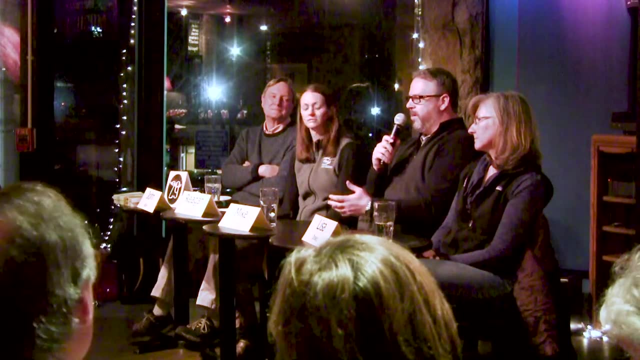 I live in Woburn Mass And I know Concord Mass was one of the first towns to do this And, if I remember correctly, a lot of the press about it was, you know, the water bottles at the river's edge. 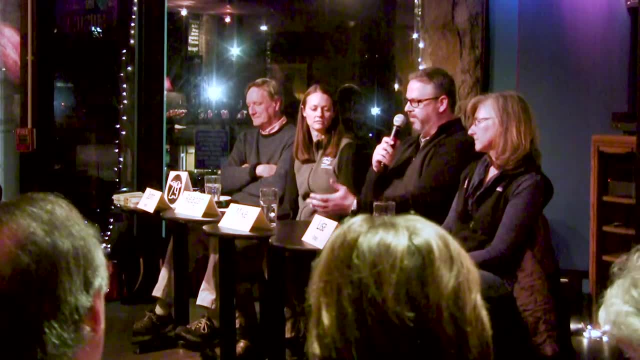 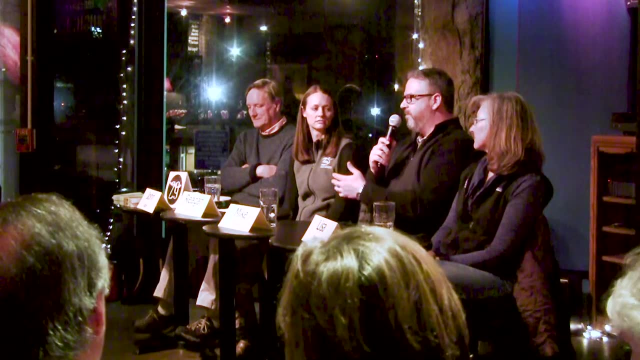 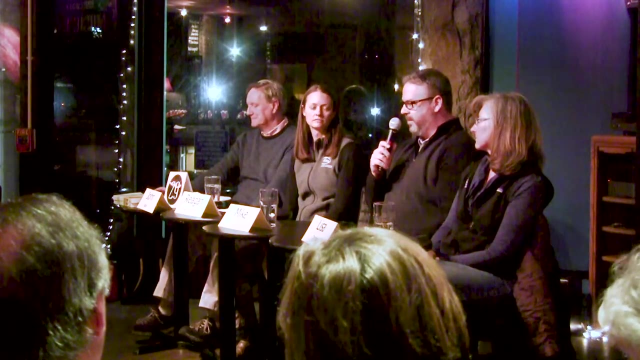 and more about the pollution impact of these water bottles everywhere and the visual of it. So there are other factors that go along with just: are there markets available? How difficult is it to recycle material and collect and process? Recycling is important and it's good. 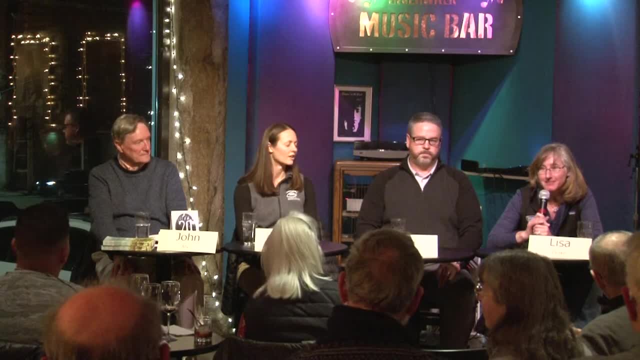 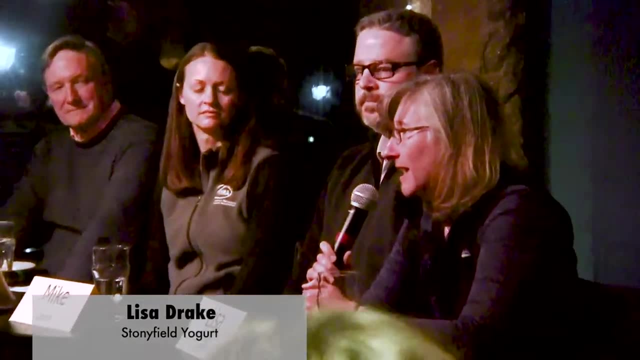 And yet if you can avoid using that water bottle altogether- you know back to the zero waste idea- then that's better Because there is energy used in making that recycling happen, Because it needs to be transported. It came from fossil fuel to begin with. 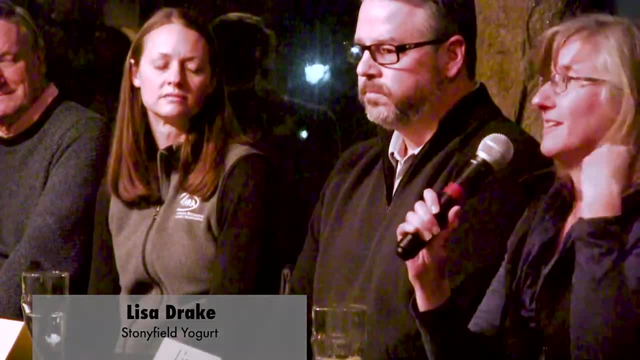 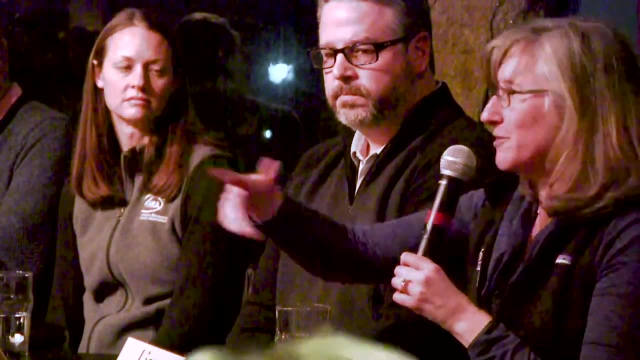 and then it had to be manufactured, and that took energy and it needed to be transported, and that took energy, and then it goes wherever it travels in its life and it takes energy to recycle it. So all of those things do have impacts. So, where you can avoid, 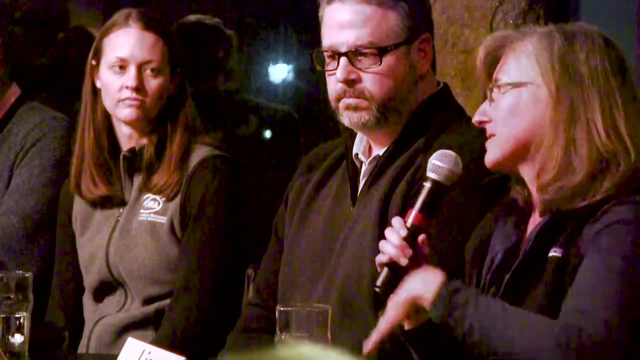 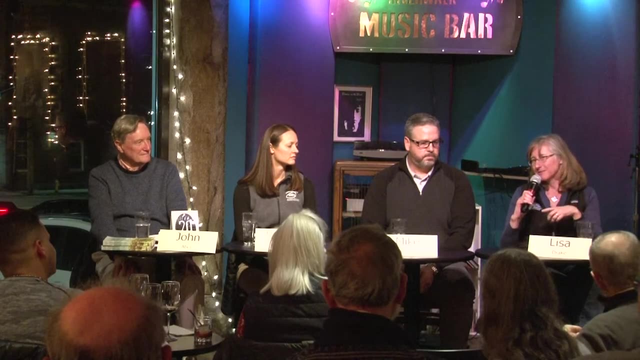 rather than recycling. you know that is better. That's like sort of the hierarchy right of reduce, reuse, recycle. And then the other thing that you're getting you started to allude to is plastic versus like some other alternative container. 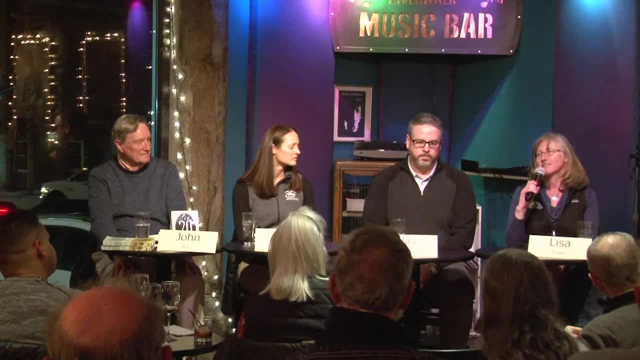 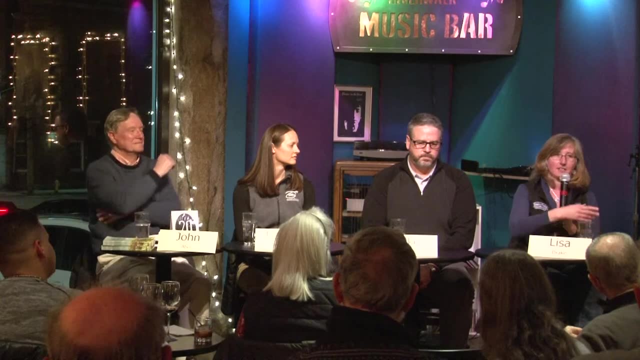 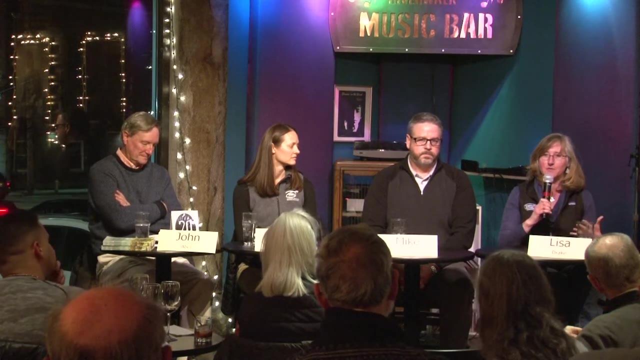 for your water And I just wanted to just mention that because you know, we really think about life cycle of packaging and impacts, like through all those steps that I was just kind of describing with a water bottle. You really have to think about all those things. 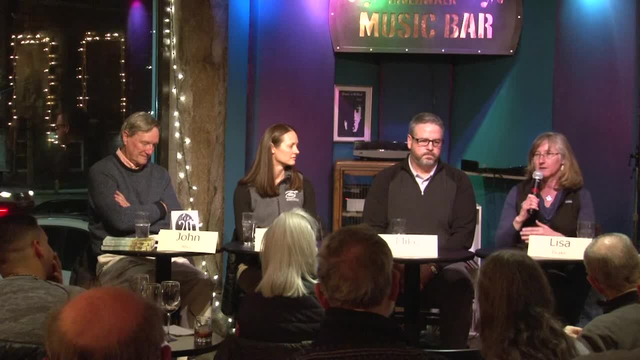 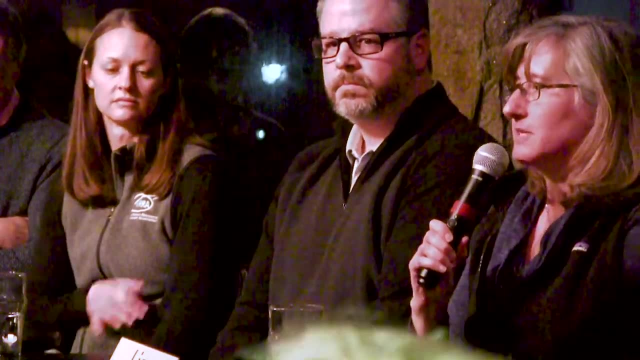 because recycling issues are really important. They certainly have impacts on communities, But when we think about what is the impact of our packaging, we do think all the way back to: where did this material come from? Did it come from petroleum products? What are the greenhouse gas emissions? 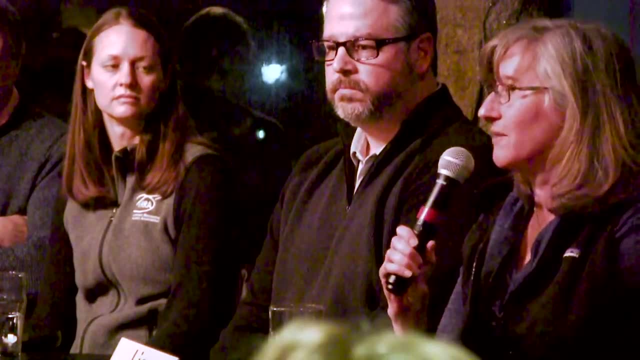 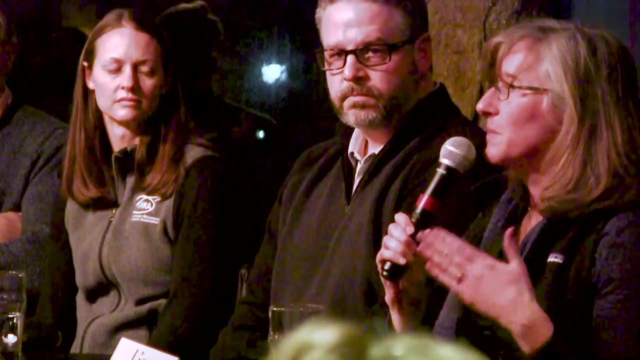 associated with taking that fossil fuel out of the ground. And then what are the greenhouse gas emissions with all those steps in between? And that, all in all, the best decision we can make is to use the least amount of material, to be thinking about it- in greenhouse gases. 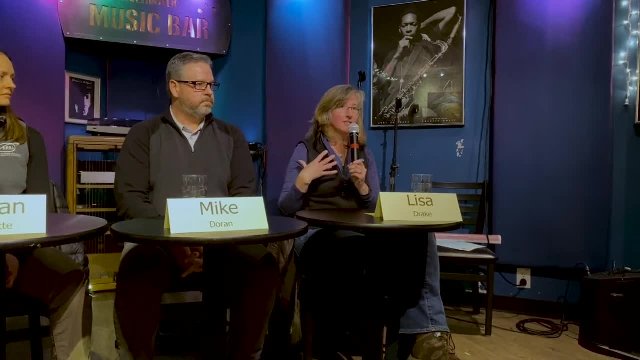 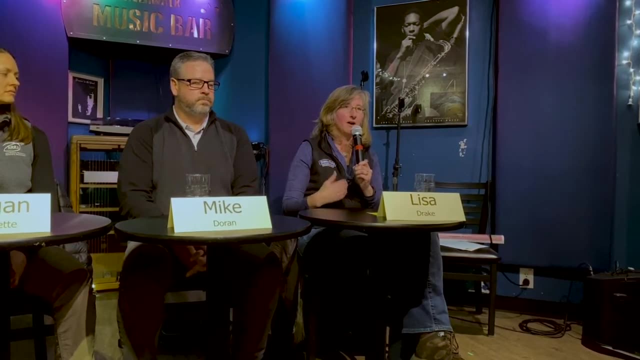 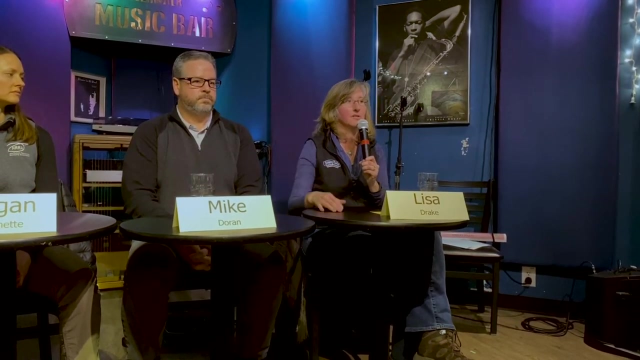 because the end of life of our package is only about 3% of its overall impact in its life. So that's why we make a product in this plant-based plastic that can't be recycled and generally can't be composted unless you go to an industrial composting facility. 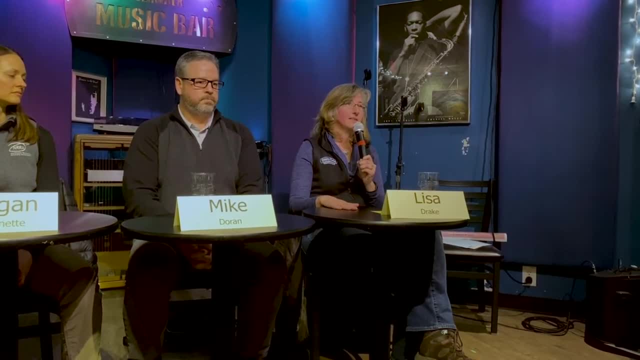 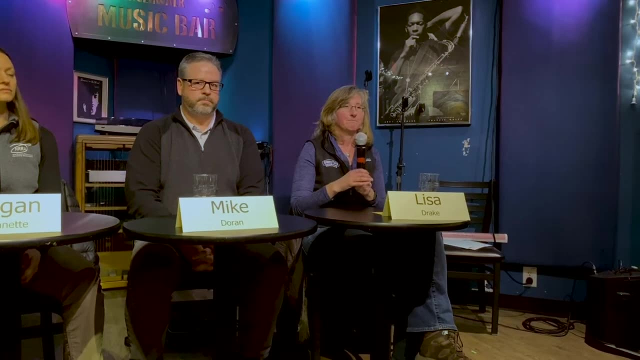 But we still felt it was a good improvement because it's not using those fossil fuels to begin with and has roughly half of the overall impact. So it's complicated. Hi, I've been reading a lot lately about microplastics in the ocean. 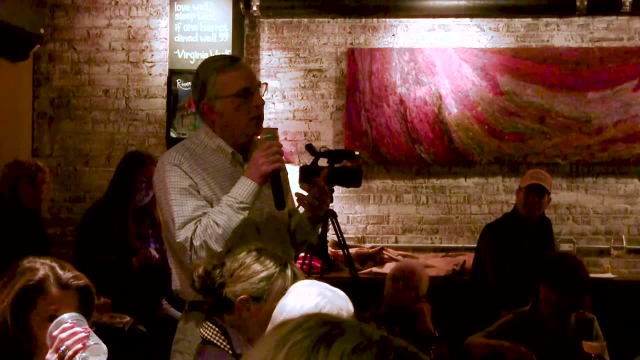 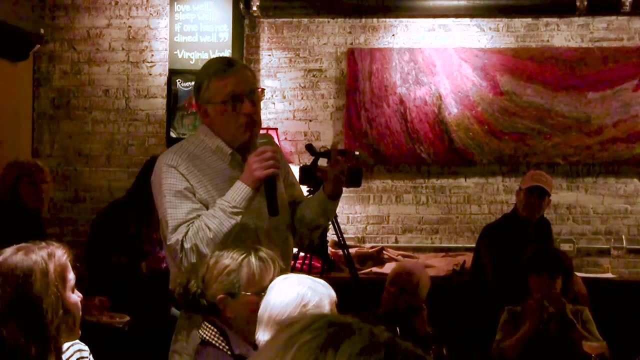 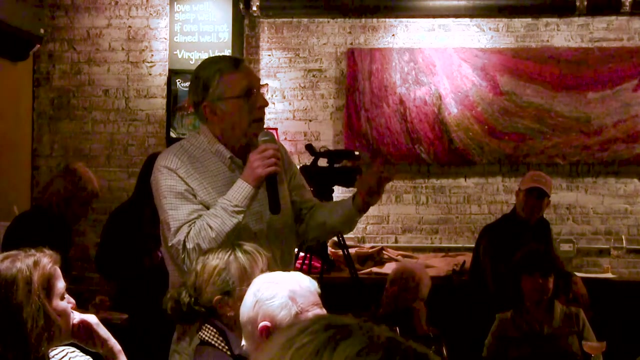 And my question to the panel is: what kinds of things can we do to help mitigate the plastics that are going into the ocean And, in particular, are there certain kinds of plastics that we could avoid using that would not lead to microplastic accumulation in the oceans? 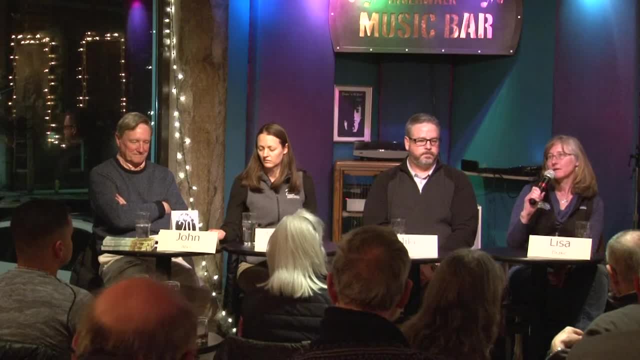 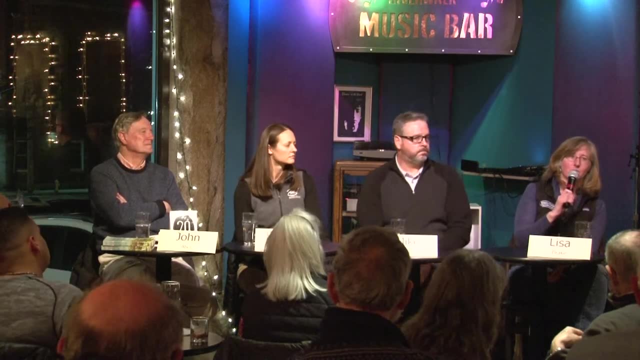 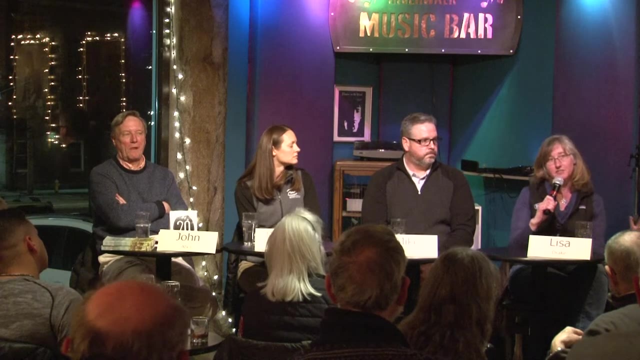 And one of the things I think we're learning about microplastics in the ocean is that one of the sources is our laundry, And what materials are we washing, and the fibers that are released every time you wash, So like polyesters, can be coming out of your washing machine. 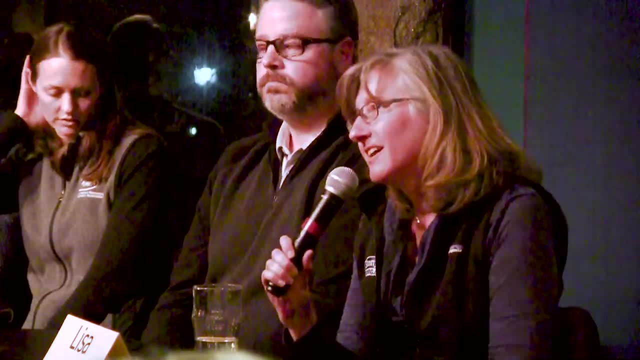 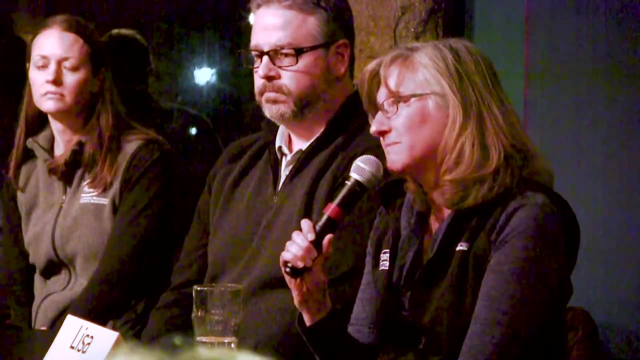 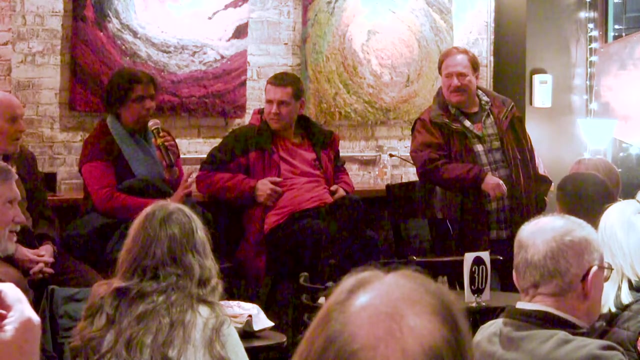 going out to Meramec River and out to the Atlantic Ocean. So you know, natural fibers over synthetic fibers may be part of that solution. In terms of plastics on packaged food, for example, I have What happens to it Like if I 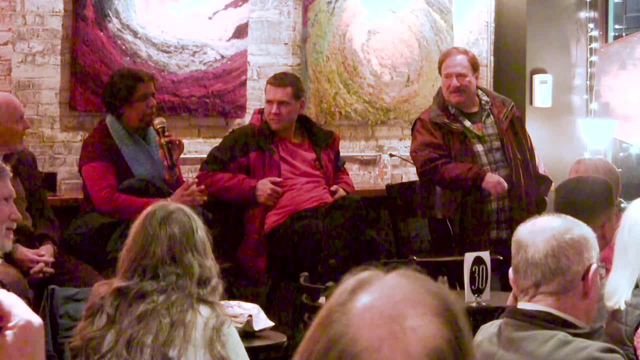 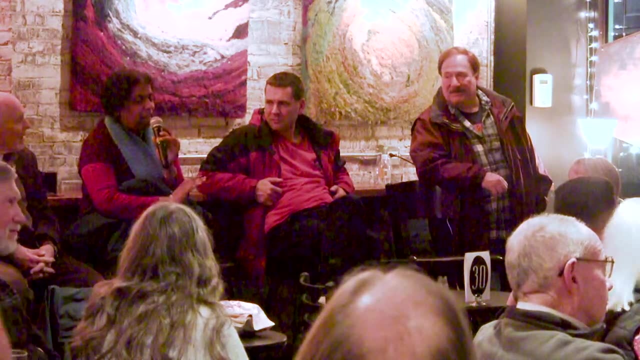 I put them in the grocery store- plastic recycling thing- but I don't know what happens to it. Does it go anywhere, or is it just going to the landfill? And do you have any ideas on how to get rid of that? Others, Most other things. 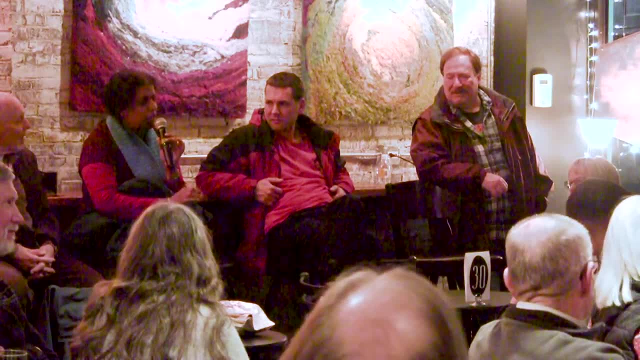 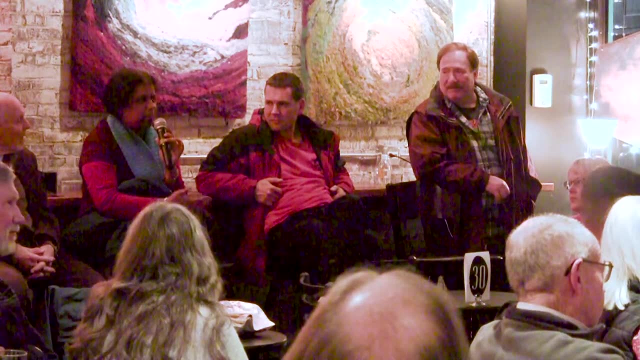 I think I've figured out some ways, But I minimize the packaged foods I buy. But still there is some plastic in packaged foods or things I buy. Like I bought a computer cable today, It comes in a plastic bag. So you're referring to plastic film. 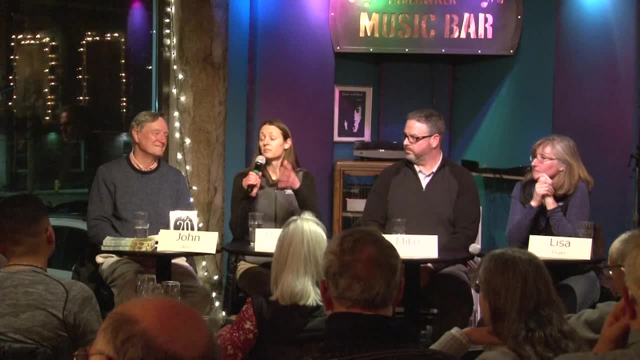 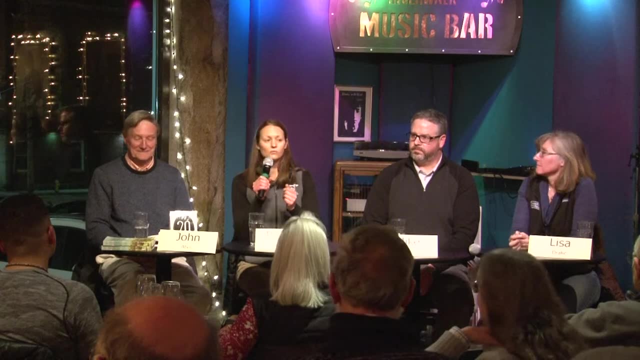 that you can take to the back to the grocery store like your, like a plastic bag, or Right? They seem to collect it if I give it to them, but I don't know what they do afterwards, Right? So plastic film. 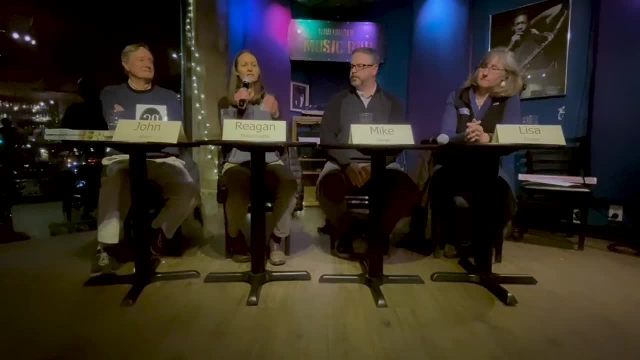 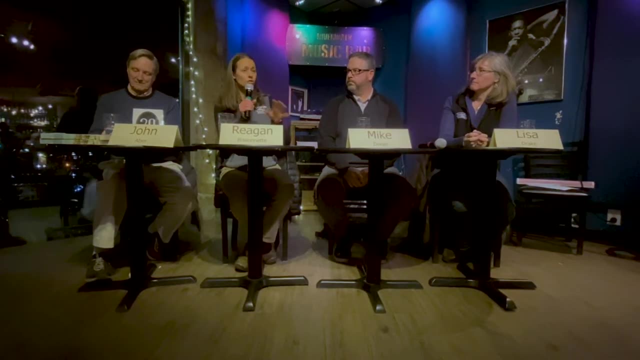 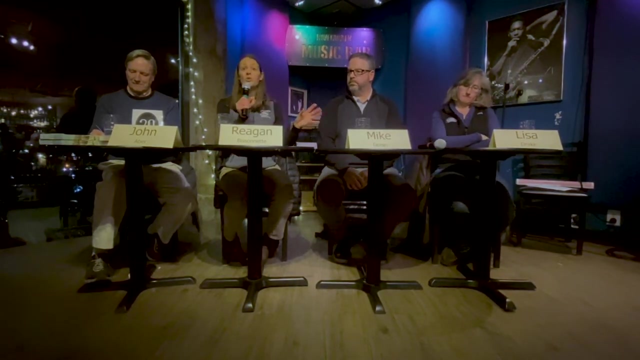 like your plastic grocery bags, the plastic bags that your bread comes in. those are recyclable. typically not through your local recycling facility because they- especially if they're sending the material to a materials recovery facility- they really don't want that gumming up the machinery. 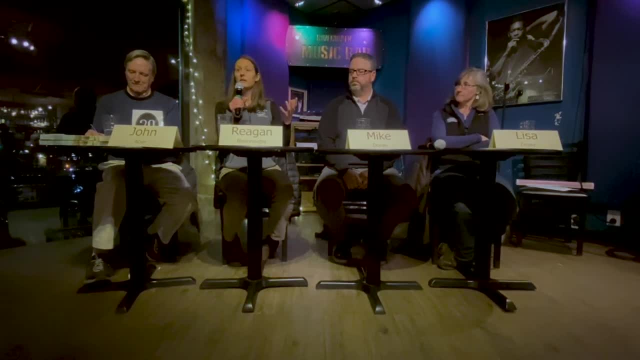 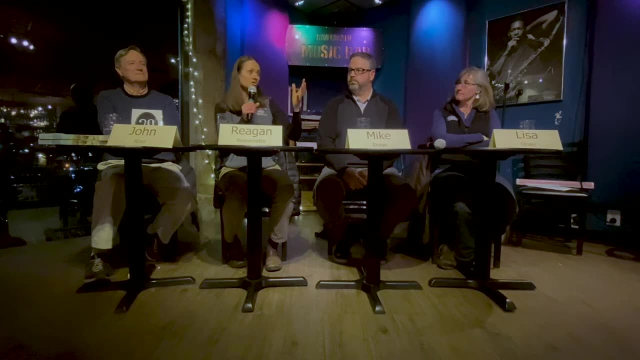 That's the number one contaminant is plastic bags basically, which is both time-consuming and dangerous for workers to go and cut bags out of the machinery. But you can take it to a lot of major retail stores like grocery stores and what actually they do. 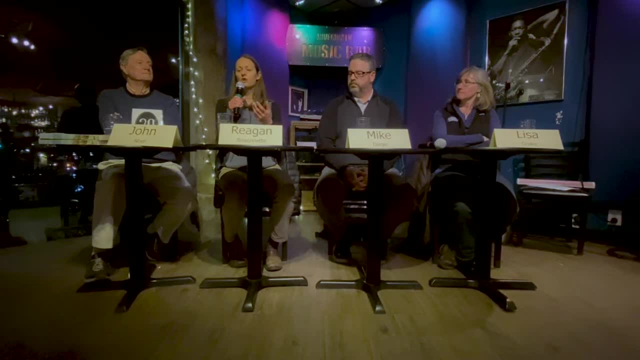 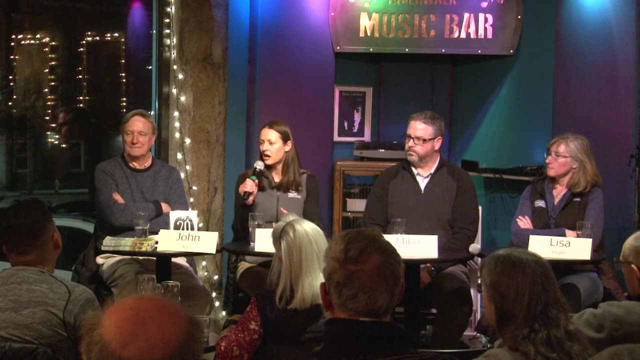 much of that material is used for Trex decking. Trex decking is a composite. It's made to sort of look like wood, but it's a wood and plastic composite decking that's very durable, So that plastic film is a major component. 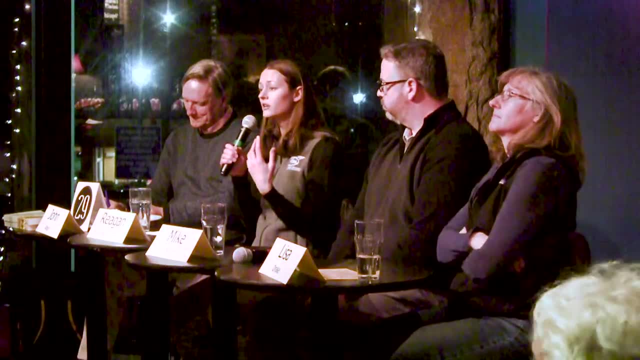 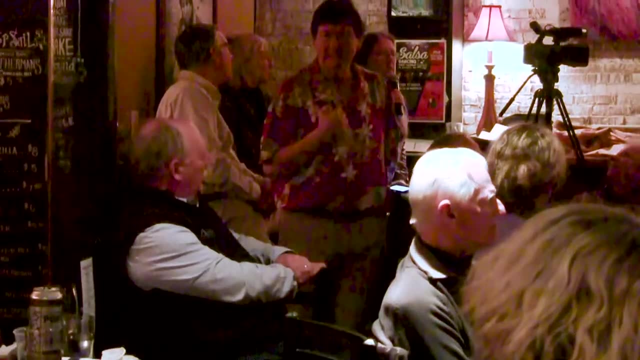 of Trex decking. I know that a number of the retail stores in New Hampshire are sending their material to be recycled through Trex. I know earlier you guys were talking about reduce, reuse, recycle, which we've been learning in schools for years and years and years. 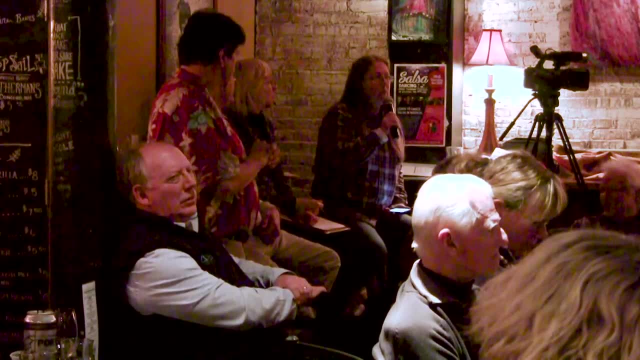 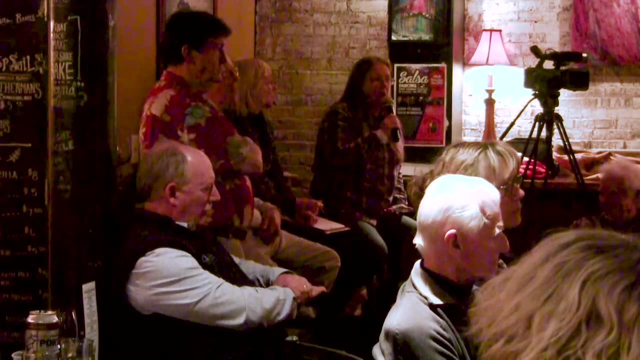 and I hope that the elementary and middle and high schools are starting to add the refuse, reduce, reuse, recycle and teach that as a hierarchy Those three are not equal or those four are not equal. You should refuse first, then reduce. 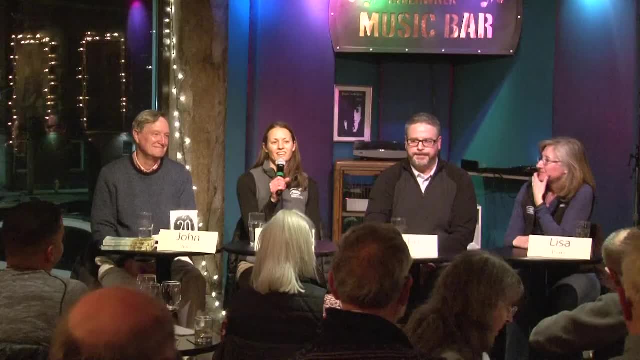 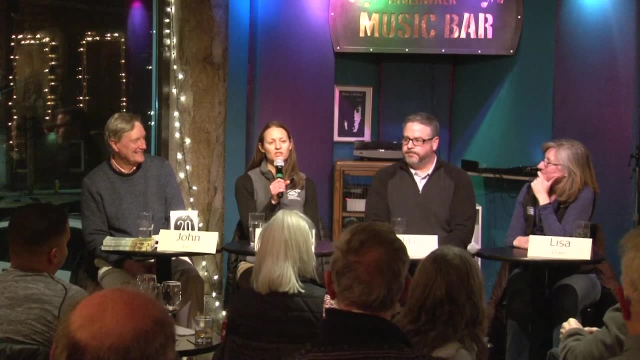 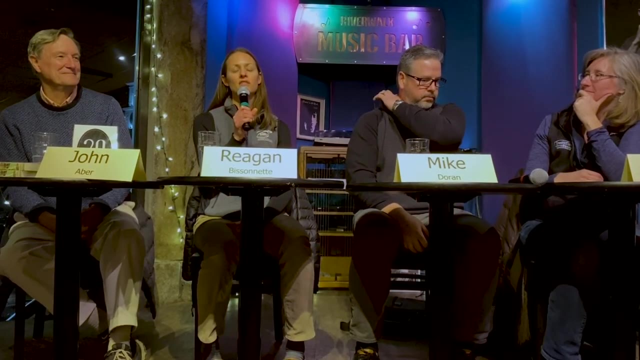 then reuse, then recycle And- can I add, rot to the end. So five Rs Actually, that's a nice segue. I'll just mention that we do a two-day annual conference each year and this year our keynote speaker is Bea Johnson. 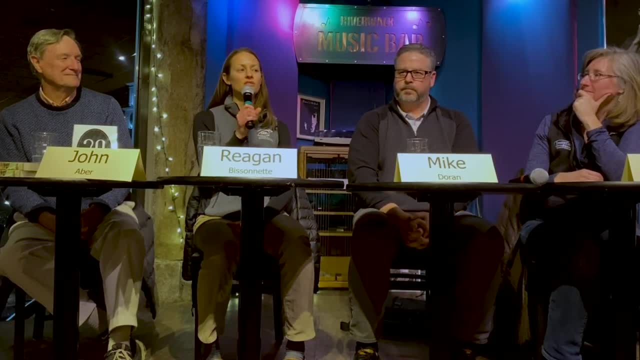 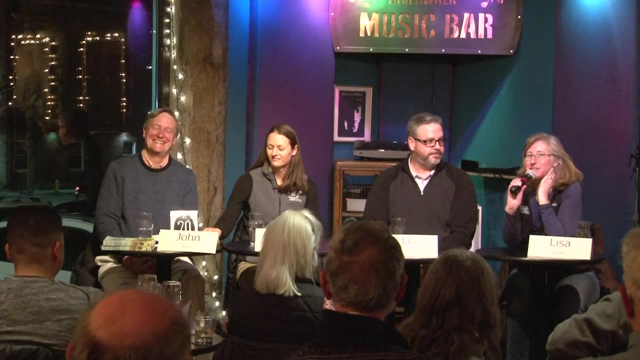 She is the leading spokesperson on the zero-waste lifestyle movement. She travels the world speaking about the five Rs, starting with refuse and ending with rot, And we should be teaching them. but you know, I'll tell you, this generation that's in school right now. 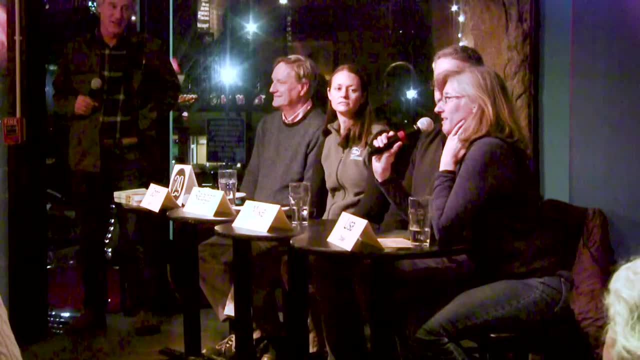 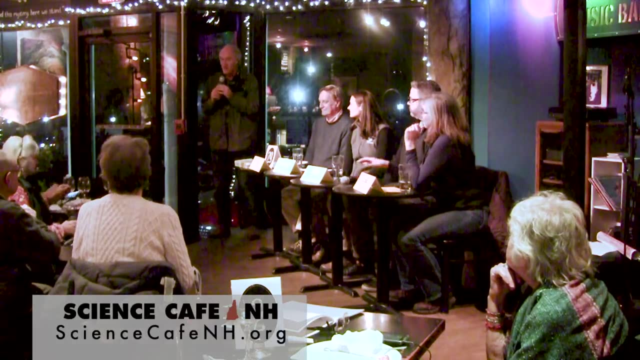 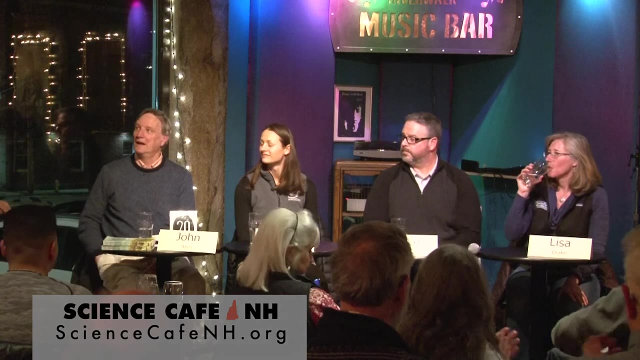 they're different and they already know it somehow, And they're changing their lifestyles in ways that, as older folks, are much harder for us to do perhaps. All right, Please join me in thanking this exceptional panel And thank you all for coming. 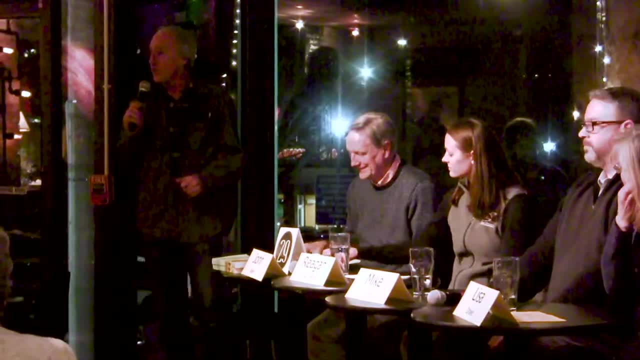 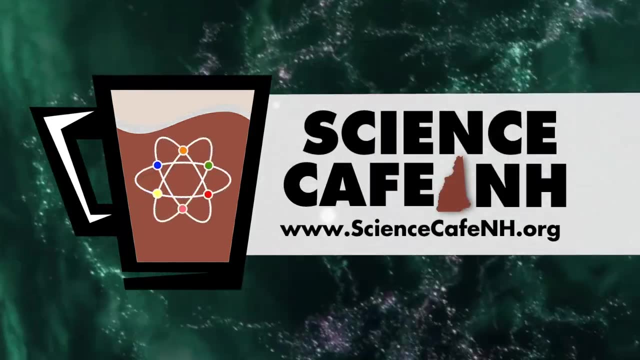 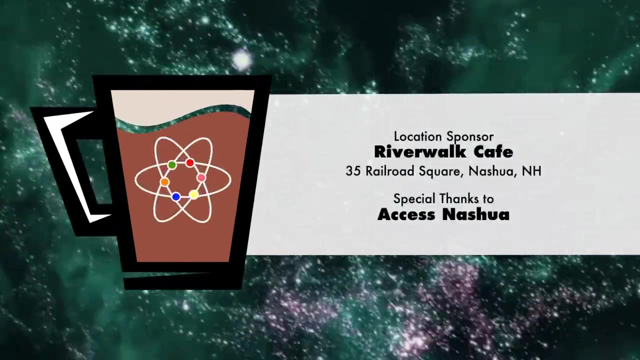 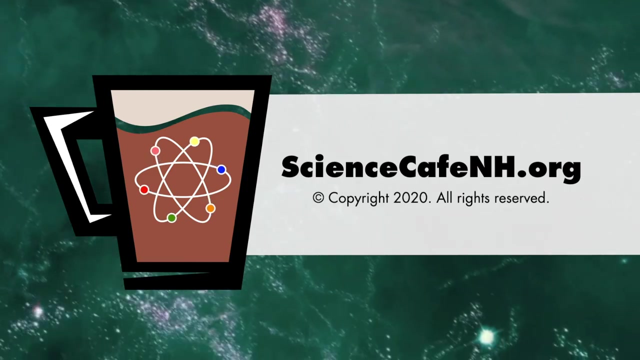 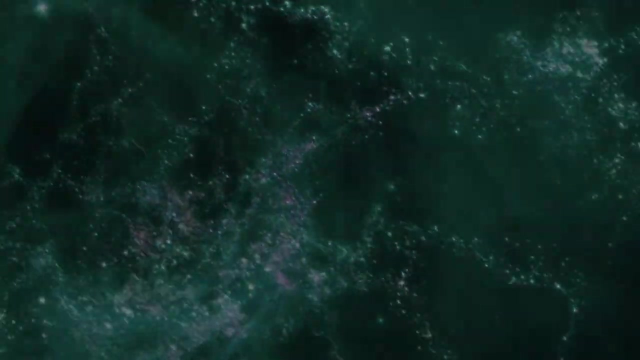 Next month we'll be talking about the science of science fiction, so put it on your calendar. See you then.